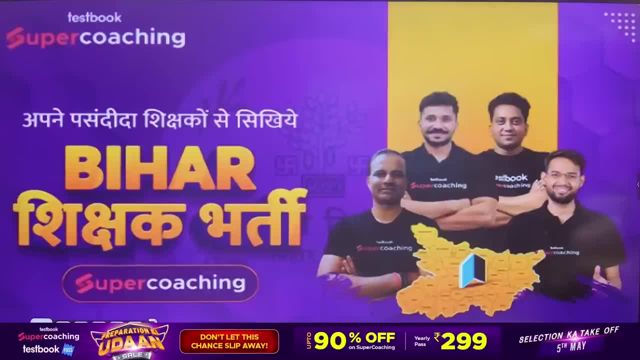 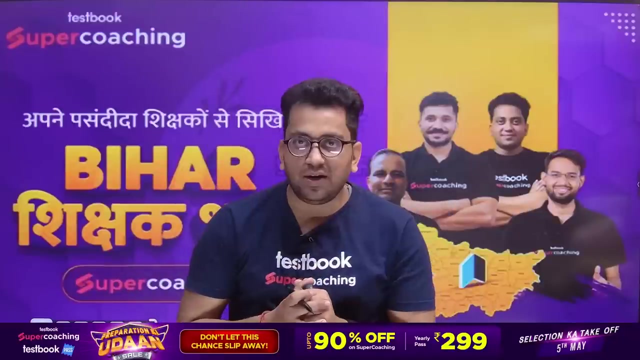 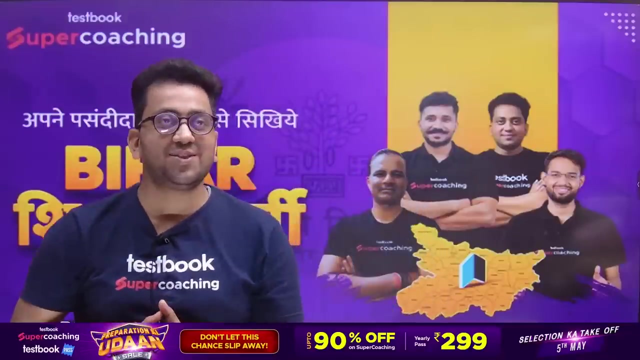 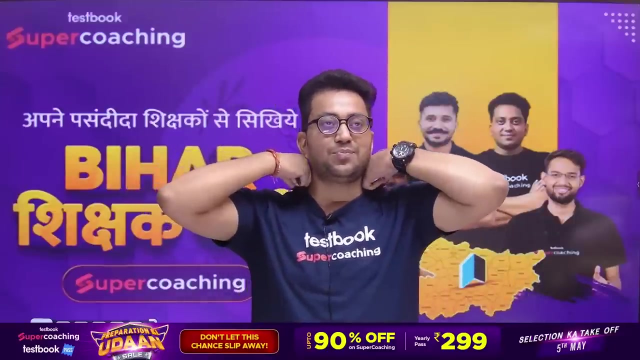 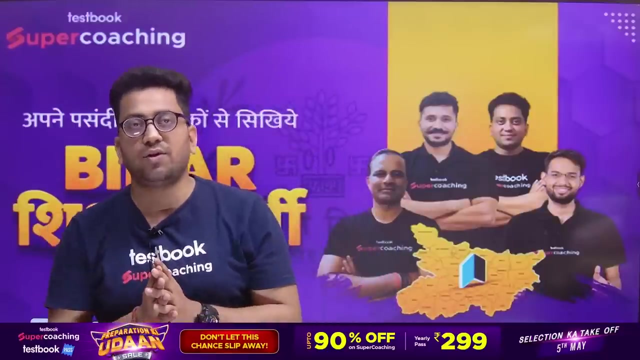 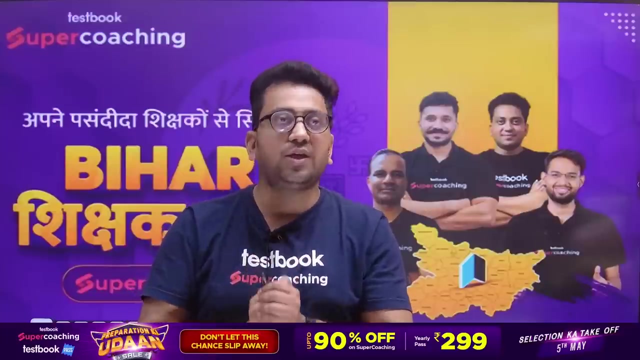 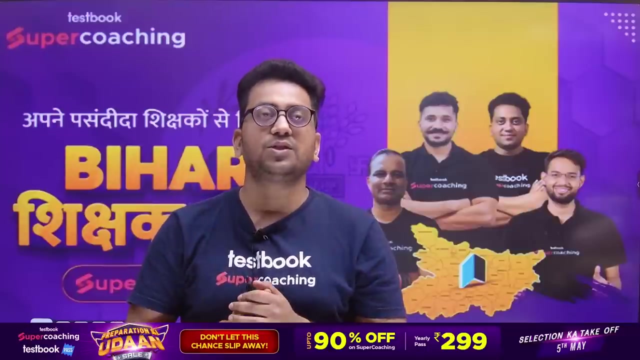 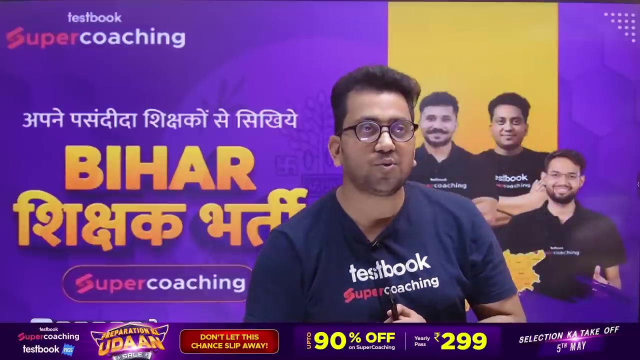 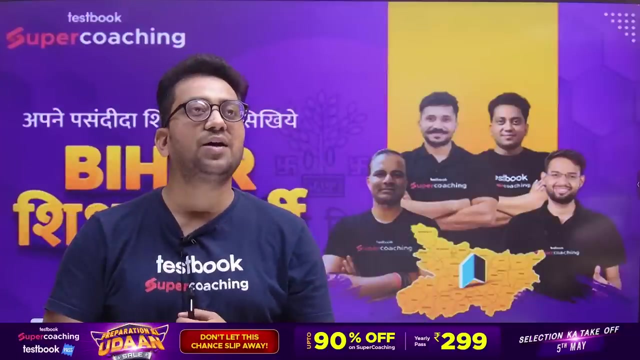 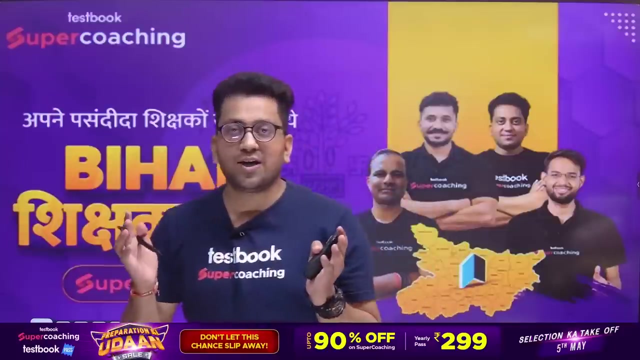 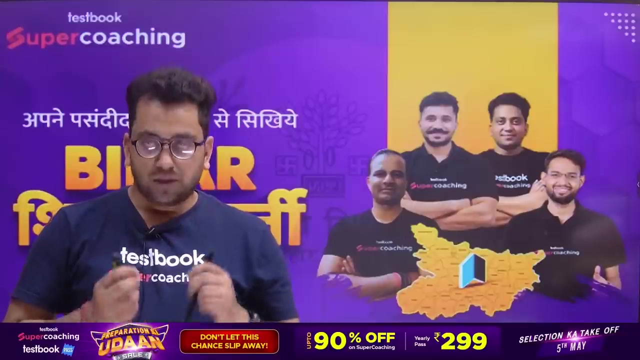 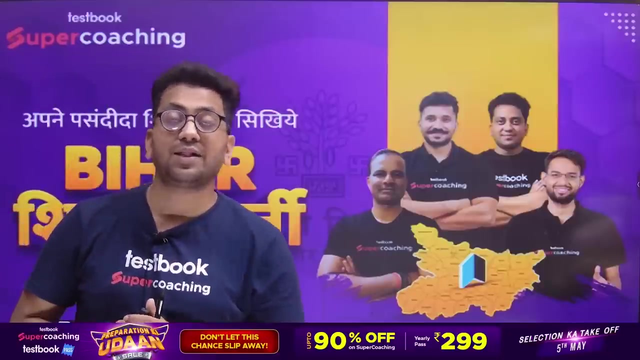 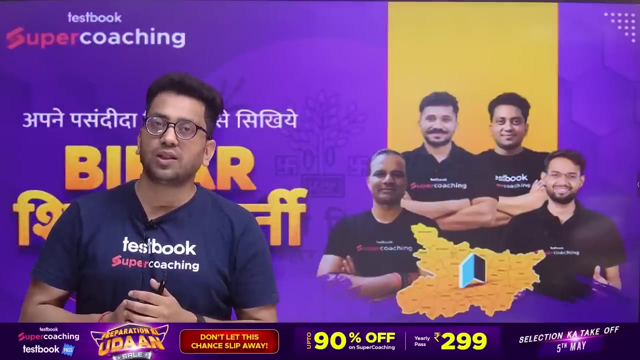 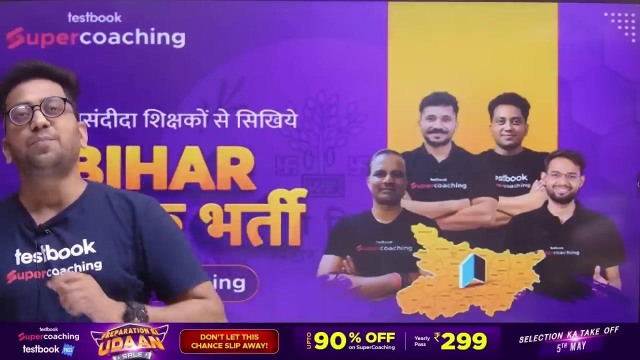 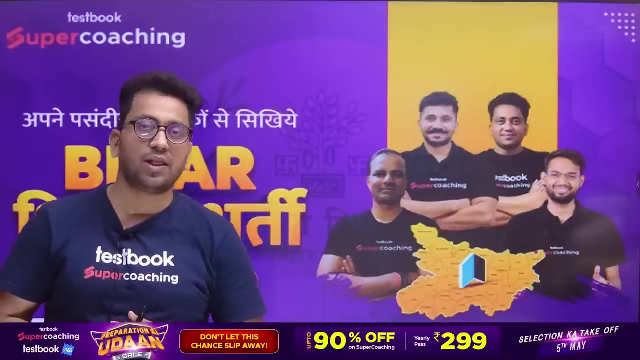 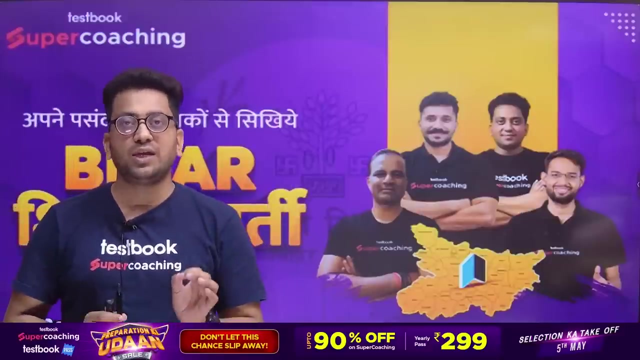 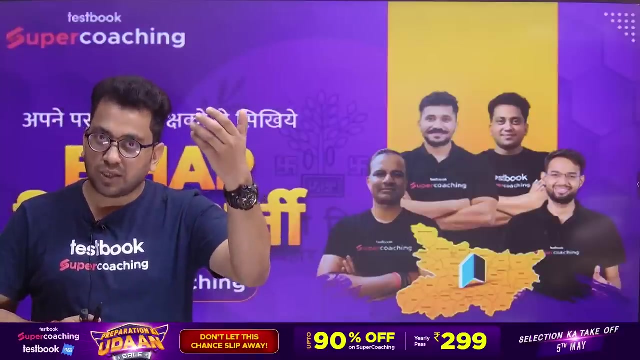 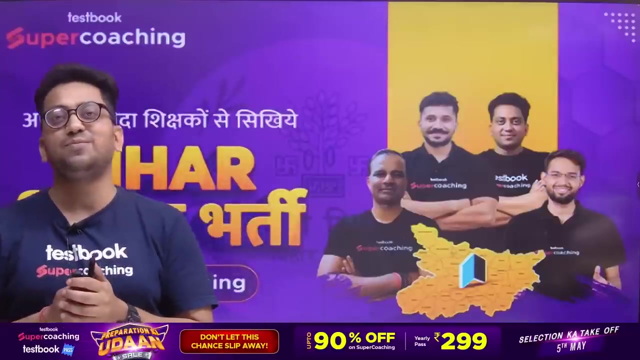 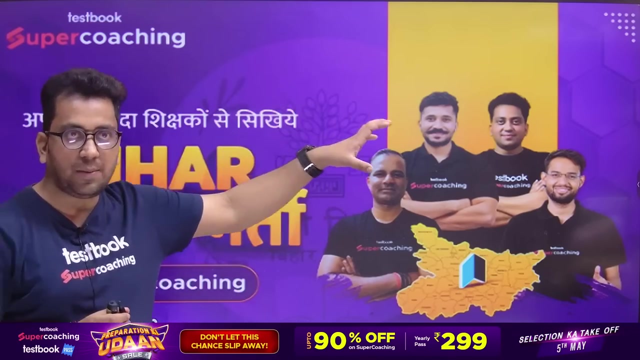 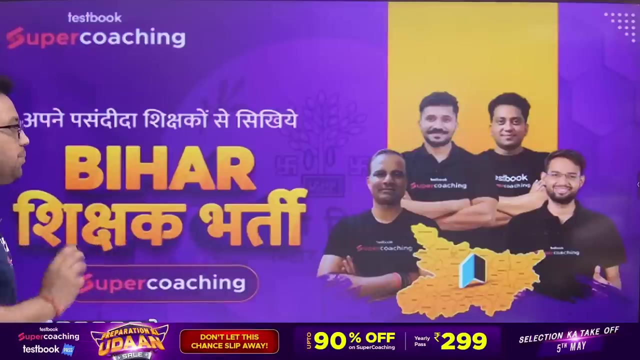 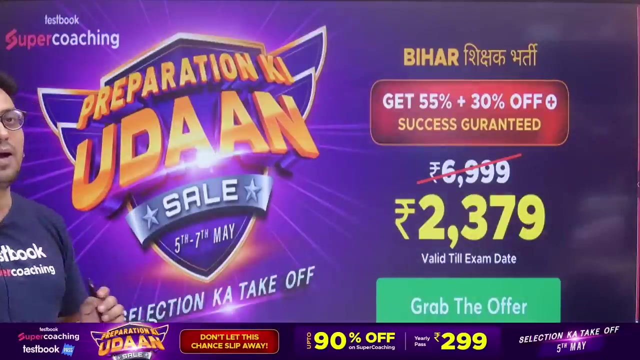 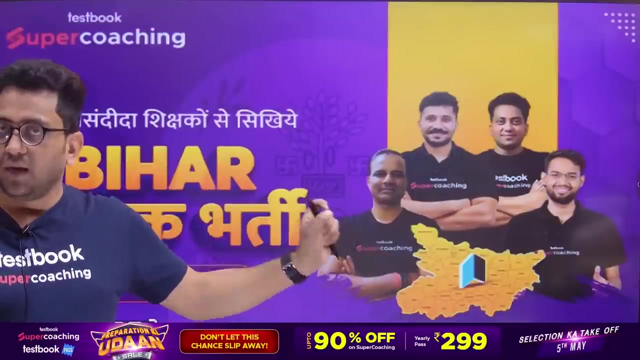 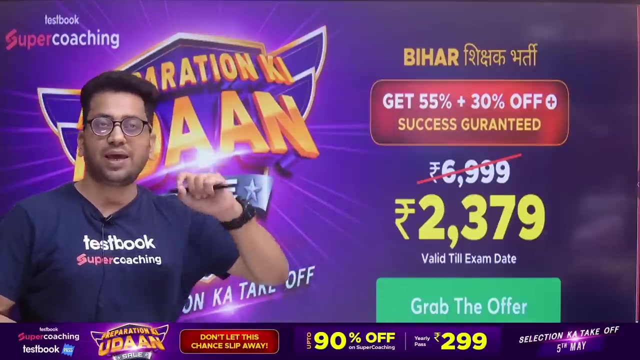 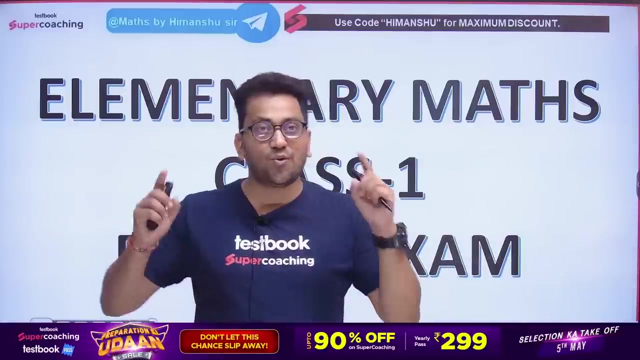 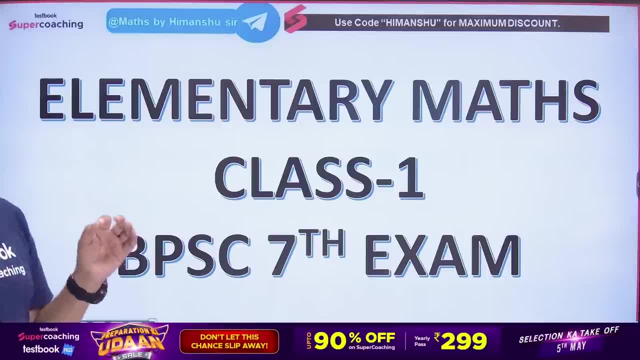 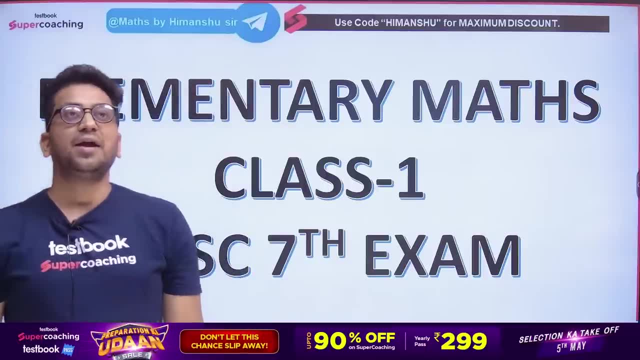 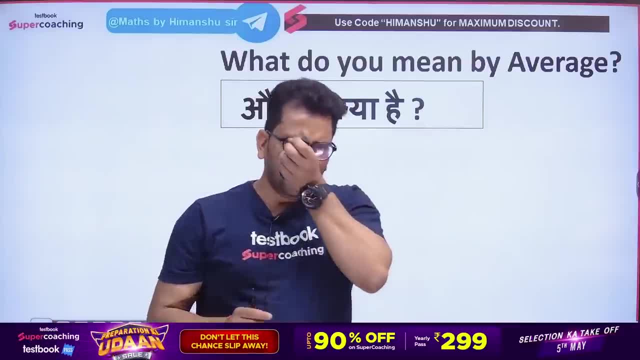 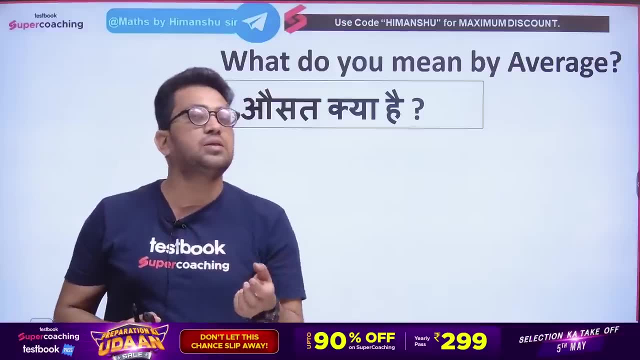 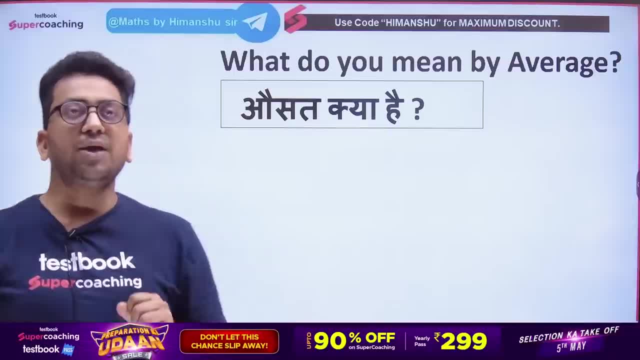 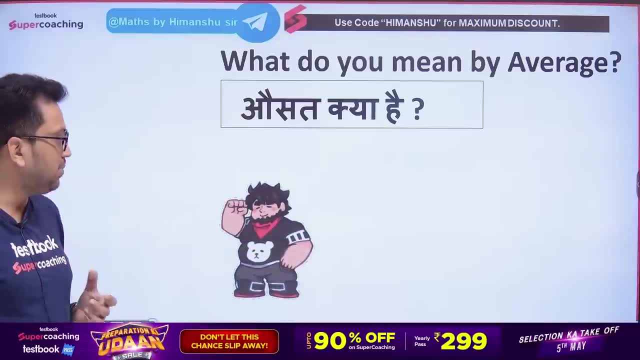 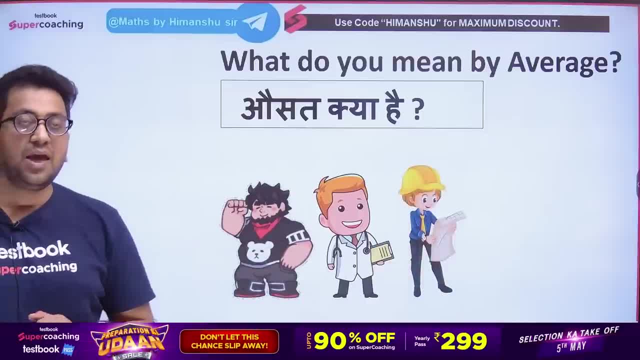 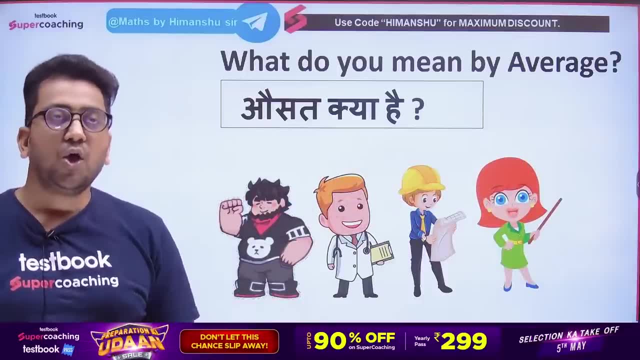 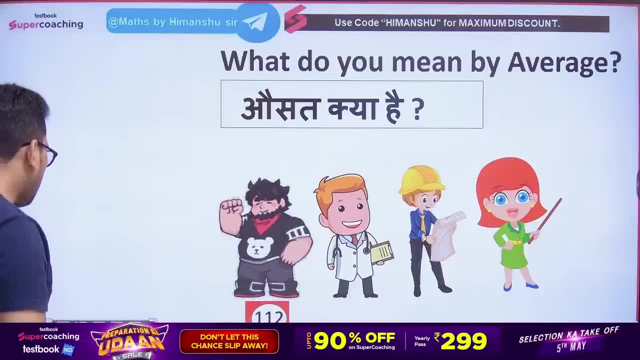 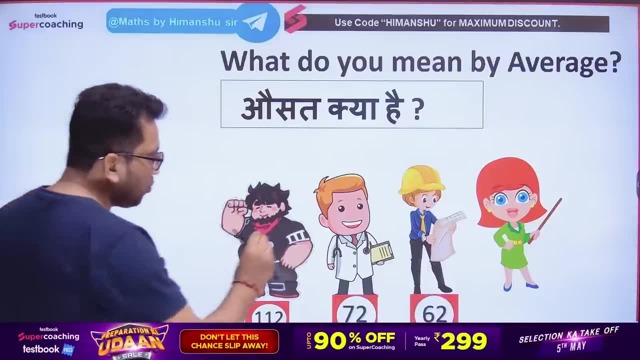 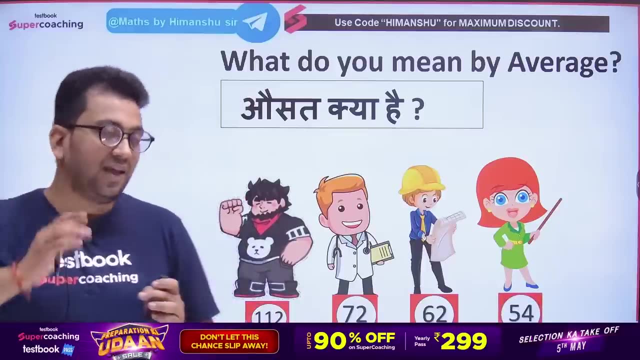 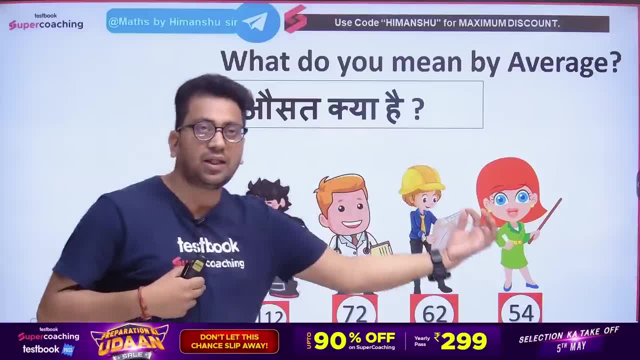 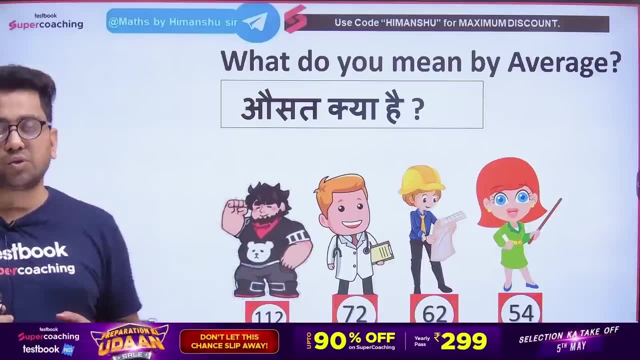 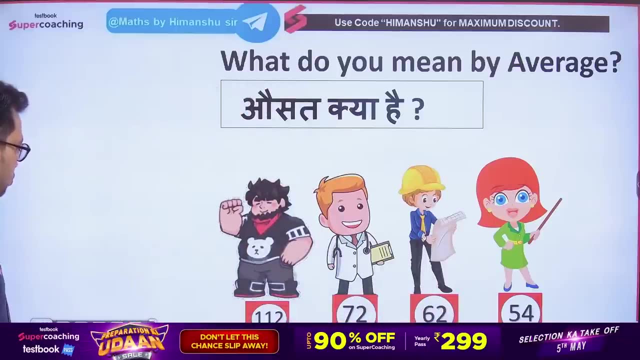 Now our point is that we want to find out the average weight of all of them. that is, the average weight. How to find out the average weight? It is a very simple question. What will you all do? We will add them all. What will we do, son? We will add them all. that is, we will do 112,, 72 in the total, 62 in the total and 54 in the total. 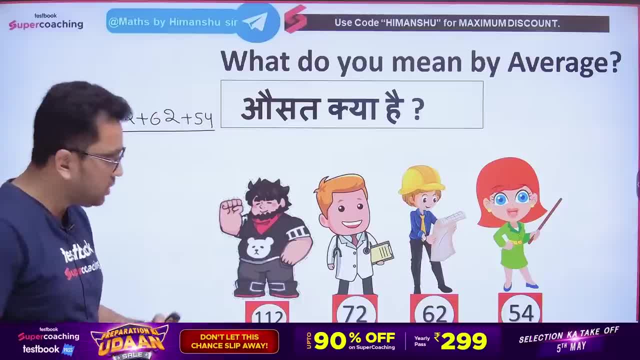 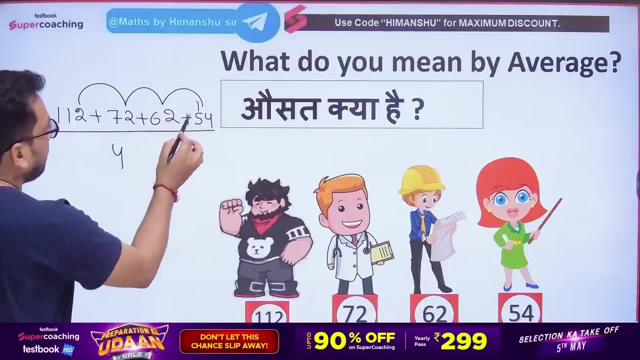 We added all of them and all the numbers, that is, all the people. we will separate them. If there were 4,, then we will separate them from 4.. 2, 2, 4, 2, 6, 4, 10,. we got 1, 5, 6, 1, 5, 1,. 6 is done. 6 is done. 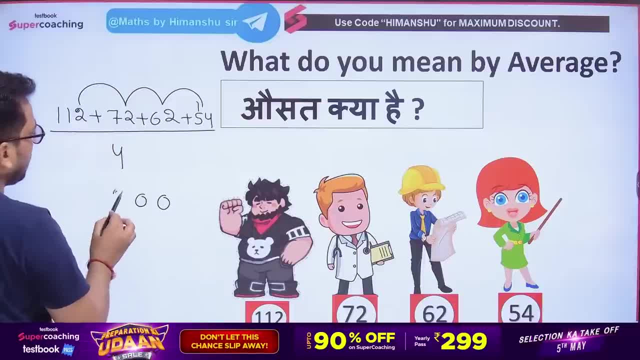 6,, 12,, 7,, 19,, 19 and 1, 20 is done. we got 2,, that is 300, and if we separate 300 from 4, then here comes 75 kg. This 75 kg which came? this average weight came out. the average weight came out. 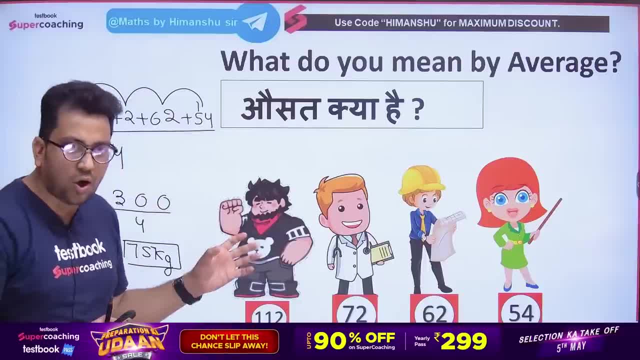 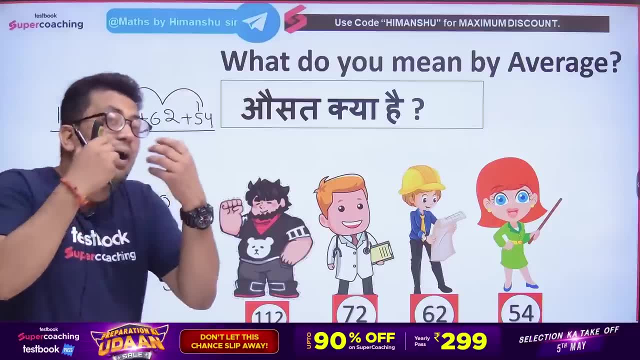 That is, if I tell you that the average weight of all four of them is 75 kg, to understand the thing, to understand the feeling, then the feeling is that I want to say that you accept my saying that the weight of all of them is 75 kg. 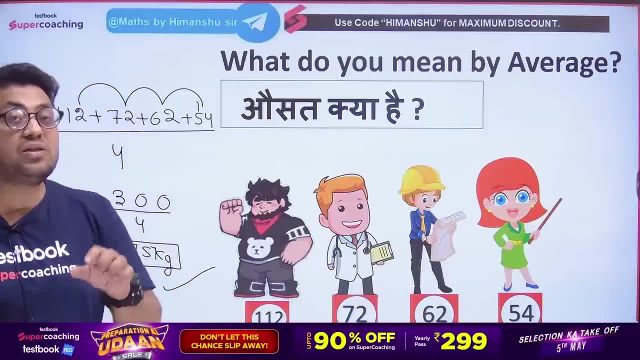 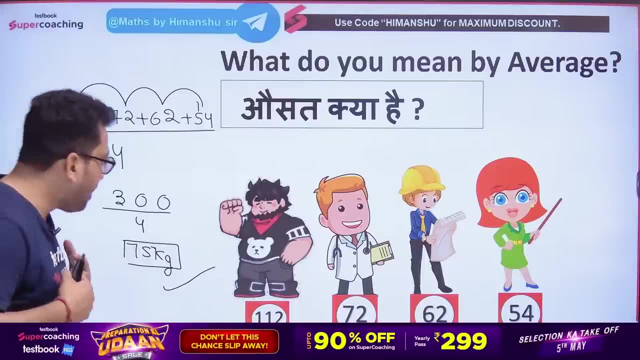 Although, in reality, someone may be 75,, someone may be less than 75,, someone may be more than 75,, but I will assume that if the average weight is 75 kg, then the weight of all of them is 75,, 75,, 75.. 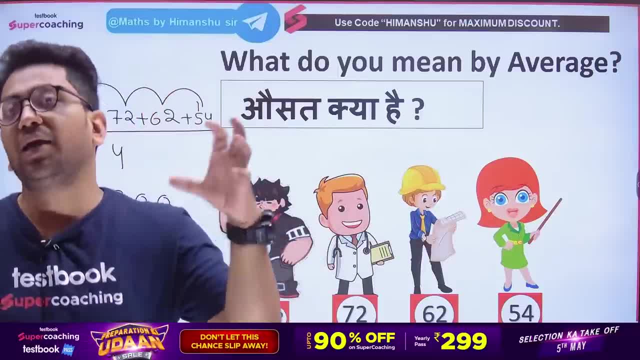 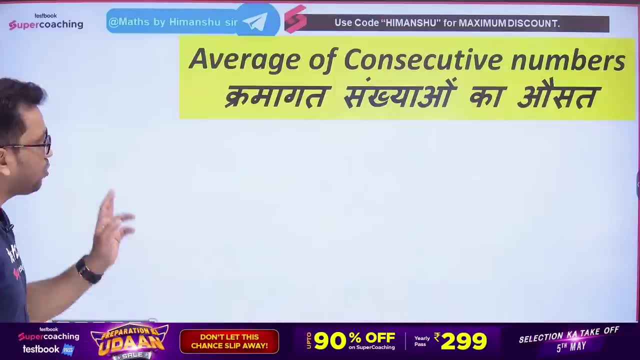 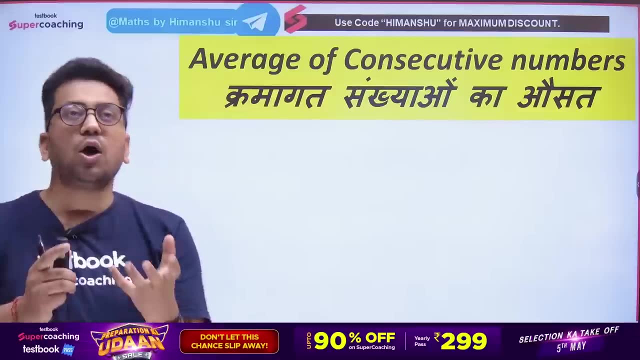 This is the meaning of the average per head that everyone has how much understood. Now, based on this, we are going to see some things. we are going to see some concepts. what are those concepts? First of all, the concept of the average number. how do we find out the average number, sir? 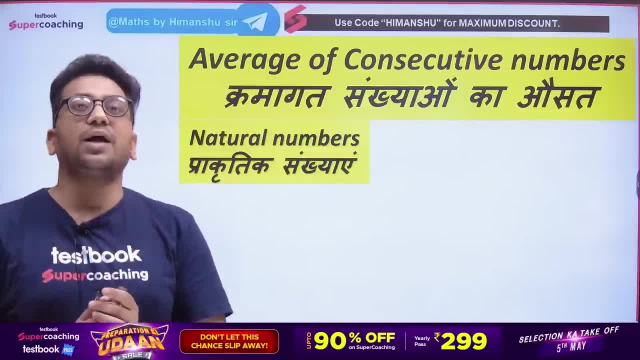 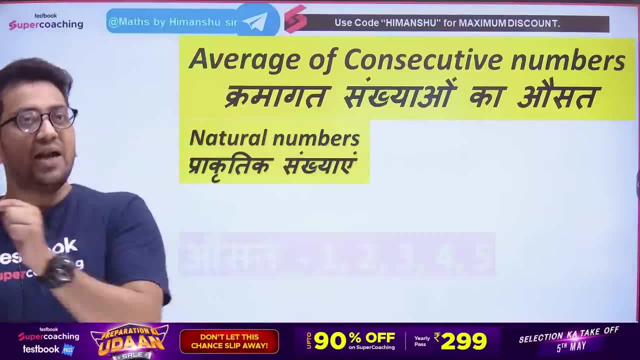 The numbers that are going on continuously. what are the numbers, sir? First of all, we will talk about the natural numbers in these average numbers, that is, the natural numbers. Now, where do the natural numbers start? Every child knows, sir, they start with 1,, 1,, 2,, 3 and keep increasing. 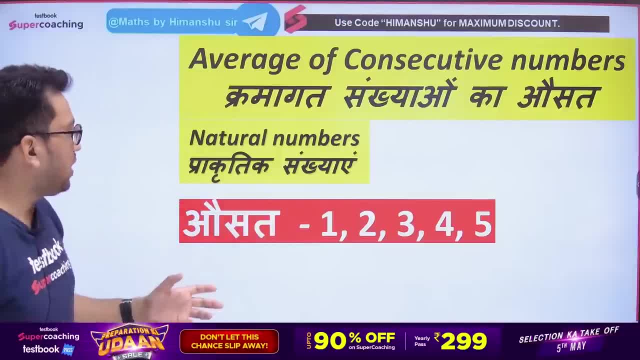 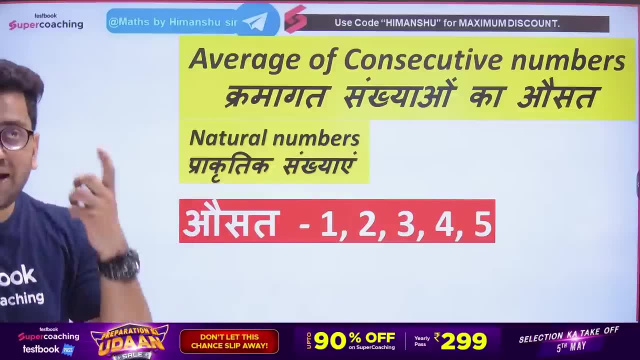 So now I just want to know from you that tell me this that 1,, 2,, 3,, 4,, 5.. What will be their average? What will be their average? You tell me this, So our child will answer in the comment section quickly that what will be the average of 1,, 2,, 3,, 4, 5.. 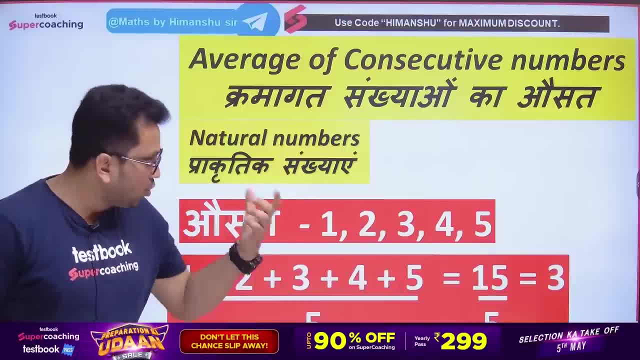 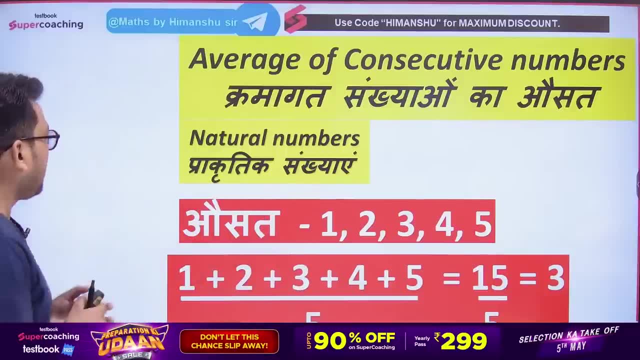 So every child can answer. What will he say? Sir, add them, Add them and divide them by 5.. What I have done below is divided by 5.. Do you understand what I mean? That is, you have added everyone and divided them by 5.. 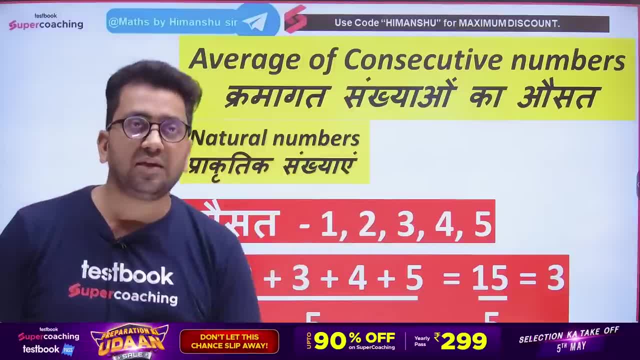 So 3,, 3,, 6,, 4,, 10,, 5,, 15,, 15 divided by 5,, the answer will come 3.. How much will the answer come? Our answer will come 3.. Are you able to understand what I am saying? 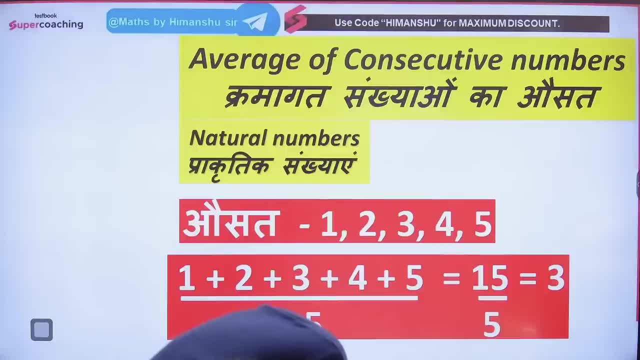 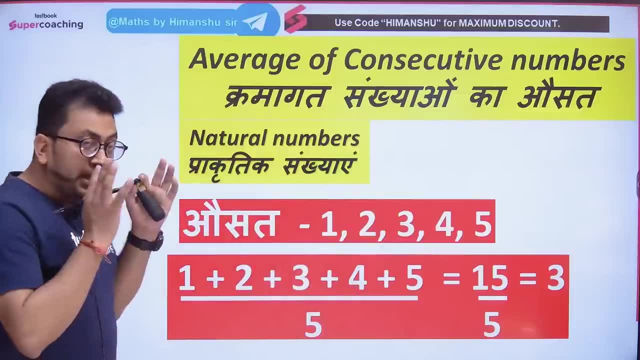 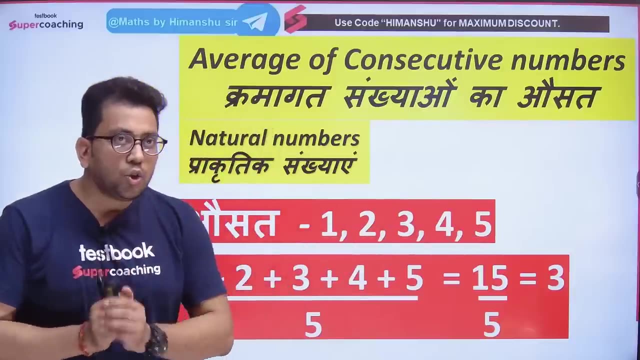 Is it clear here. Are you able to understand? Okay, Yes, So 3 will come. That is, you just look at it carefully. that where was 3?, Sir, when these round numbers were going on? then the middle number that you can see: yes, child, you can see this 3.. 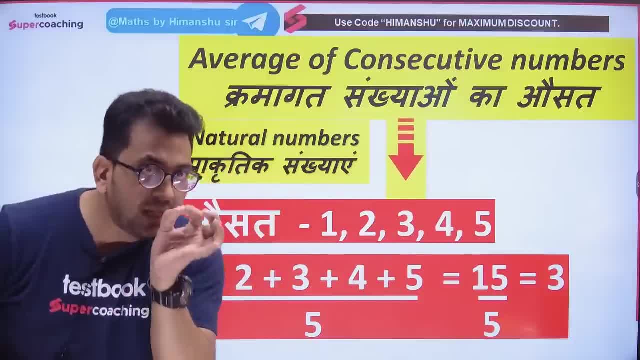 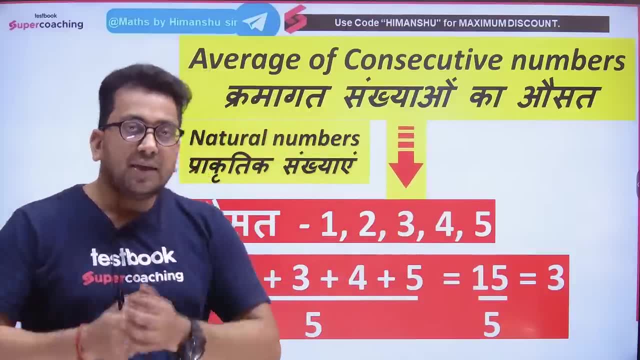 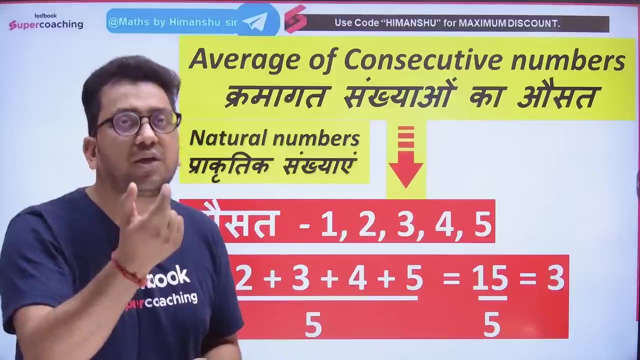 Can you see this? You can see this. 3, right, This is the middle number. This is the middle number. This is your average. Yes, That is. if the numbers are going on continuously, there are round numbers- then the middle number will be called its average. 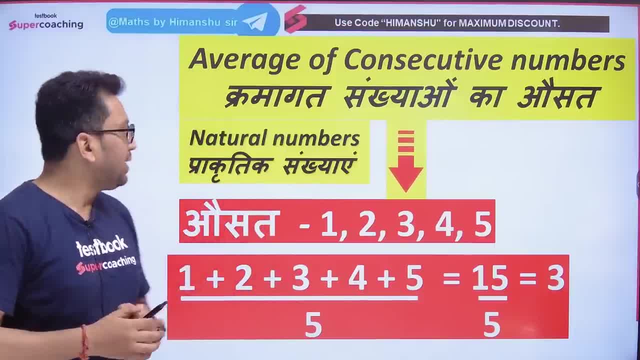 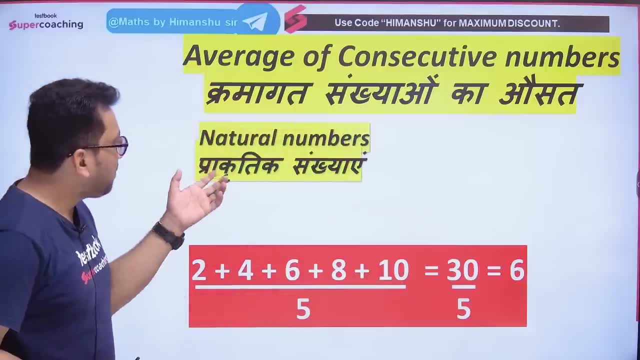 This concept has shone from here, sir. Sir, do only natural numbers come in round numbers? No, No Here in natural numbers 2, 4,, 6,, 8, 10.. This also comes because these are natural numbers. 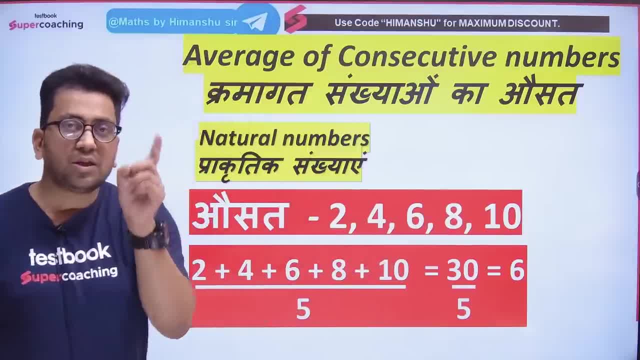 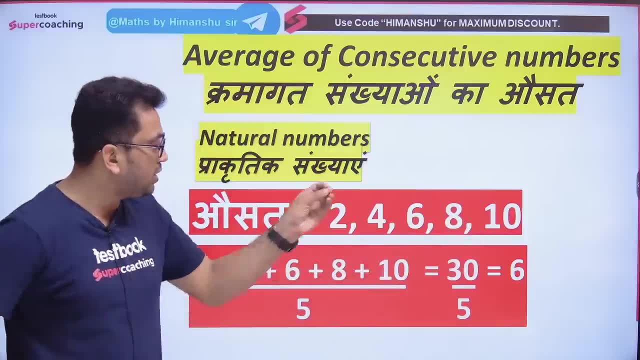 What are natural, Natural numbers And natural numbers? even in natural numbers, there is a difference of 2, 2.. You all know 2, 4,, 6,, 8, 10.. These are Now, let's say, I want their medicine. 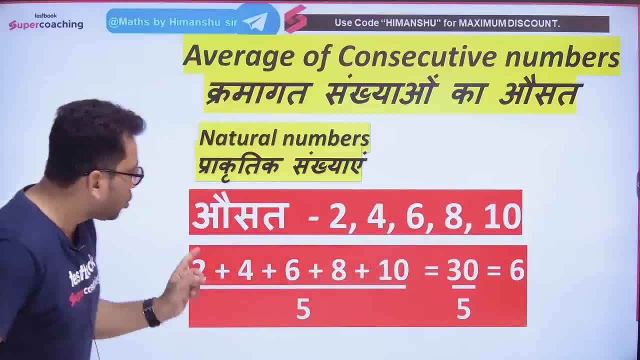 Now, if I want their medicine, then what will I do? I will add them all child, So 2,, 4,, 6, 6,, 12,, 8,, 20,, 10,, 30. I will run from 30 to 5.. 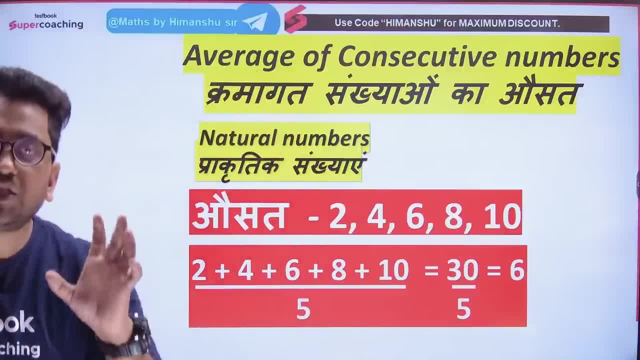 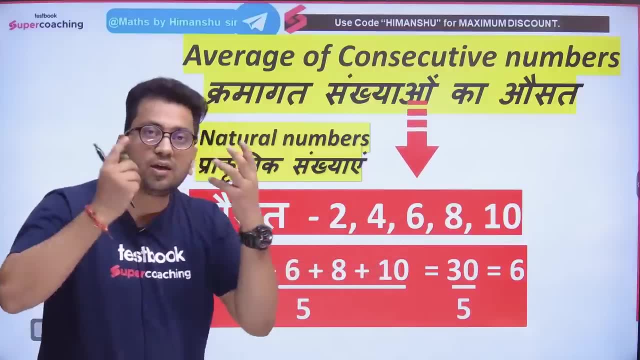 How much medicine will you get? You will get 6.. How much will you get? You will get 6.. And, sir, just look carefully. Look carefully and think that the middle number here is 6.. This is the medicine. That means, sir, the concept is slowly shining. 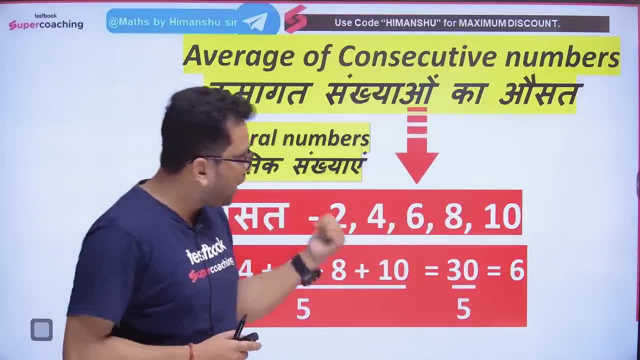 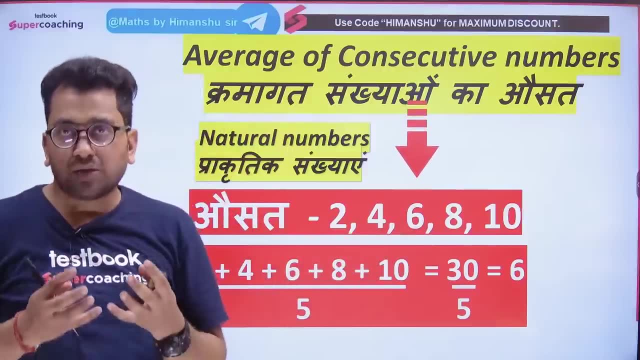 The concept is shining that, sir. in the previous one, 1,, 2,, 3,, 4,, 5 were running continuously. Here, 2,, 4,, 6,, 8 are running like this. That means if any system is in front of you where there is a difference. 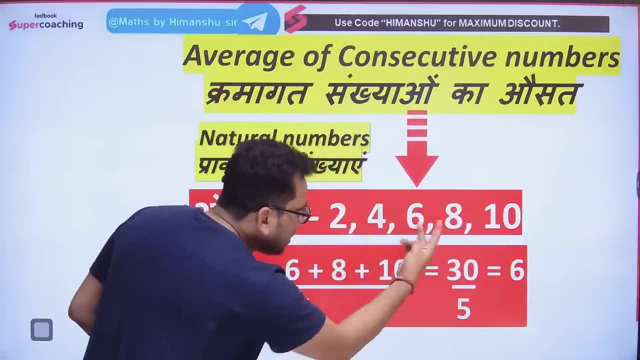 Can you see? There was a difference of 1,, there was a difference of 2, there was a difference of 2,. there was a difference of 3,. there was a difference of 4, there was a difference of 4,. no matter how much difference I take, 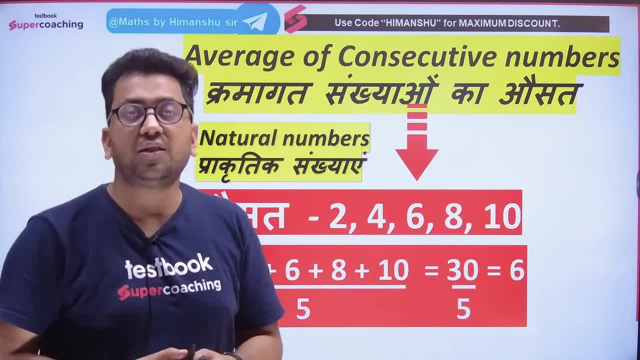 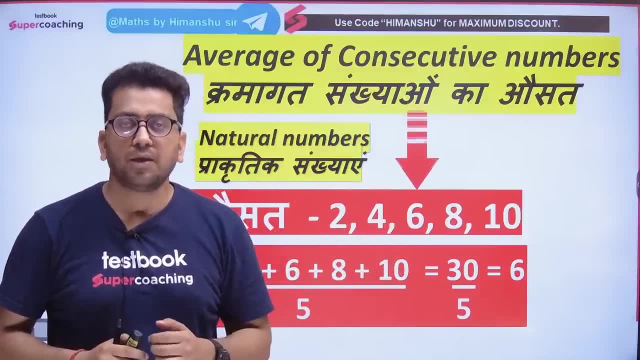 If there is a difference in a system, then the middle number, the middle number will be the same average. That means it is the same quantity. Sir, do all these natural numbers come in the numbers? No, There are also extra natural numbers, brother. 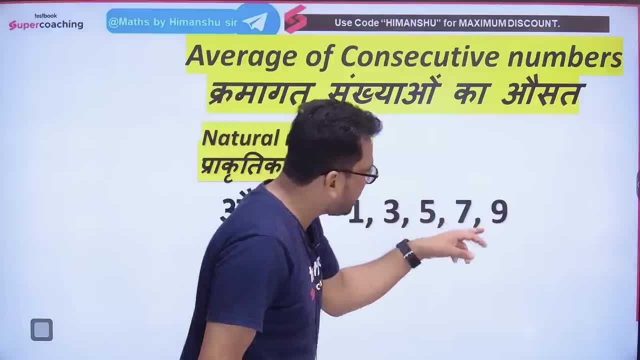 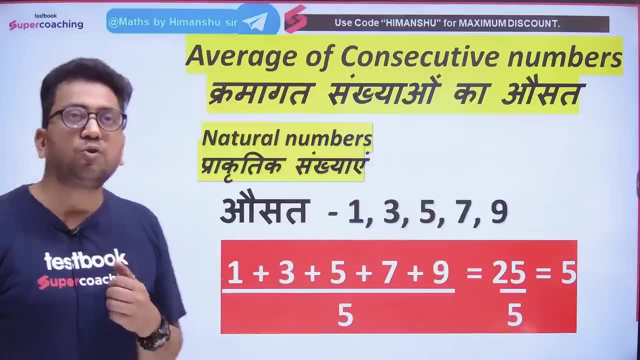 It can also happen that 1,, 3,, 5,, 7,, 9 are running like this. It can happen, sir. How will their quantity come out, Sir? then we will add everyone. We will add everyone, sir. 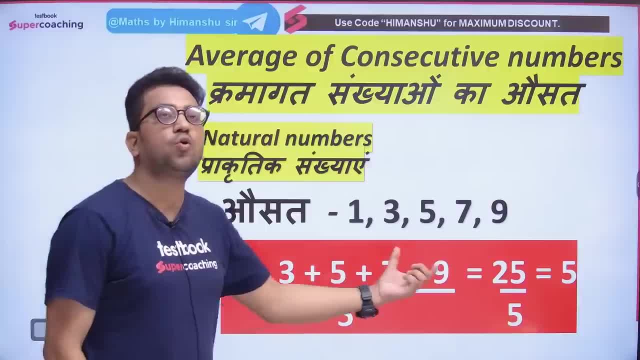 We will run from 5.. That means 1,, 3,, 4,, 5,, 9,, 9,, 18.. And 7,, 25, 25 will run from 5.. The answer will come to us: 5.. 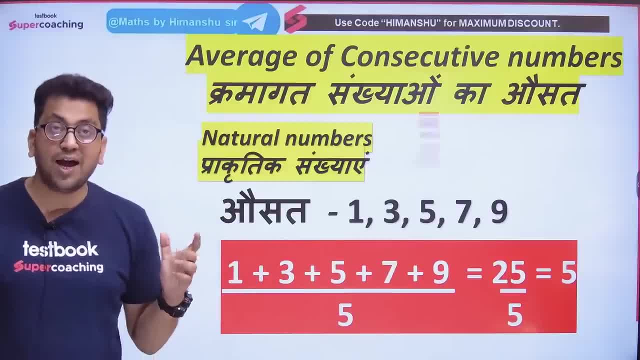 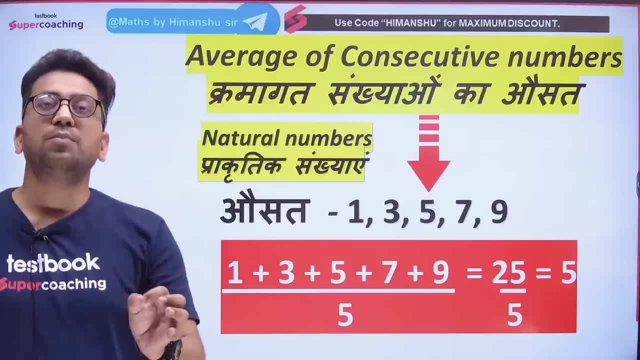 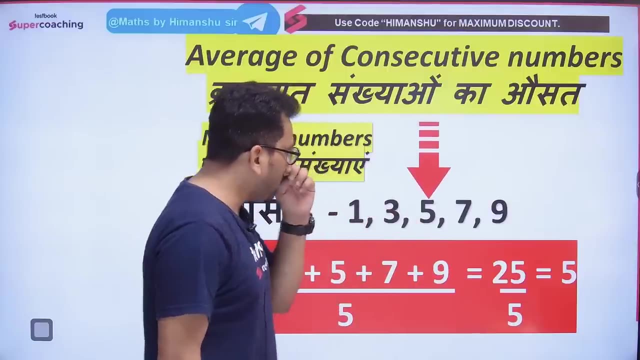 That means, sir, if we pay attention here as well, then the middle number that came out, middle number 5, this is our average. So the concept is now clear like a mirror and has shined. What If there is a system where the difference will be the same? see here also, sir, the difference of 2, 2,, 2, 2.. 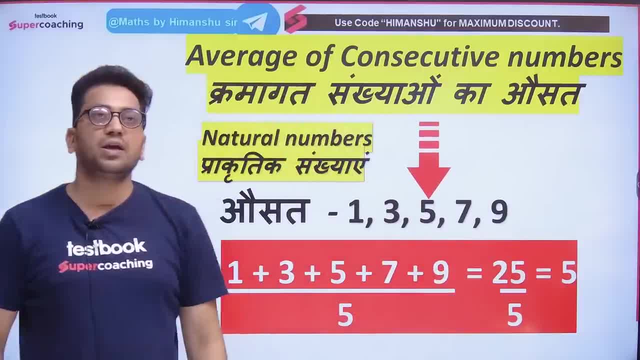 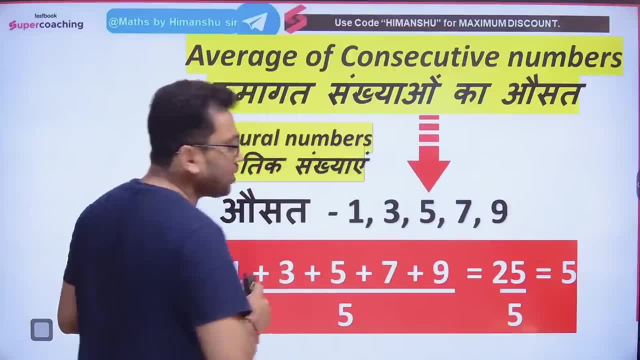 So the number of the middle is 5, that is our average. Now I will ask you a question. Now, see BPST son. how will the question based on this print you? in a way? This was the first question of today's session. 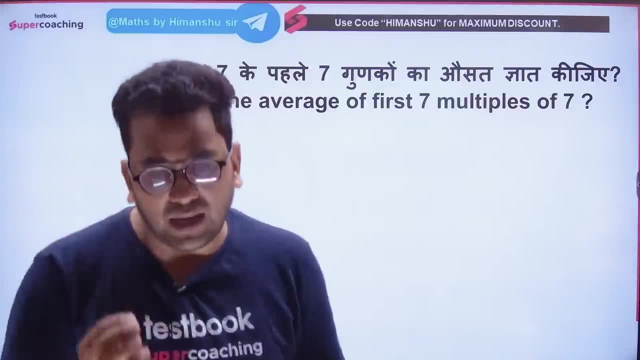 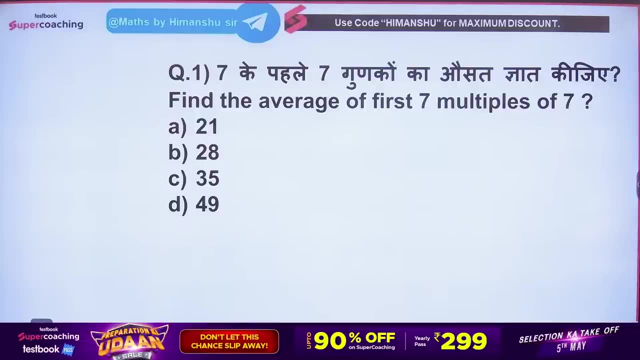 You have to learn the average of the first 7 qualities. Answer all of them quickly. Come on with speed. Right children answer. What are you saying, son? You have to tell the average of the first 7 qualities. You have to tell the average of the first 7.. 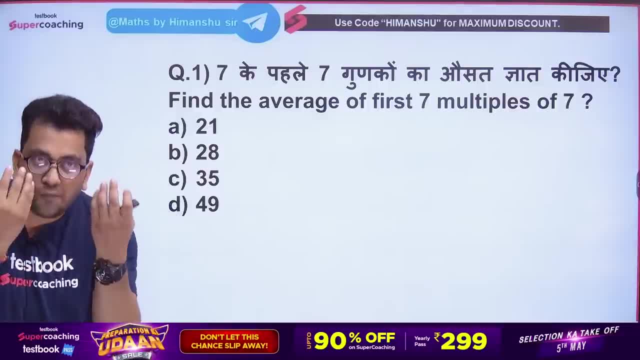 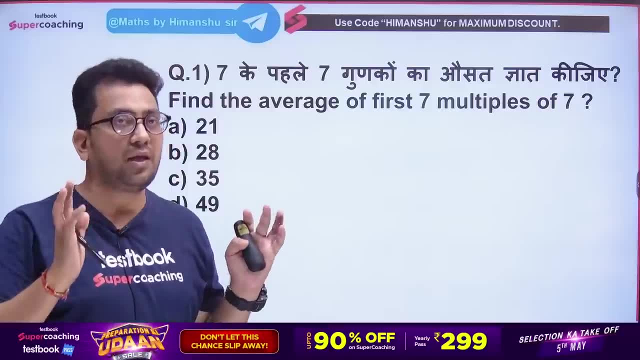 Find the average of first 7 multiples of 7.. So you know, your Himanshu sir explains to you and then also tells you the way to shine. So now come to this question. Let's take a look at this question, son. 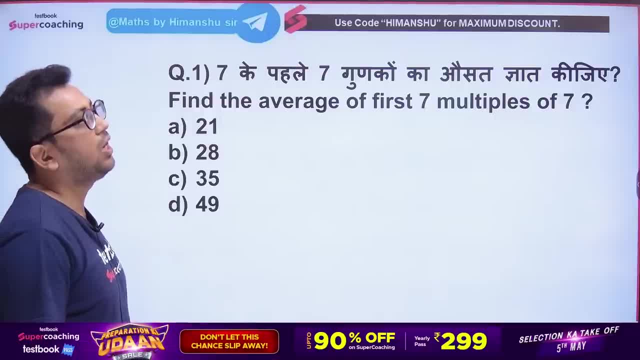 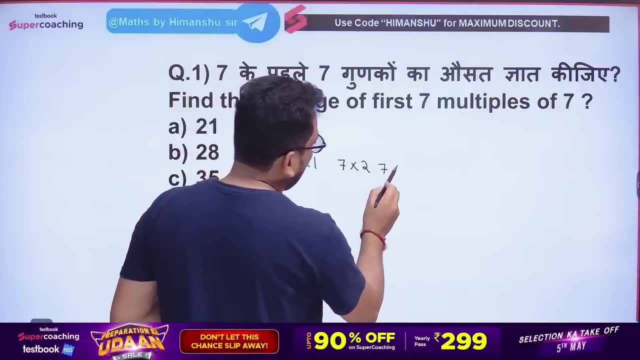 See what he is saying: The first 7 qualities of 7.. Okay, The first 7 qualities of 7 means they will be like this: 7 minus 7.. 7 times 14.. Isn't it 7 times 21.. 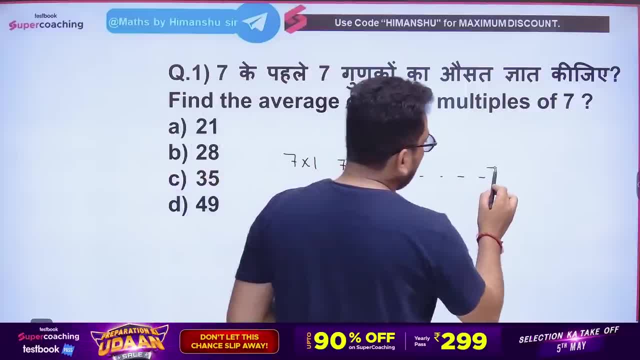 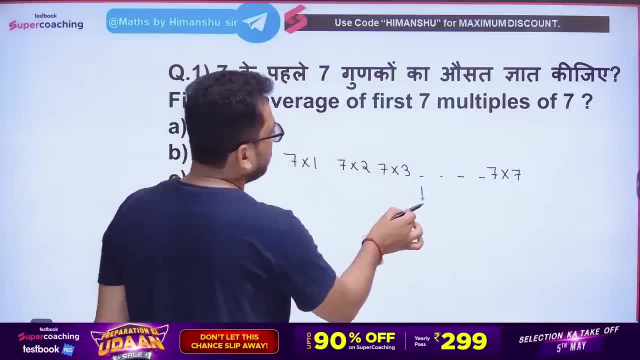 They will be like this, And the 7 qualities are being said that the last one will be 7 times 49. Say yes, isn't it? It will be like this, isn't it? Now he is asking us to tell the average of this. 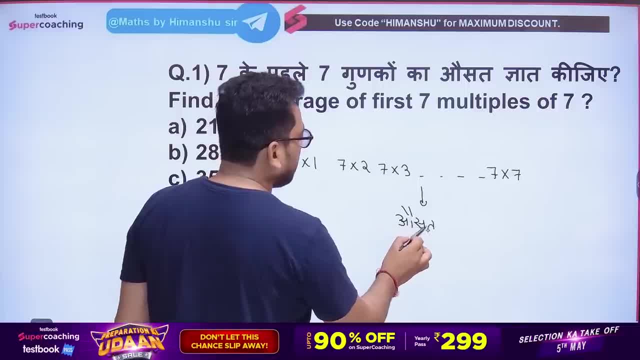 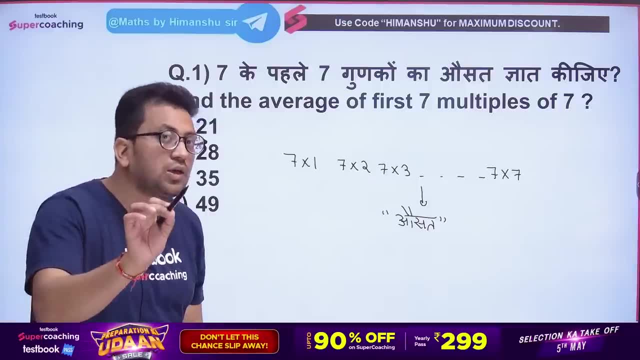 What will happen? Oh sir, just now we understood the concept: Such a system where there is an integral between the columns. The middle number there is the average. Is it so? If it is so, sir, then is there an integral here? 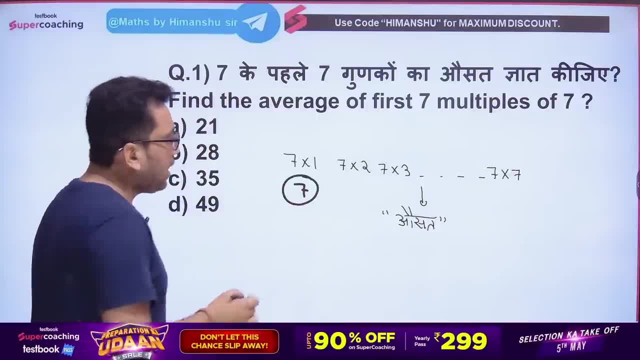 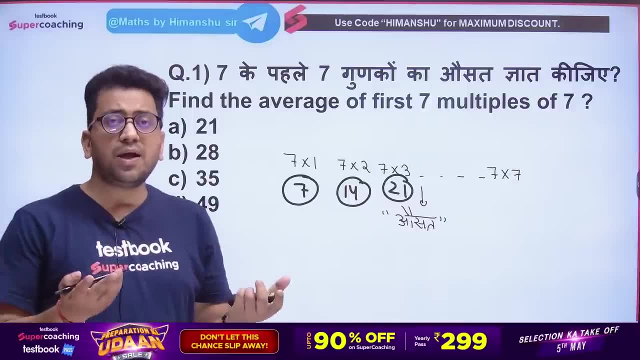 Absolutely, Because these are the multiples of 7.. 7 times 7.. 7 times 14.. 7 times 3. 21.. Can you see the difference between 7 and 7?? The difference is equal, So the middle number is the average. 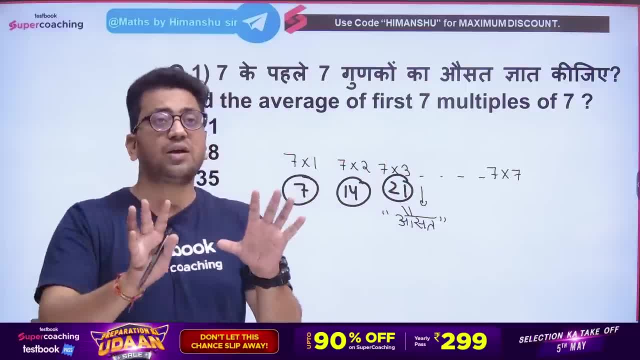 So tell me this: If you have 7 numbers, my son, 1,, 2,, 3,, 4,, 5,, 6,, 7 are there. So, brother, put 3 aside here. Put 3 aside here. 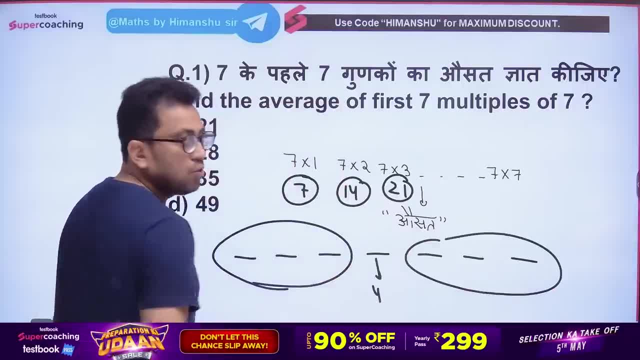 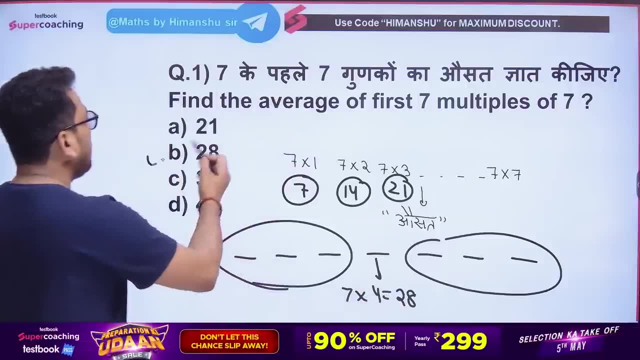 That is the fourth number is going to be our average. So our child does not do anything. Our child directly multiplies 7 by 4.. And 28 is the answer. That is the option is also our answer. The fourth multiple of 7 will be our average. 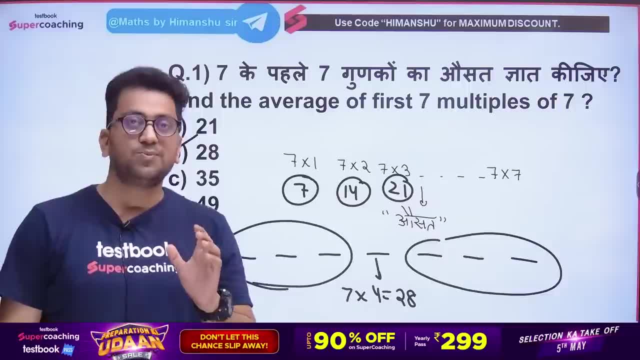 Because it will be the number of the middle. Are you able to understand the thing? Are you able to understand the feeling, son? Are you able to understand the feeling? See the next question. The next question is coming in front of you. 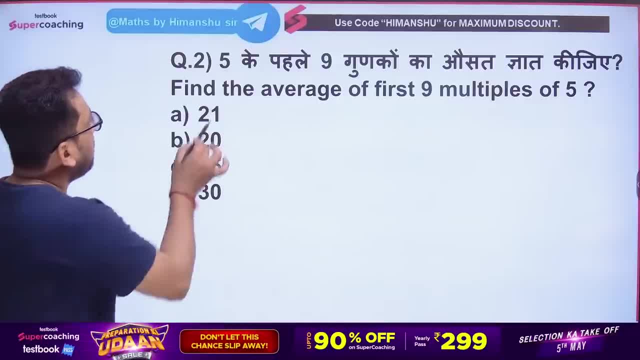 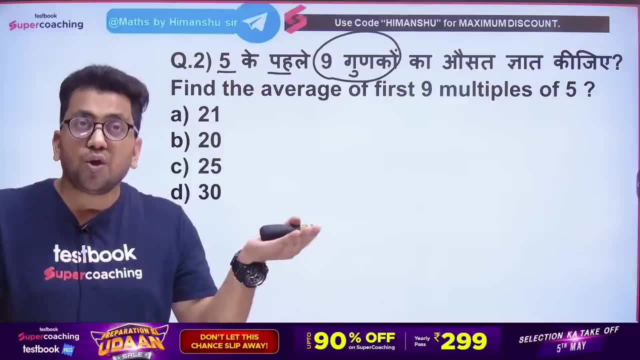 I would like you all to give the answer to this question. Remember the average of the first 9 numbers of 5.. Okay, How many multiples are there? There are 9 multiples. Whose are they? Of 5. That is, there must be an interval of 5 by 5.. 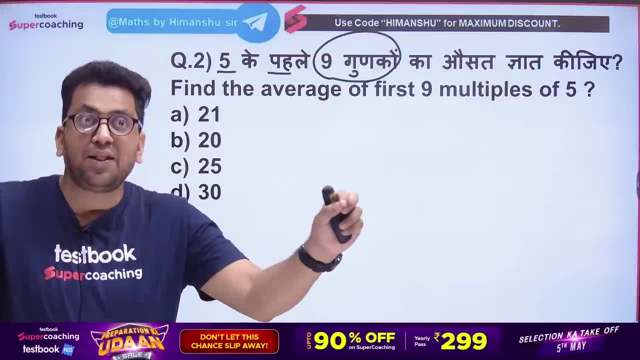 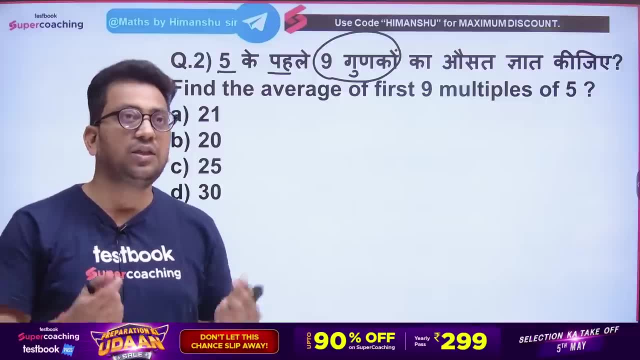 And if there are 9 multiples like this, there are 9 multiples. Then just see which number will come in between. Hurry up my son, Tell me what will be the answer. All of you, With speed, I am setting a timer for you here of 20 seconds. 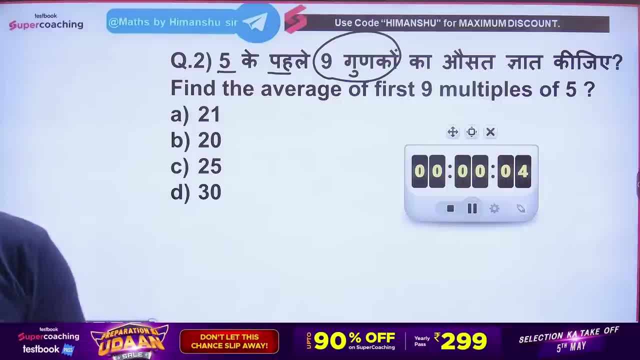 I want an answer from every child. Hurry up and answer the question. We will open the door when I am ready. If you are ready, then call me. you will be ready. You can tell me the correct answer. I will take your number. 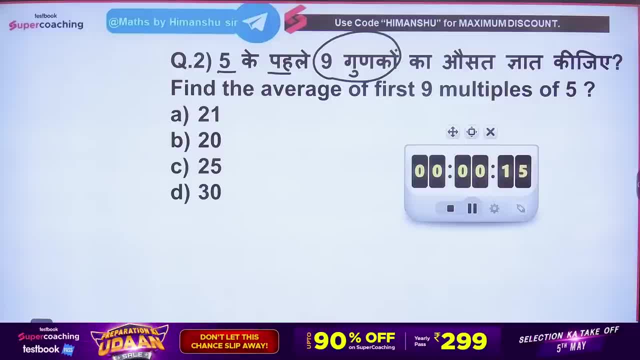 And here is the total number of the kids, That is, we will take the number one, two, three, four, five. And I will tell you that: number one, two, three, four, five, And if two is two, then I will take two. 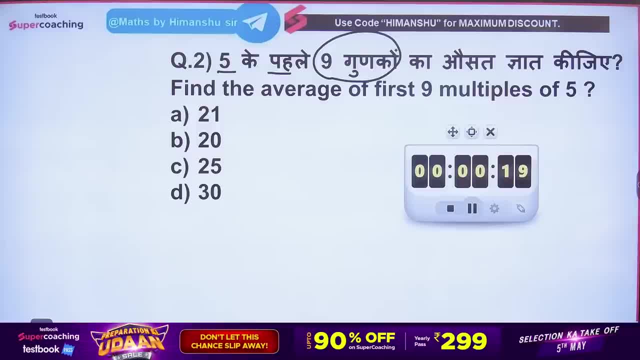 And the answer is B. That is now you will ask for B. This is the number for B, That is, if two is two, three, four, five, Then it is also B. That is here you have to ask five. 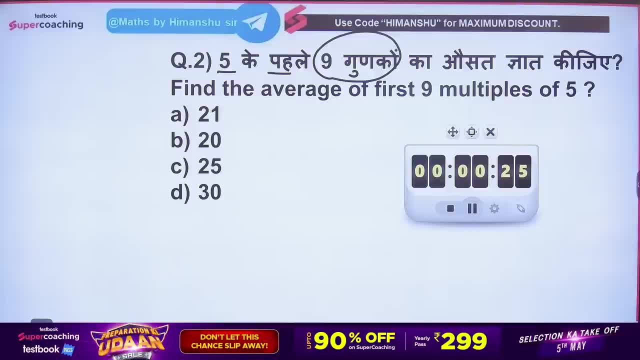 It is one who has more than 50,000, then the answer is A. That is now we know. B, That is, I have to ask B because the answer is C. Like and share is less here. so all the children quickly click on the like and share button. 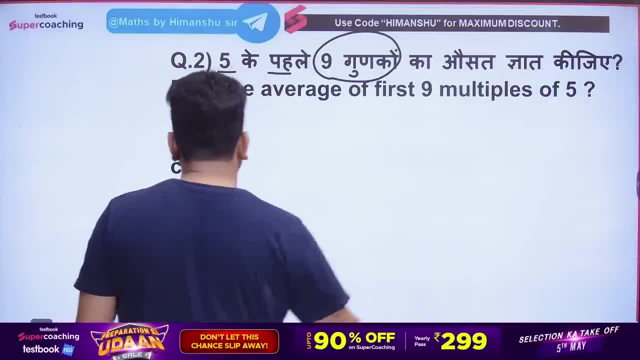 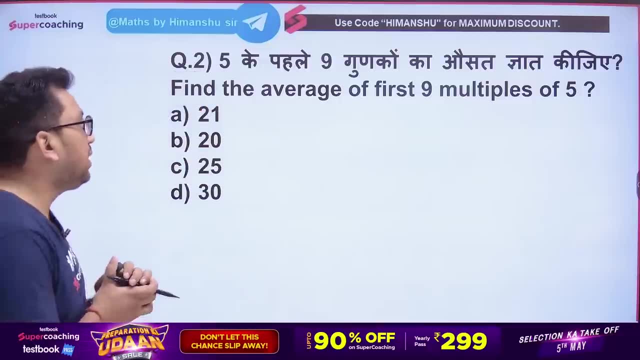 Come here, son, pay attention. He is telling you what will be the ratio of the first 9 qualities of 5.. Very great, See son 1, 2,, 3,, 4,, 5,, 6,, 7,, 8,, 9.. 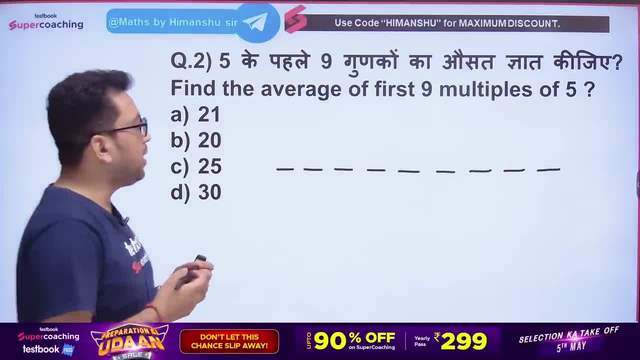 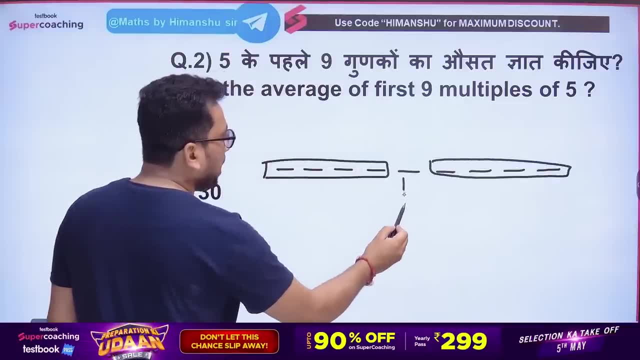 These are 9 qualities. If I say in these 9 qualities, then you have taken out 4 here first and 4 you have taken out there first. That is the 5th factor will be our answer. And who is this 5th factor? 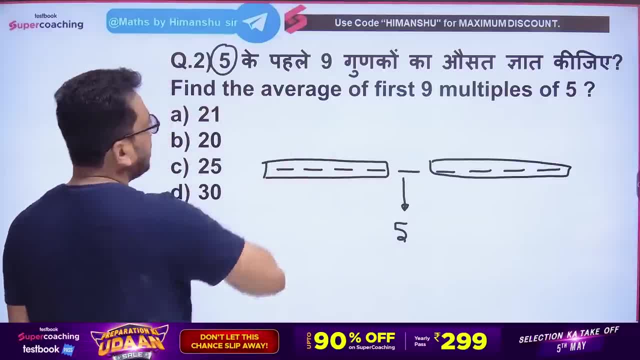 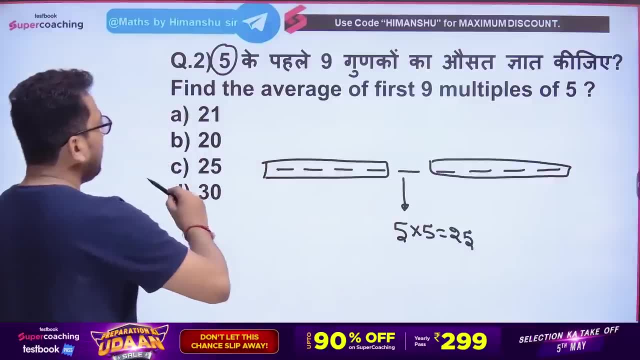 Sorry, yes, who is this 5th factor? It is 5.. That is, if we multiply 5 by 5, then the answer will be 25.. What will come? 25.. That is, this number will be 25.. 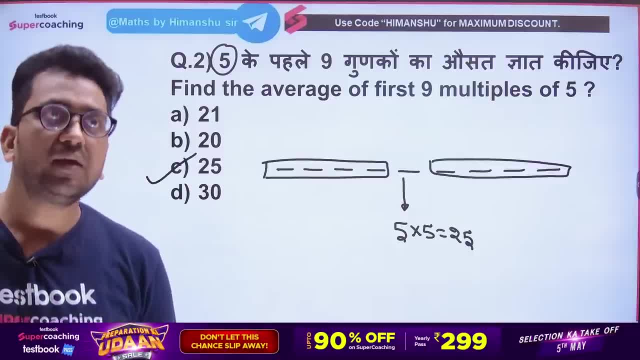 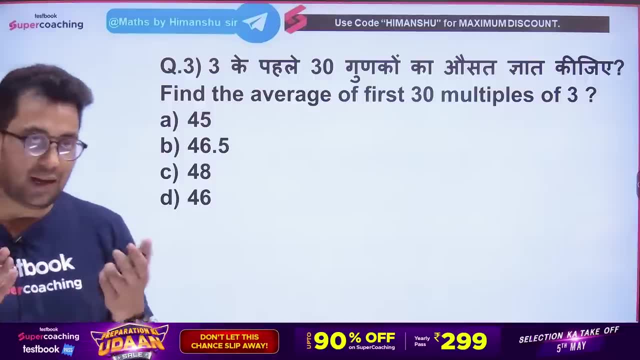 That is the answer is C. Okay, Okay, Sasa Ram, Welcome son, Welcome son, Come on. so our answer here is absolutely correct. Next question, son. Question number 3 is in front of you. We will answer quickly. 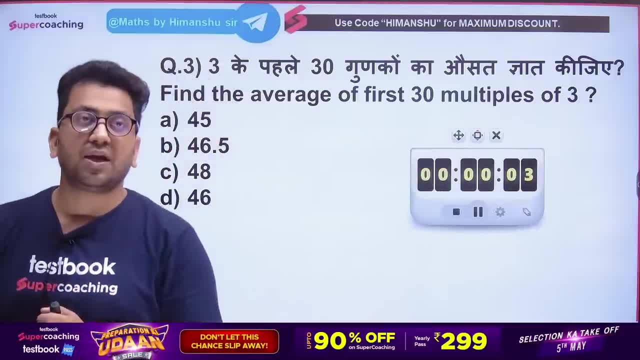 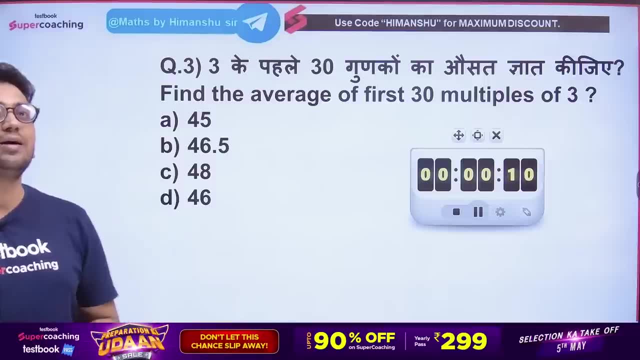 All of you have a timer set here for all of you of 20 seconds. Fly, son, Tell me what will be the answer. Yes, a child has said a very good thing, that if the number was so much, if it was 8,, then 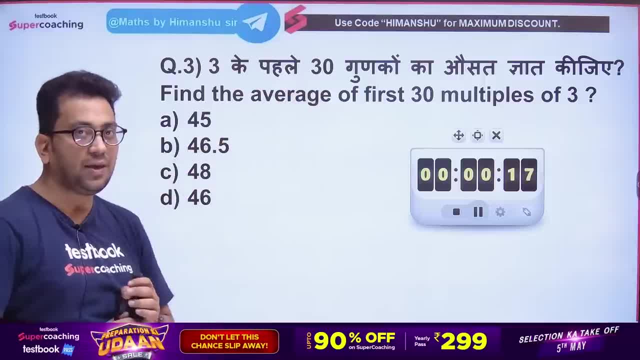 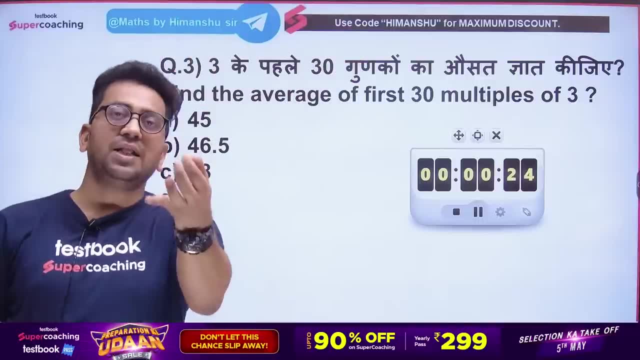 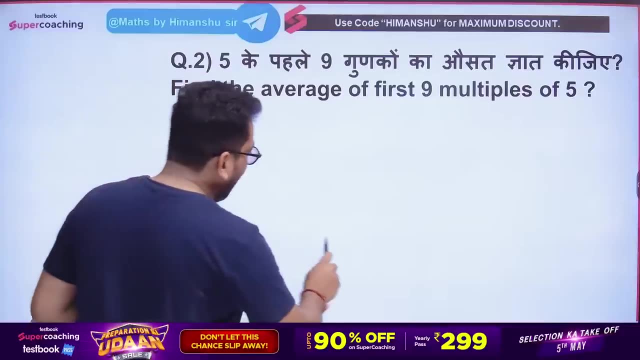 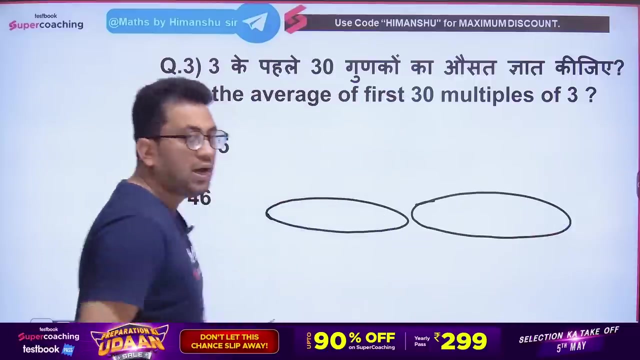 I have taken this question here to erase your same dilemma, See See. And if we will do theCamber challenge, that's confirmed. And if I tell you the answer, I hope this challenge happens when the correct answer, the case has been removed, then in that case how it will be determined, when we will say: 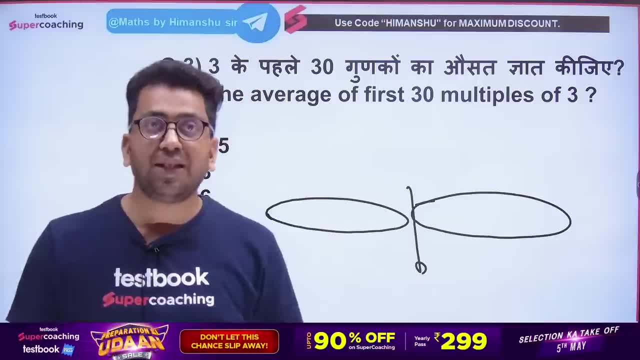 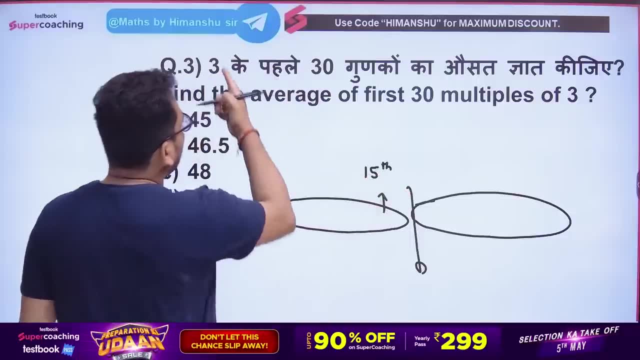 that the house wants to find C avatar Right. Yes, C is 8. in fact, Sir, what is the 15th multiple that we are going to get? Whose is it? 3's. So multiply 15 by 3,, ie 15 times 45.. 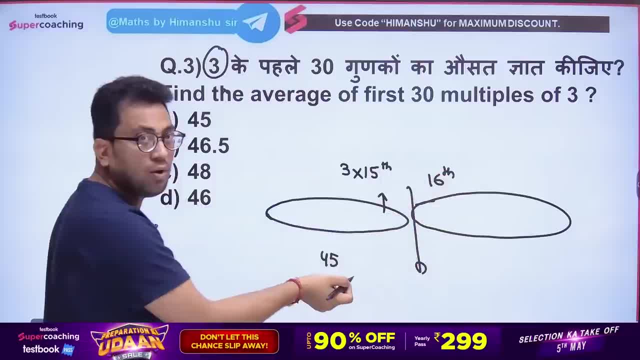 Sir, what is the 16th multiple that we are going to get? After 15, only 16 will come Next one. So what is the 16th multiple that we are going to get? We will multiply 16 by 3,, ie 16 times 48.. 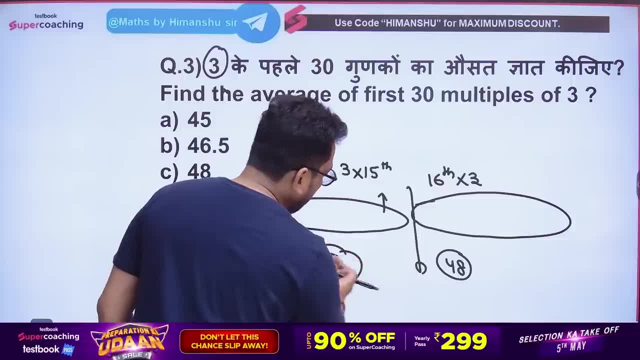 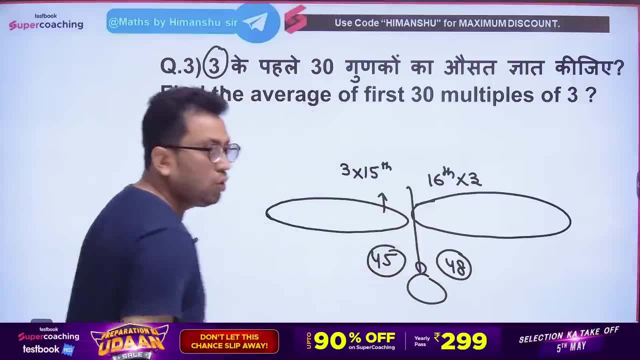 So, sir, the number that will come- between 45 and 48, that will be our material. So how will we know, Sir? add 45 to 48,, divide by 2.. Or you can do it like this: 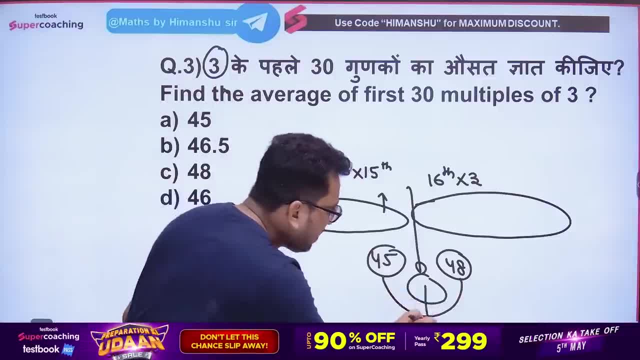 if there is a difference of 3 between them, then there will be a gap of 1.5 to 1.5 between them. The whole gap is of 3, right? So there will be a gap of 1.5 to 1.5.. 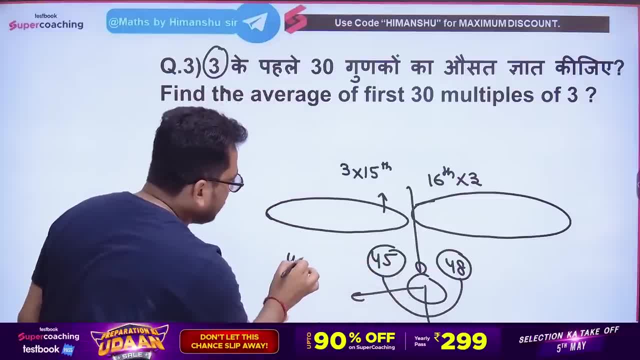 ie more than 45 to 1.5, ie it will be 46.5.. Or I can say less than 48 to 1.5, ie it will be 46.5.. So our option is also B. 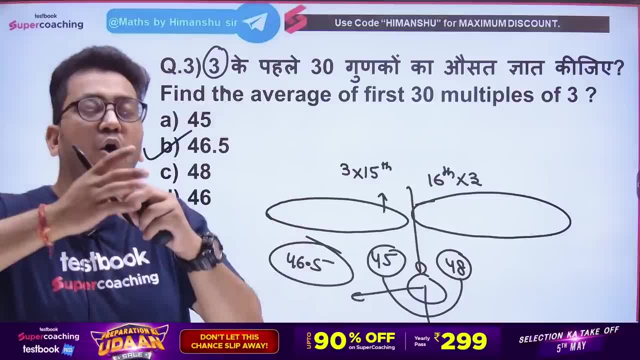 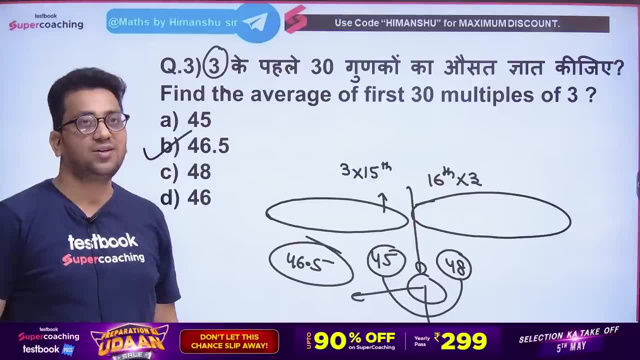 Open your brain. Open your brain, The old time we used to do all these things. get out of them. Understand the feeling of calculation. Okay, do you understand the thing? So we were looking at the middle number. we took out the middle number. 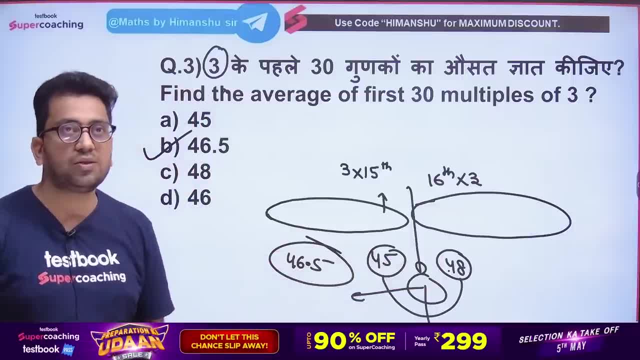 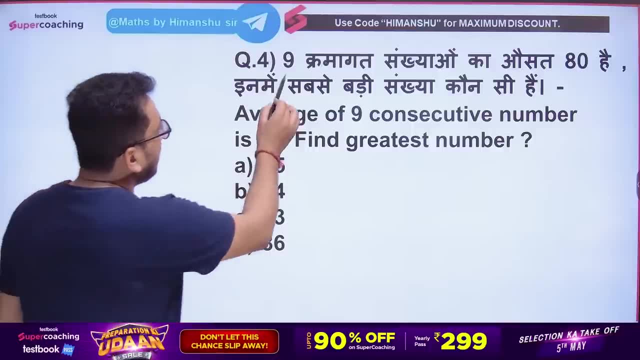 Is the matter clear. If you add both and divide by 2, this will come Next question. The next question is coming in front of you, Question number 4.. I would like every child to answer me. It is said that if the average number of 9 parameters is 80,. 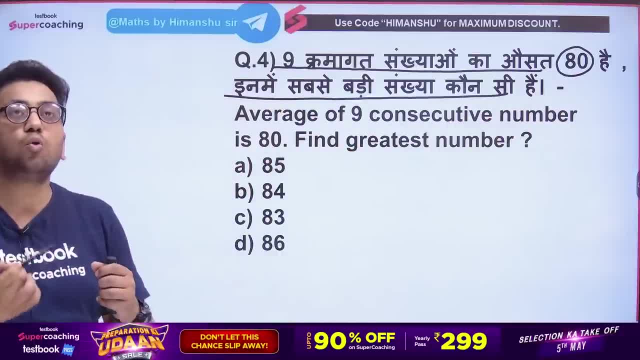 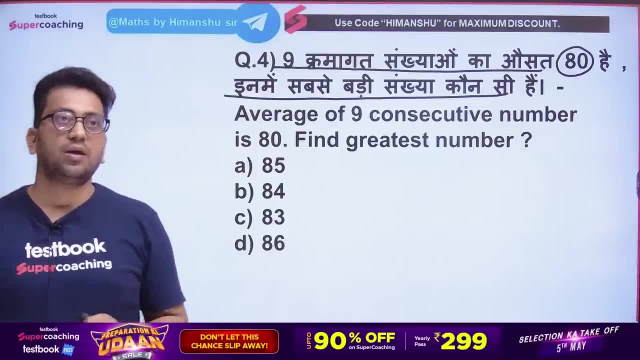 then what will be the largest number? This time in the question there is a slight change in the number of parameters, But we are going to use the same concept, the same concept. Okay, Yes, Okay, See, once again, tell me. 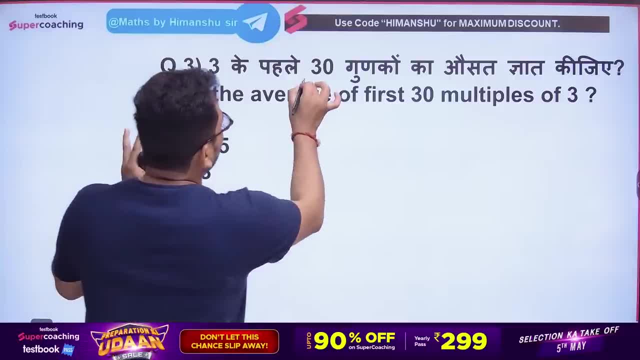 I know it is a little difficult for you people. See, tell me once Quickly, Don't look here and there, next to each other, next to each other. those who are sitting next to each other, kick them. I am saying the right thing. 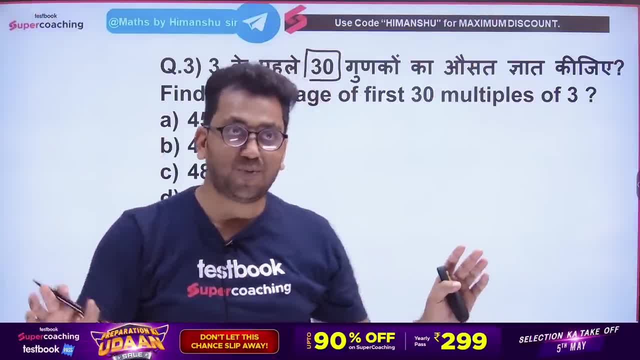 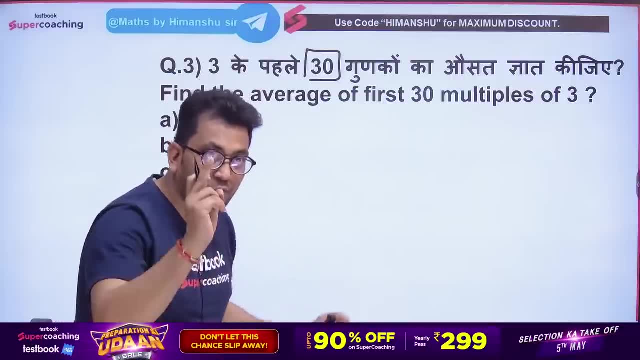 Because your attention is wandering. If your attention is wandering, kick them And say: brother, I am studying, let me study, Okay, Kick out, Okay Say: run away. I just want to study And focus, Focus. 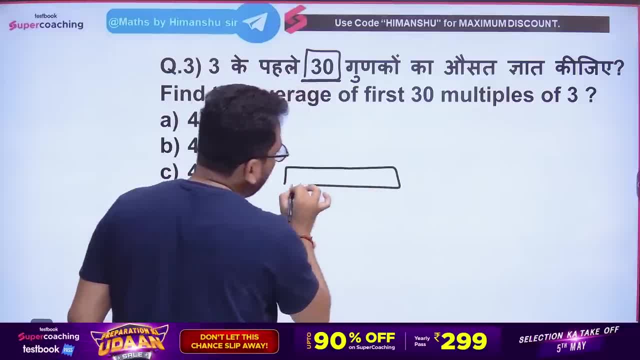 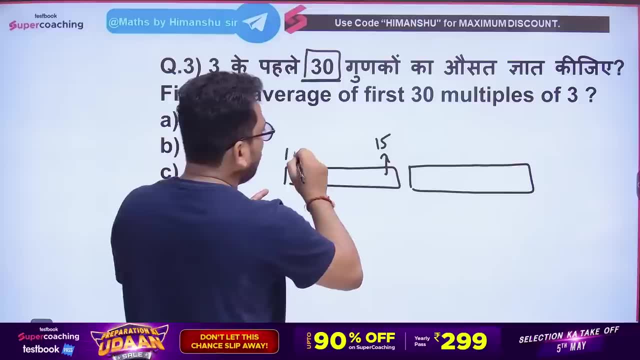 Brother, how many multiples were there? 30 multiples. So tell me that the first 15 multiples and the last 15 multiples will be the same, From 1 to 15.. From 1 to 15.. Say yes. And from 16 to 30, these will be the last multiples. 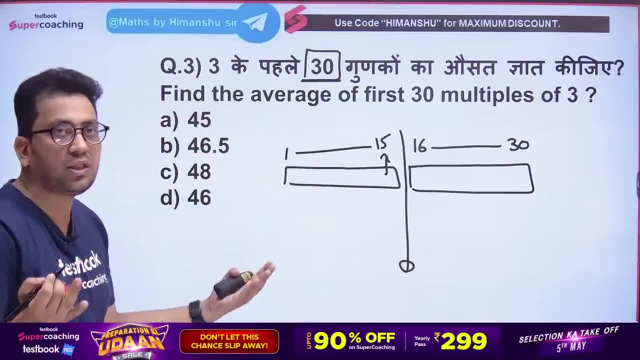 Sir, the number that will be the middle, that will be called the average. So tell me what will be the 15th multiple. Whose is it? Three? So, son, 15,, 30,, 45,. this happened. 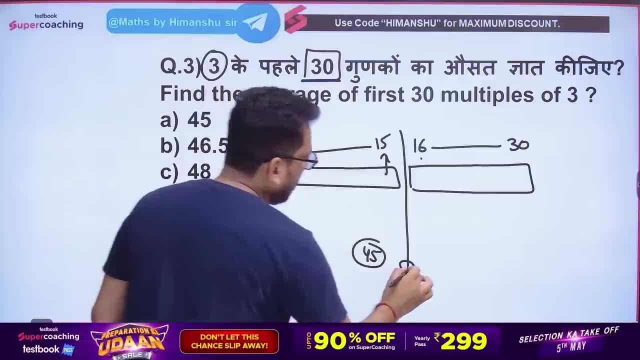 Multiply by 3.. And 16,, 30,, 48, this happened. That is, tell me the number between 45 and 48, how much will it be? Now, one way is that brother join both of them. 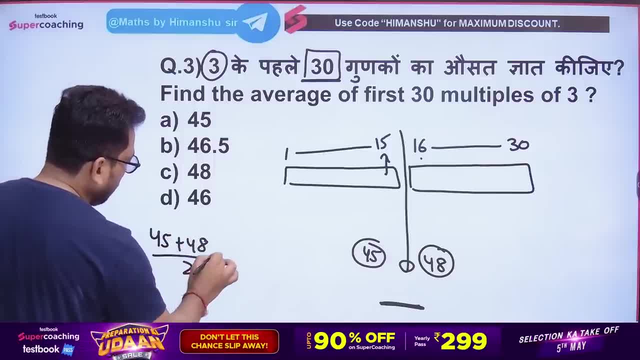 Divide by 2.. The middle number will come. Why are you getting worried? 8,, 5,, 13,, got it. Divide 1, 93 by 2, brother, This will come 46.5.. 46.5 will come. 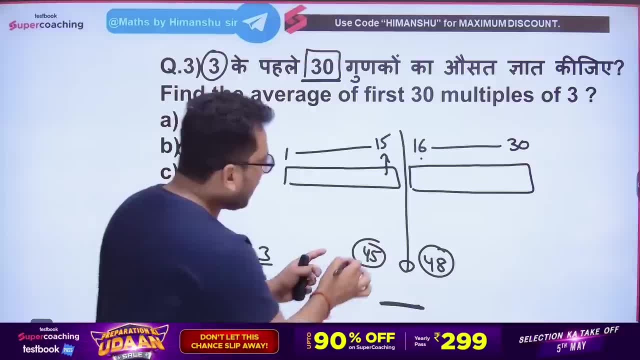 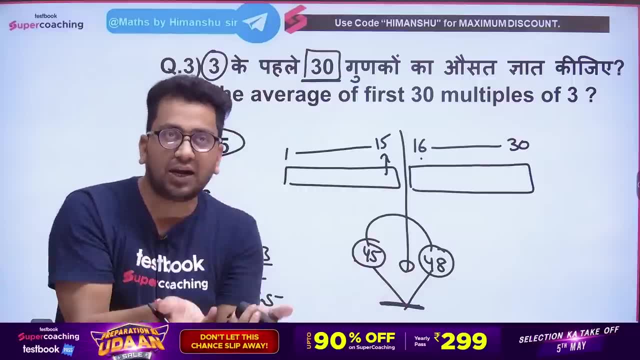 Or I said that if there is a gap of 3 between them, then the middle number will be at a distance of 1.5 to 1.5 from them. Brother, half of 3 is 1.5.. So open your mind a little. 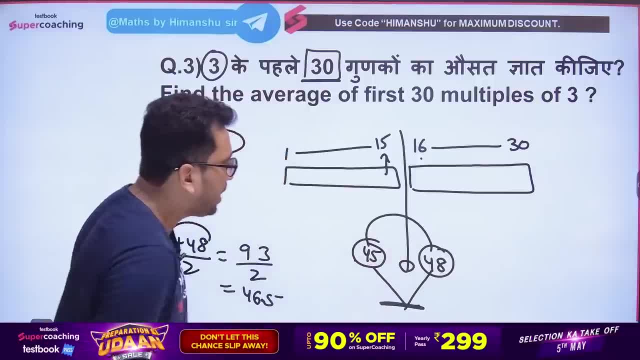 So, brother, if there is a gap of 3, then there will be a gap of 1.5 to 1.5,. my son, That is, this will be more than 1.5, or I can say that this will be less than 1.5.. 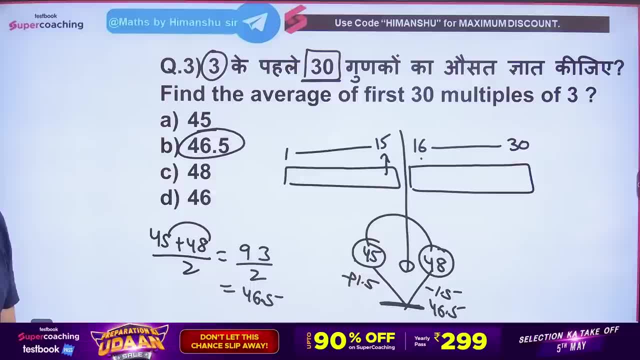 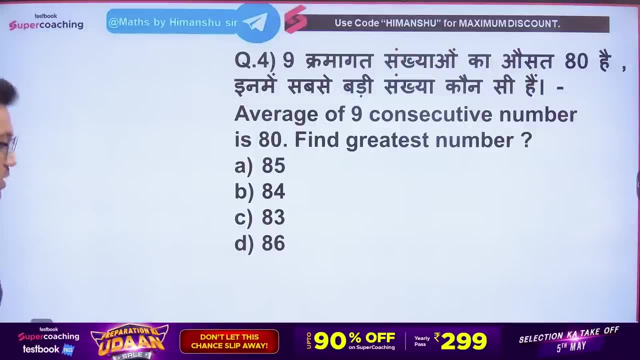 So I said that it will be 46.5.. I wrote it like this. That was the thing. Can you understand? Can you understand? Next question: Now let's come here In this question. what did he tell you? Look carefully. 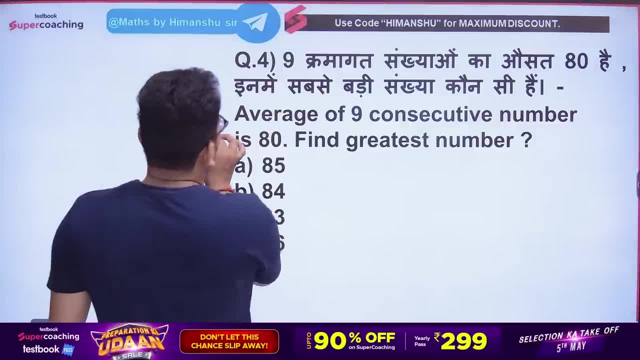 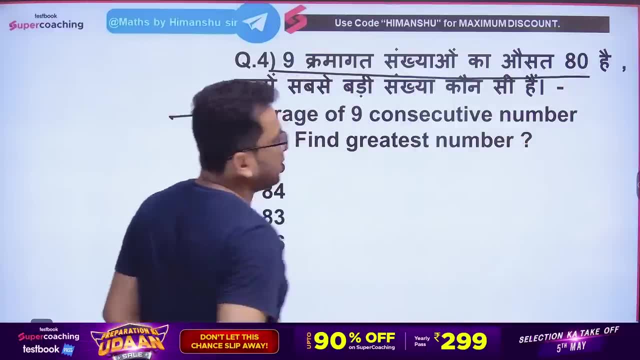 Very good, I can see that Aastha is giving the full explanation here. Look carefully. Yes, He says that Aastha is 80 out of 9 numbers. How many numbers are there? First tell me this: It is 9.. 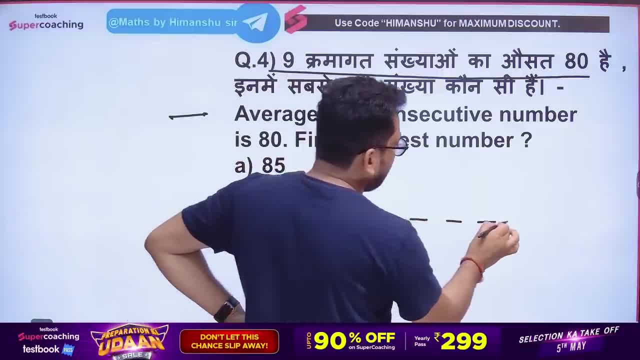 Okay, brother, That is 1, 2,, 3,, 4,, 5,, 6,, 7,, 8, 9.. Hey, you can hit 9 lines. Hit it Now. he is saying that Aastha is 80.. 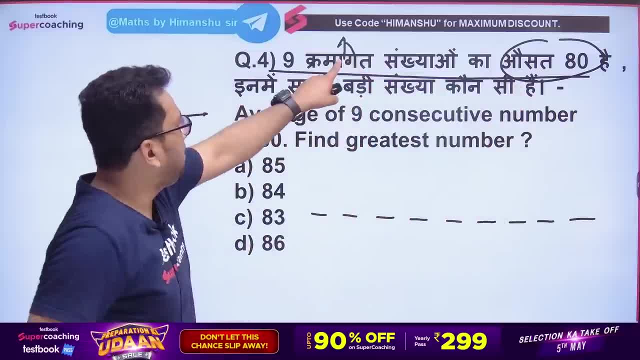 Brother, what is Aastha? If it is a number of numbers, Sir, Aastha is the middle number. If it is a number of numbers, Middle number. So, brother, 1,, 2,, 3,, 4.. 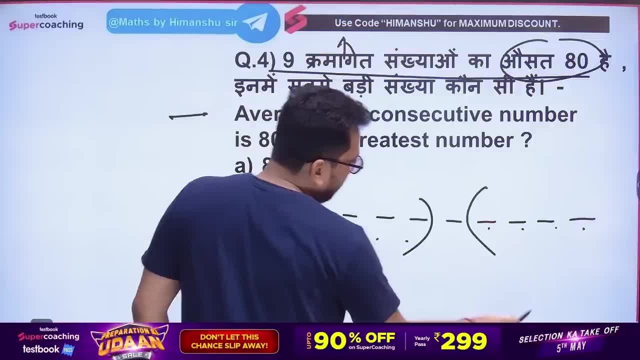 4 is removed from this side. 1,, 2,, 3, 4.. 4 is removed from this side. The middle number is 80.. This is 80, sir. He is saying that, brother, we need a bigger number. 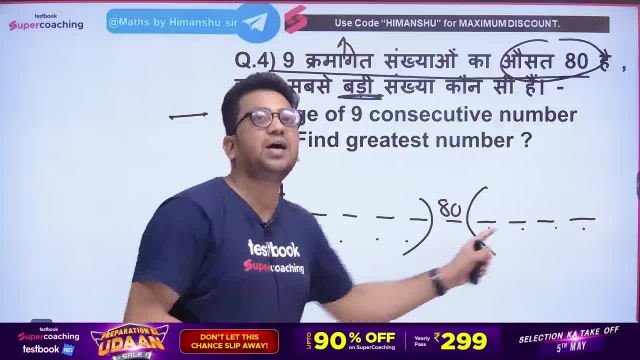 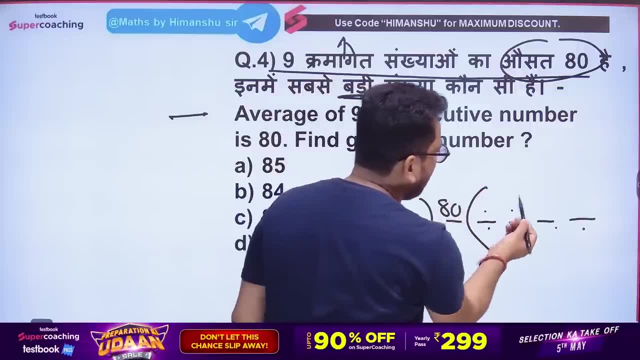 Now tell me, when there is a cycle, it is constantly increasing- then will the bigger number be found there or will it be found here? You will say that it will be found there, sir. It will be found in the end, That is, after 80,, 81,, 82,, 83 and this will become 84.. 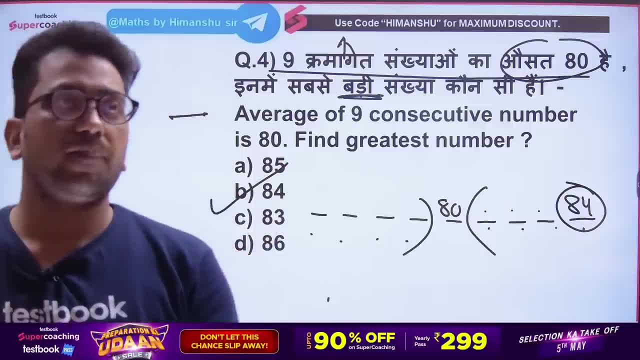 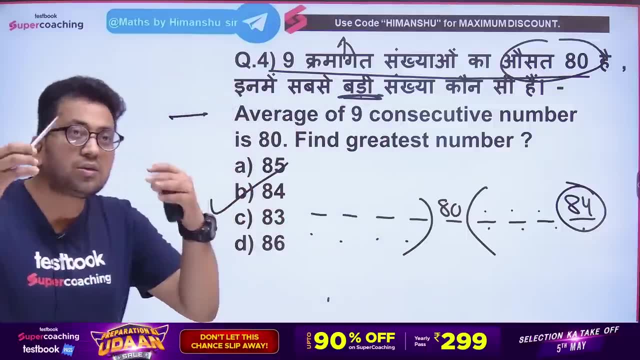 So the option is also our answer. 84 is our answer. Tell me, are you able to understand what I am saying? That is, we can answer many types of questions with just one concept. one example: Yes, 84 was our answer. 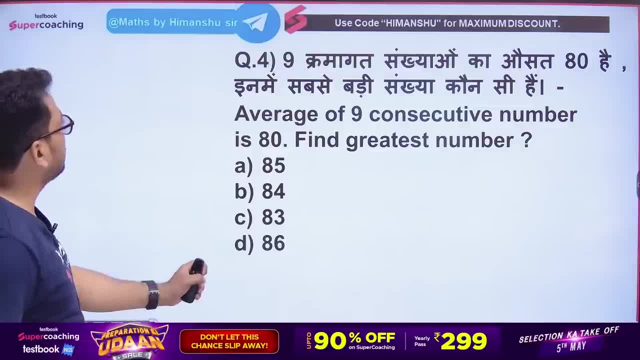 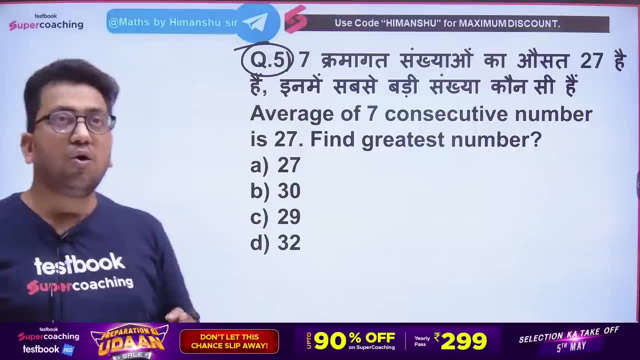 Let's go ahead. Next question, 5th question: Let's see how many children answer this question. If the average of 7 cycles is 27,, then the biggest number should be known. The question is exactly the same, my dear. 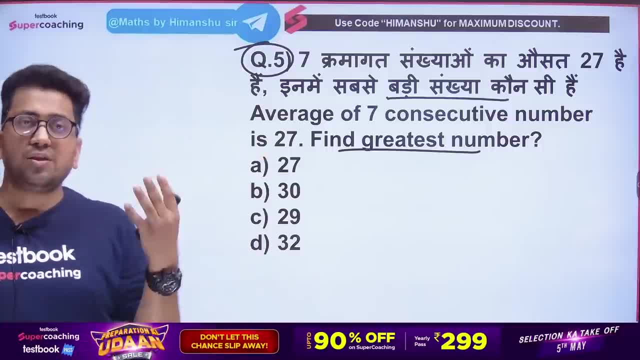 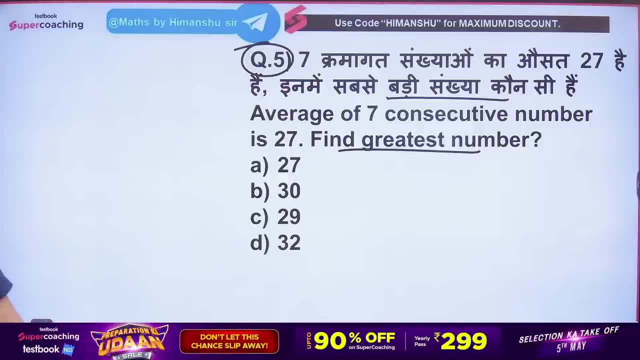 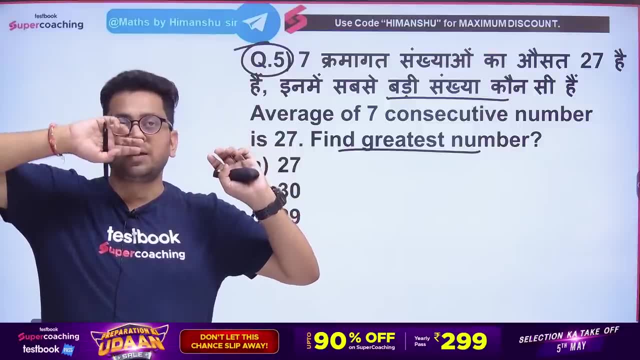 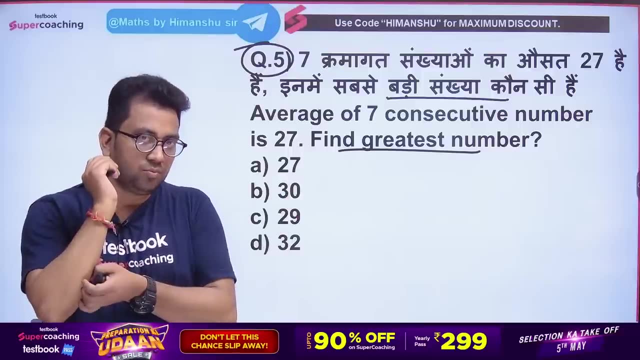 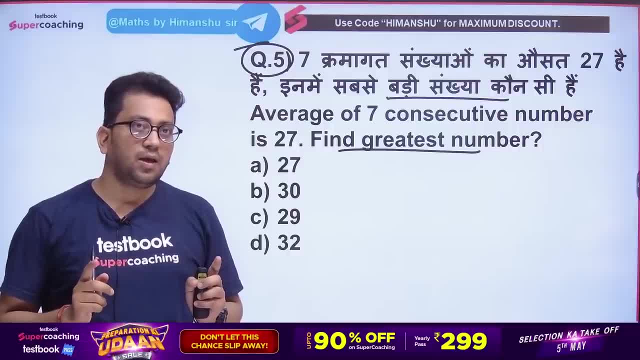 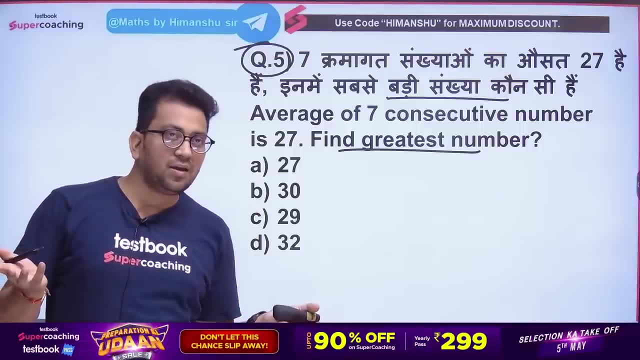 Don't do it like this. If I am teaching from the heart, then read the heart and mind first, Not like this. come and sit. Come and sit and study. The class starts at 12 o'clock. come and join at 12 o'clock. 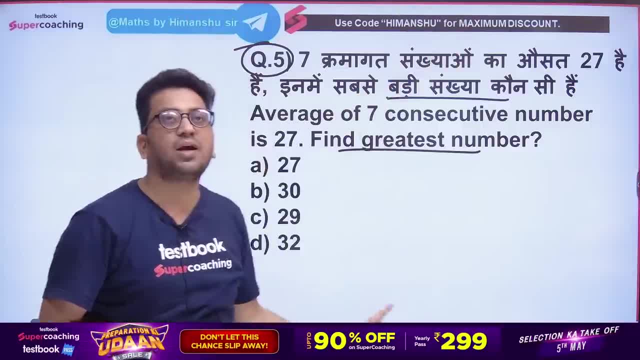 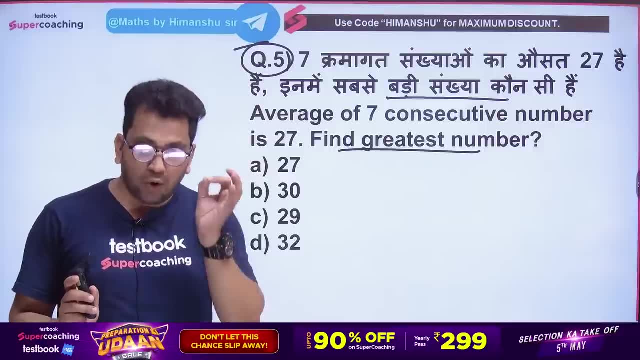 I tell the concept before the class and then ask the question. It has never happened that the question came like this and started studying, for you Never done this. If it is regular, then you understand this thing. So come and join at 12 o'clock. 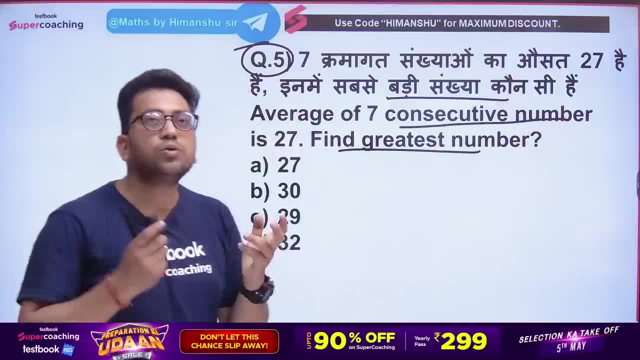 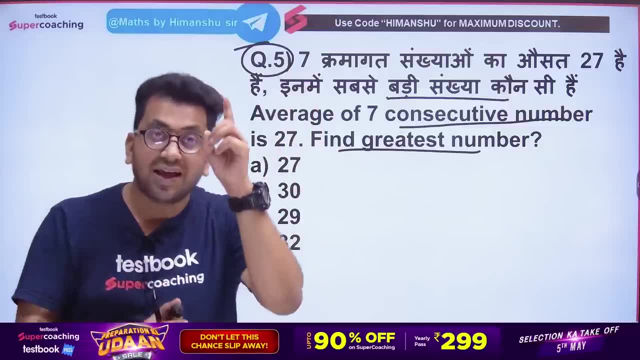 Now come here. What are these? These are consecutive numbers. I told you earlier that in consecutive numbers, In the middle numbers, Why is it regular? I took it out and told you Then I am using a concept. I am not doing it like this in the air. 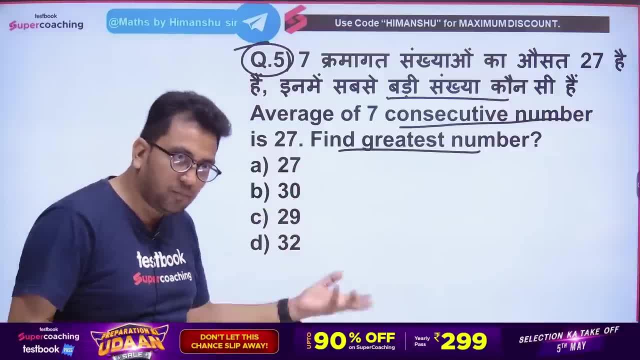 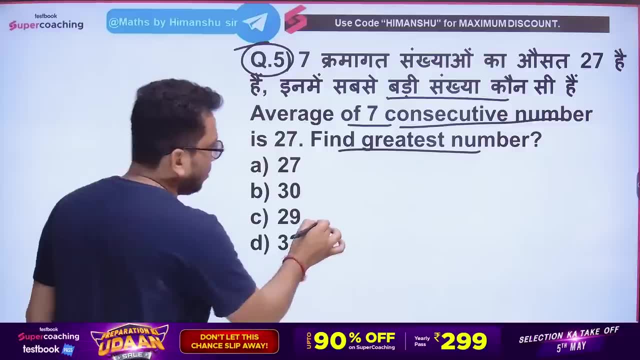 So the hard work you have to do it. Come and join at 12 o'clock, Right at 12 o'clock. So see there are 7 consecutive numbers, So 1,, 2,, 3,, 4,, 5,, 6,, 7 consecutive numbers. 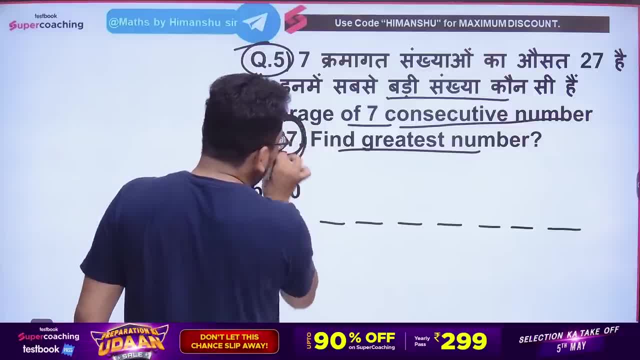 He says, son, its regularity is 27.. What is the regularity? The number in the middle is regularity. So tell me, how will they get the number in the middle? Sir, I moved 3 to this side. 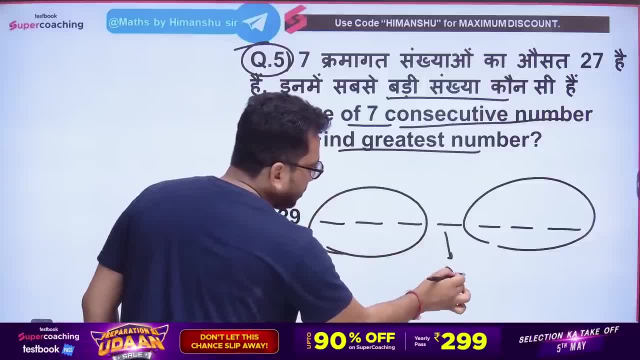 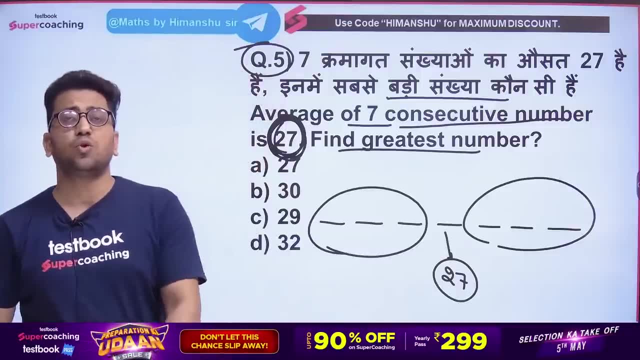 I moved 3 to that side And the number in the middle is the regularity. That is, 27 is the regularity. Say yes or no. Simple sober, the number in the middle will be the regularity. When will it be? 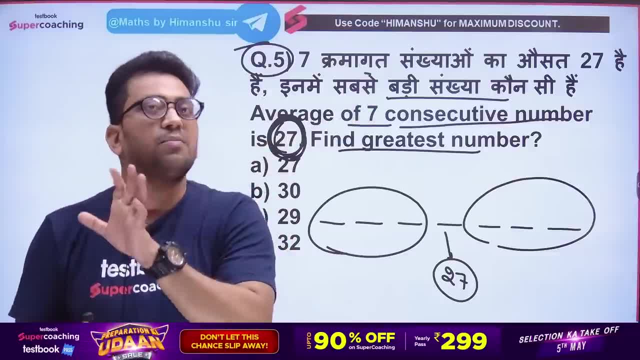 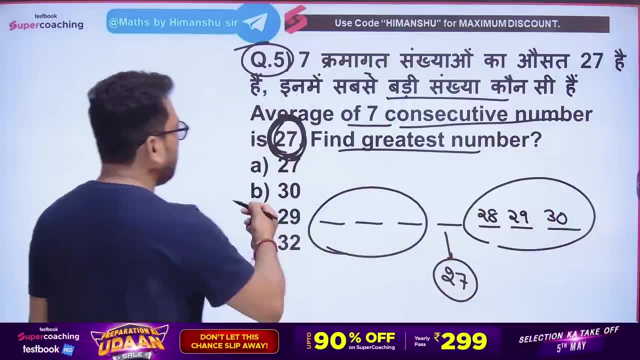 If the numbers are continuous. This is such a system where the differences are equal. Now ask us: what will you get after 27? 28,, 28,, 29,, 29,, 30. So, brother, you will get your answer. 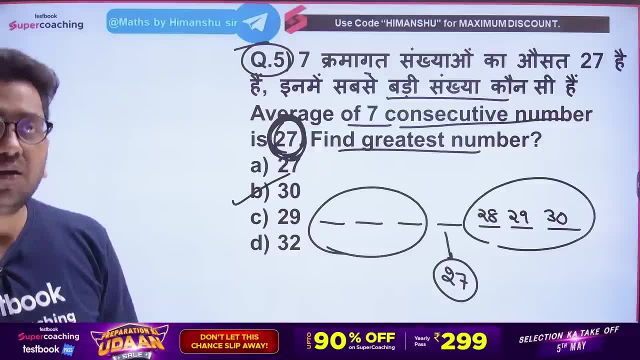 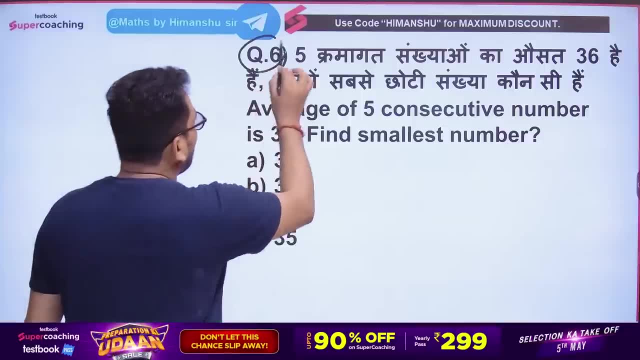 Option number B: Oh, yes or no? B is our answer. Next question. Next question: Son. it will be fun. Why will it be fun? Because it will be understood. When it will be understood, it will be fun. 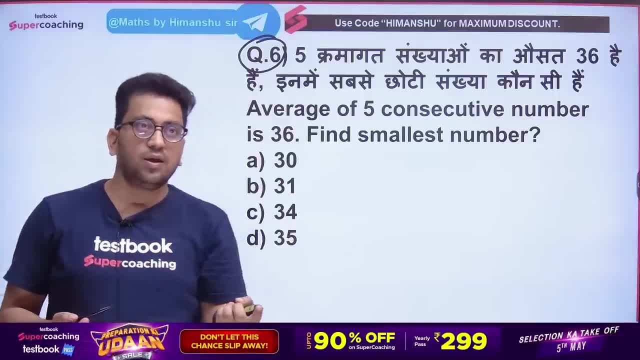 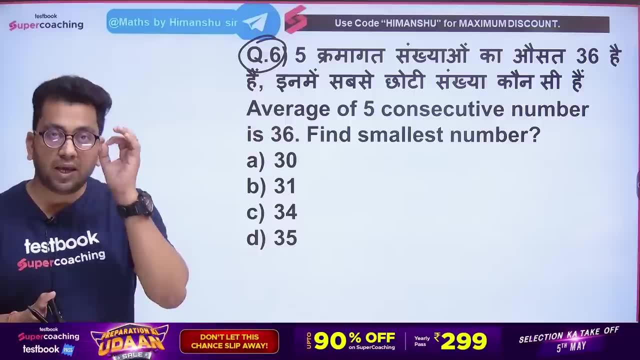 And when will it be understood, Son? when you will come at 12 o'clock, Okay, If you come late, you will not understand anything. This is a guarantee. It will not be understood. I always say that even a good movie, your favorite movie, if you go and see it from the middle son, you don't feel like it. 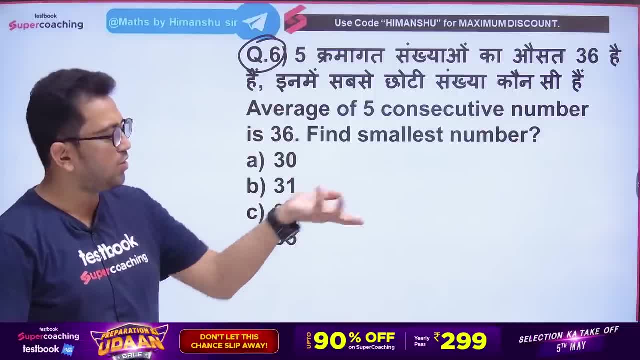 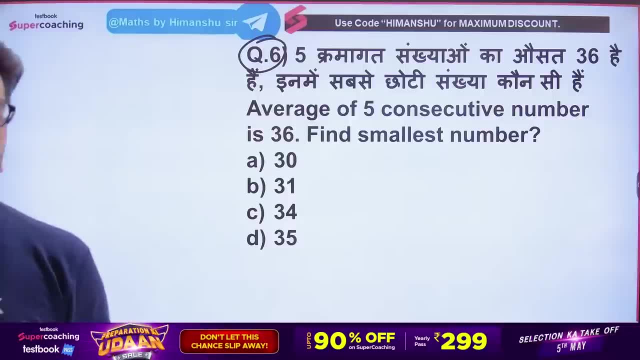 What is happening? Why is this being beaten? Why is the hero beating the villain? Why did he do this? Why, Brother, your brother will also come late, So see from the start. OK, Come and connect at 12 o'clock. 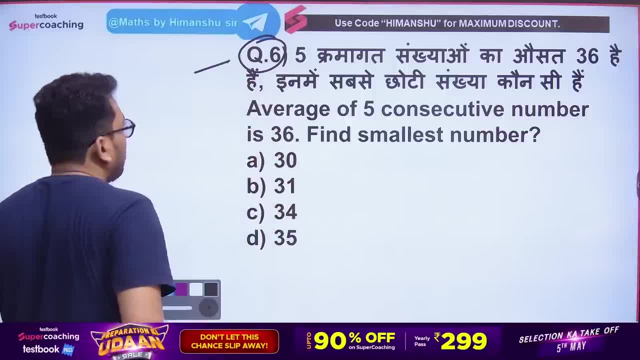 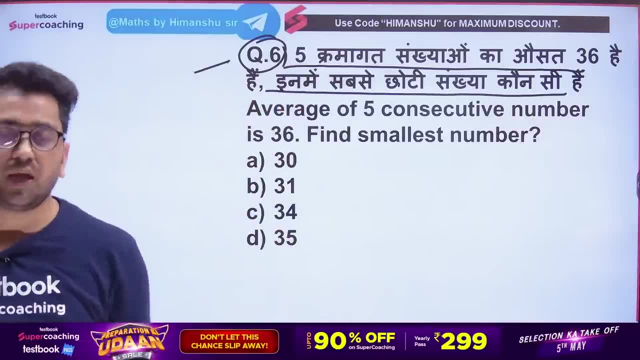 Question number six is in front of you. See what he is saying to you. Five grams are the average volume of number 36.. So what will be the smallest number in them? Brother, asked the chutki chutki. now the question was going on. the old one was now asked for this: 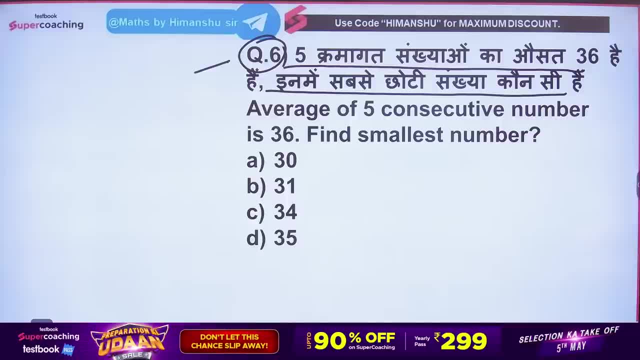 Chutki. Come on, son, tell us what the answer will be. All of them answer. Tell me the answer with speed. All of them, All of them. bhai, 5 kramagat sankhyaon ka osat 36 hai. 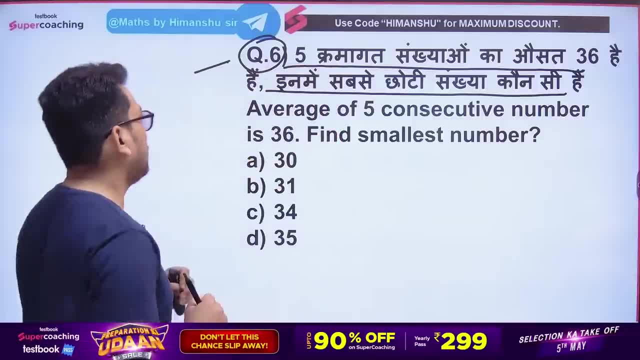 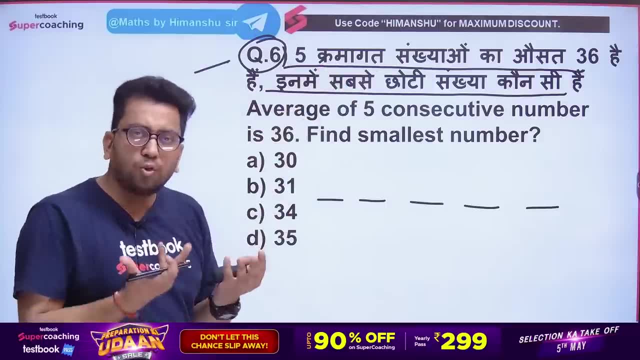 sabse chhutki wali poochli gayi hai, sir 1,2,3,4,5, sir osat kramagat sankhyaon hai toh beach ki sankhya osat yaani ki. yeh hai osat 36 osat hai. 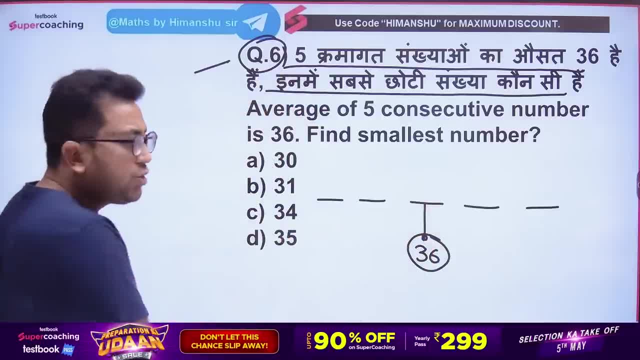 yeh 36 ho gayi beach ki sankhya chhutki poochli chhutki. toh 36, se pehle 35 35 ke pehle 34, toh C apna uttar hai bolon haan ki na. 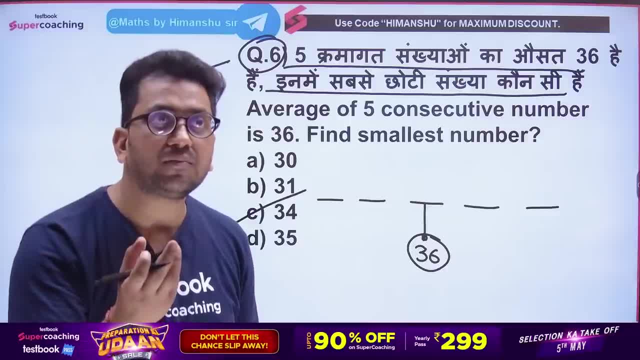 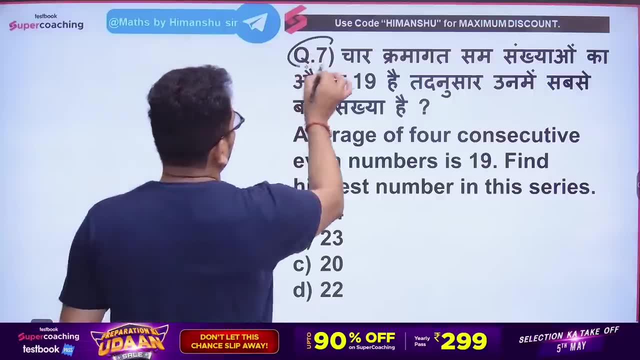 arey kar pa rahe ho, samajh pa rahe ho mera laal samjhoge, samjhoge na kuki concept apko samajh me aage agla sawal. question number 7: maine ap loon ko bola tha telegram par. 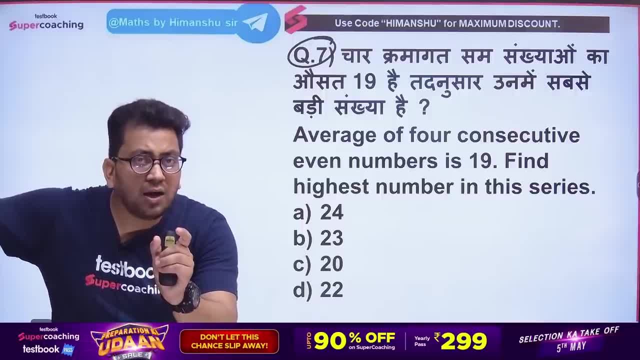 ki is tarike se apko beta gadit karaunga, ki apne pehle kabhi padha hi nahi hoga. kyu nahi padha hoga. arey bachay, ko lagta hai, math hai yaani, pata nahi kya hai. 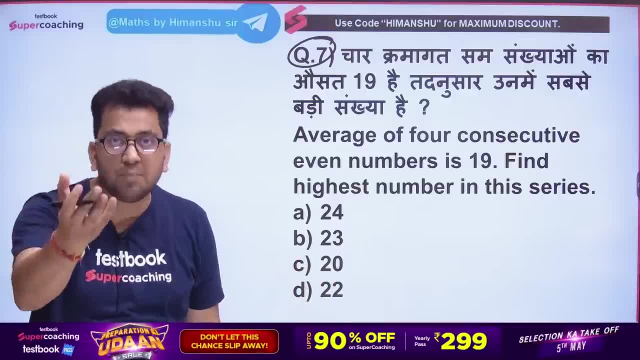 hawa bana rakha hai math ko arey usko padha ho toh sahi, bachay ko us tarike se uske dil aur diman. samajh ki baap tohko. samjho toh sahi wo padhna chahata hai. 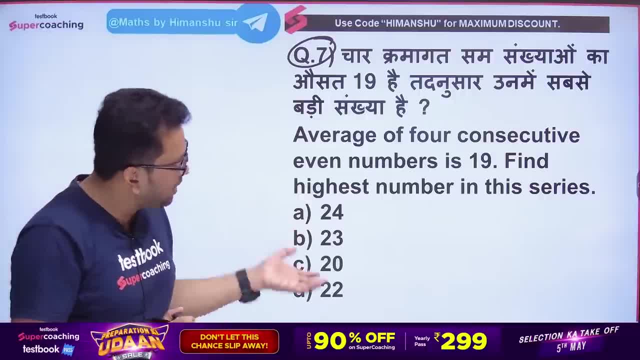 pekin usko tarike sikhau, toh sahi, jo wo tarike sikhega uski khud interest develop hoga, usko khud ruchi aayegi, toh padhna khudi shuru kar dega. 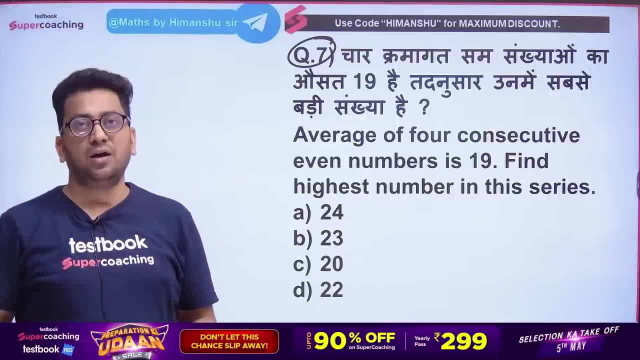 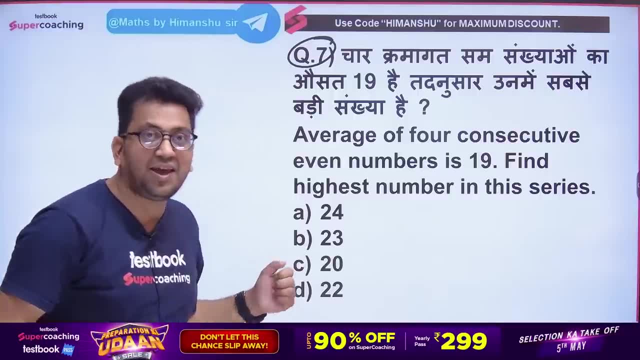 per jo muskil sawal hongi na, wo unko bhi karne ka effort dalega. bhai, jab wo asaan mein hi tum usko aise sikhate chaloge hain, aise se malab, gande, gande se tarike. 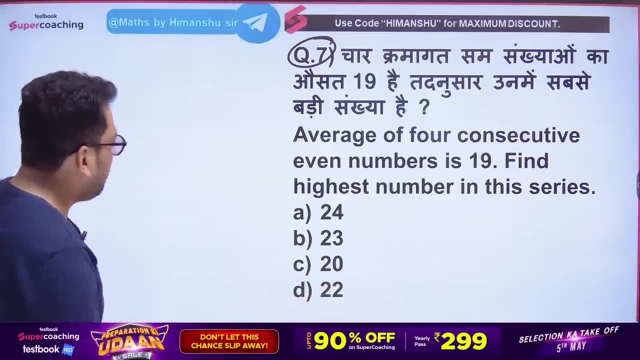 sikhate chaloge. toh bachay. toh aise hi ghabar a jaega 22, 22, 22 answer kar rahe hain: bachay, aao, bhai keta hai 4 kramagat sam sankhyaon ka ausat 19 hai. 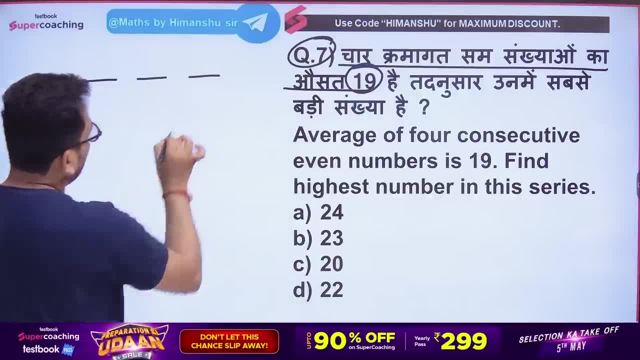 19 hai kitni sankhya hai 1, 2, 3, 4 kramagat sankhya hai ausat kitna hai 19 hai aare sir, 4 mein beech ki sankhya kaise nikal hain. aare beta, aisa batao na sara. 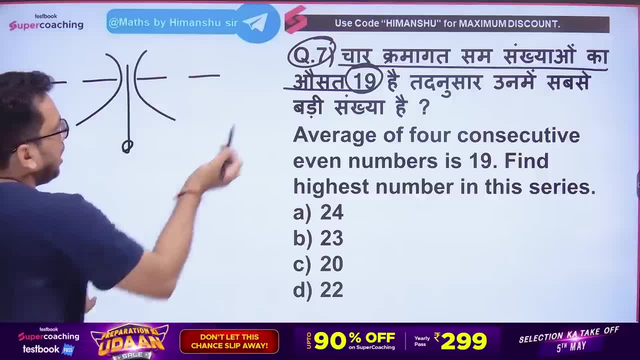 ki 2 ko idhar baju, 2 ko idhar baju. toh beech ki sankhya ausat aare haan ki na toh yaani ki 19 hai ausat ab humse kera hai iske anusaar batao sabse badi sankhya kaunsi hogi. 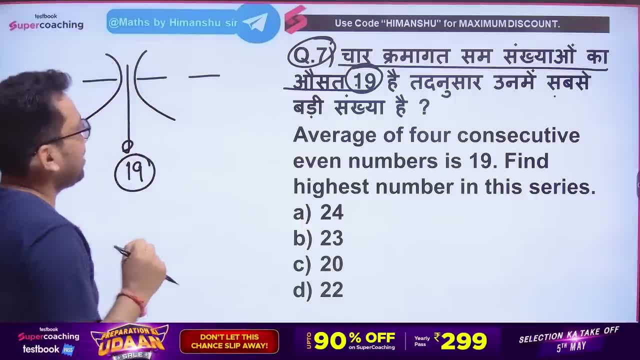 lekin dhyaan se samajh na, dhyaan se samajh na mere laal, kyo yaha par sam sankhya hai bola gaya, yaha par even numbers bola gaya hai, ki nahi, yeh bhi kramagat hai. 2, 2, 2 ka antar chal raha hai. 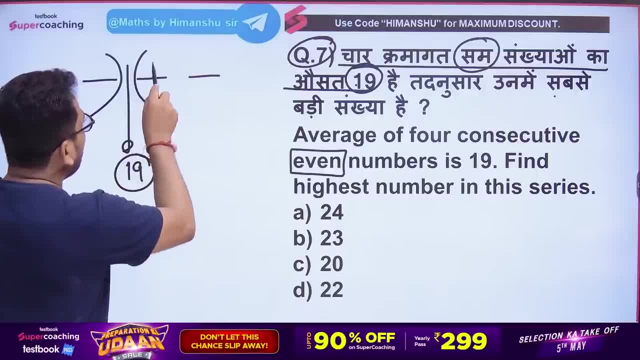 hai, na, toh even hai. toh mujhe batao: 19 ke baad even number, kya aayega 20? aur 20 ke baad kya aayega 22? toh yaani badki, jo sankhya milegi. 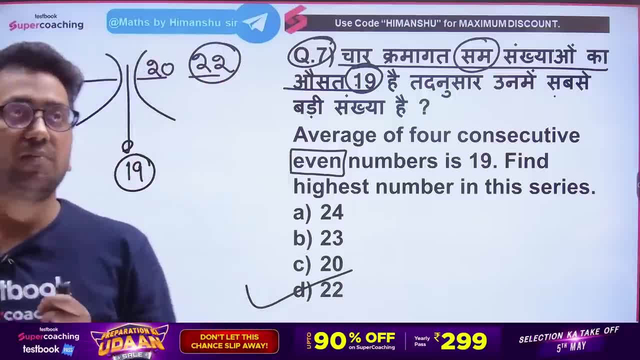 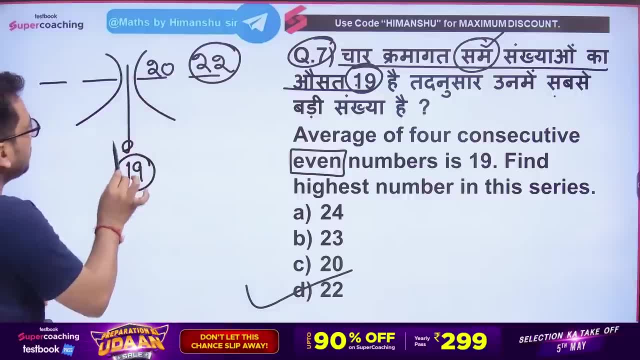 wo 22 milegi, 22 bhi humar answer samajh paare ho. aap toh bohot badya, toh bohot dhyaan se samajhte ho: chalna yaha sam sankhya boli thi. isliye 19 ke baad sam sankhya 20 milegi. 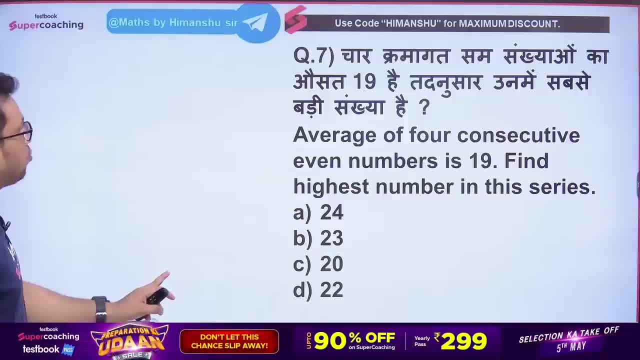 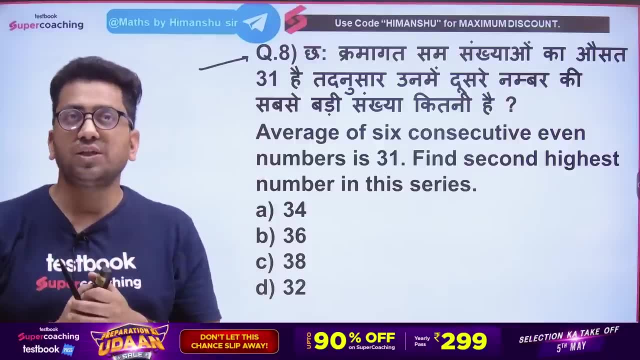 aur 20 ke baad 22 milegi agla sabal kushe number 8, aath ma sabal dhyaan se padna 6 kramagat sam sankhyaon ko ausat 31 hai. tadun saar unme doosre number ki sabse badee sankhya, aapne gyat karne. 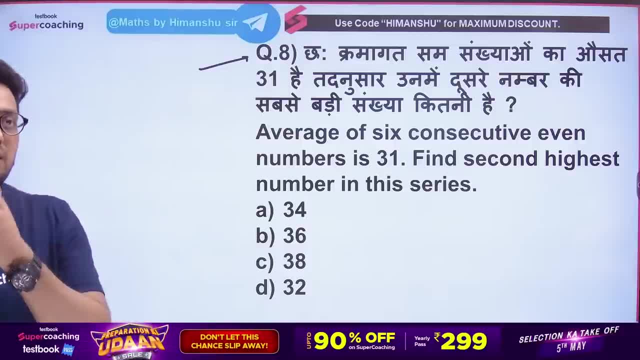 yeh doosre number ki sabse badee, second highest, batani hai. jaldi se bataye, kya uttar aega. chalye 6 kramagat sam sankhya hai. dekhteyan kitne bachche answer kar par rahe hai. 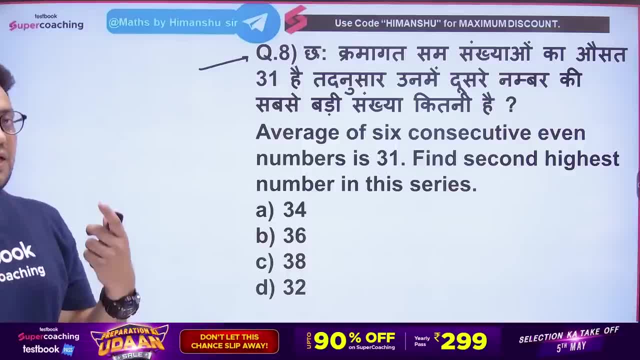 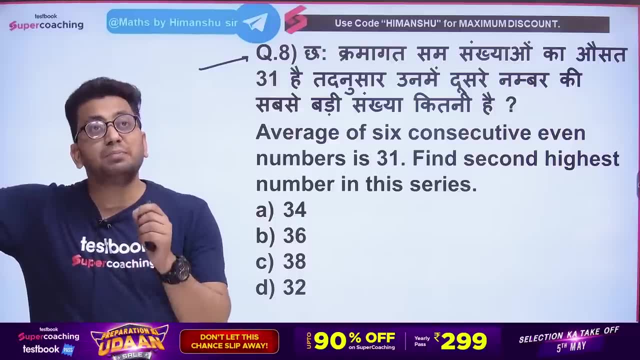 answer kariye achha ek baad sam sakhyan hai. jalde se batae keya uttar aega chalye 6 kramagat sam sankhya hai. I am a little upset with you that when I give you homework you have to answer all of them. 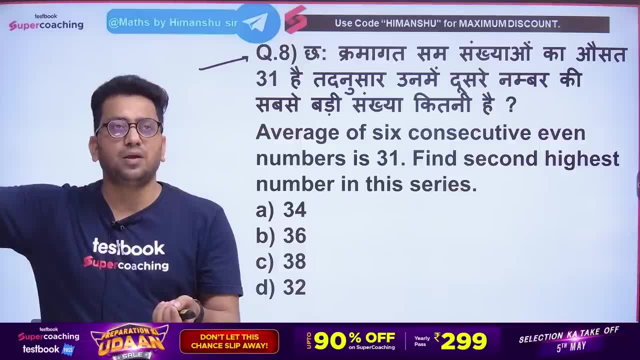 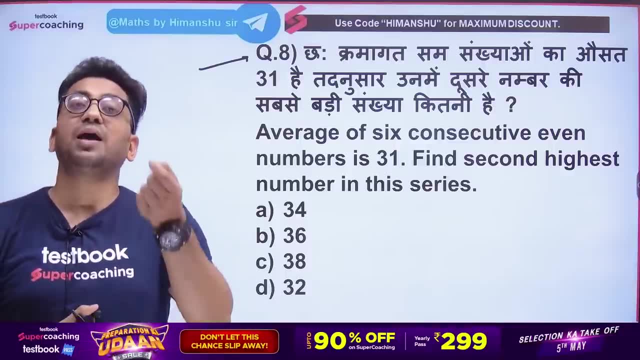 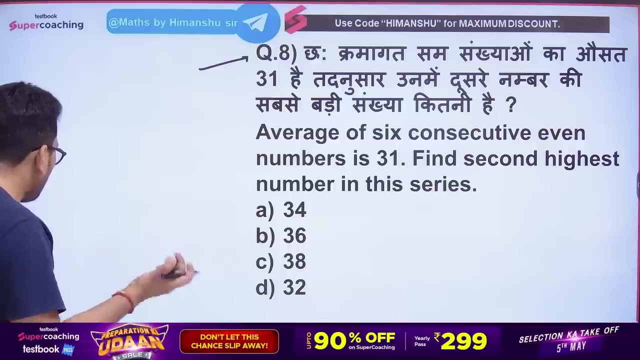 I can see that very few children's comments come. At least those children who are studying live. they must answer the homework question in the comment section. Make your routine, Make a daily answer to whatever question you are given. Make a continuity. See what he is saying. 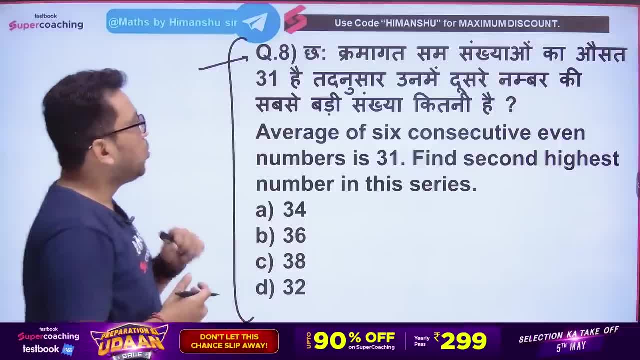 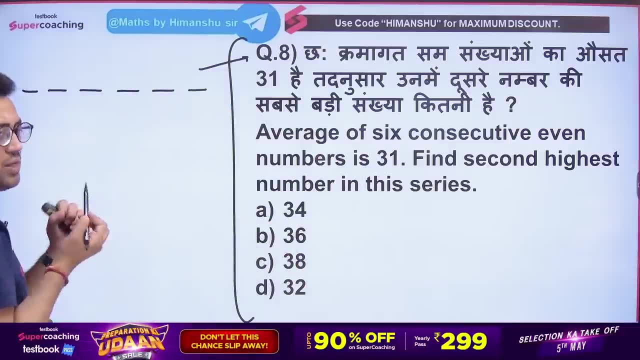 The average of all numbers is 31.. According to that, the number of the second number has to be told: Sir, 6 numbers 1, 2,, 3,, 4,, 5, 6.. Sir, how will you get the middle number? 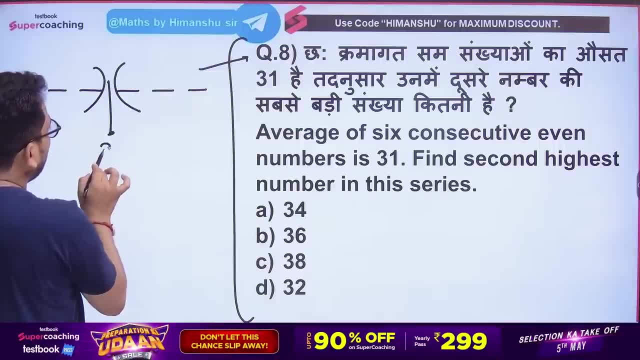 Hey, 3 on the side here, 3 on the side here. removed, That is 31 became. Now what will you get after 31? 32,, after 32,, 34,, after 34,, 36.. 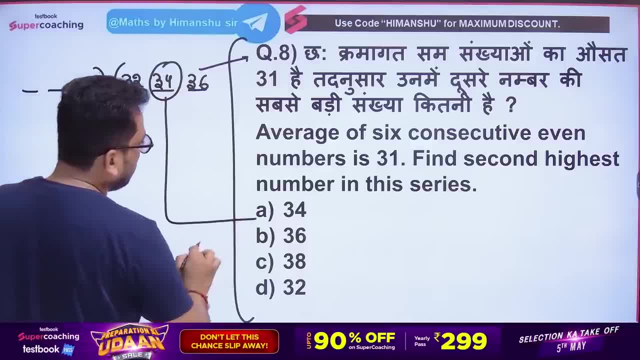 He is saying that the number of the second number is the biggest. then what will you get? 34, because this is the biggest and this is the biggest of the second number, That is, 34.. 34 will be your answer. 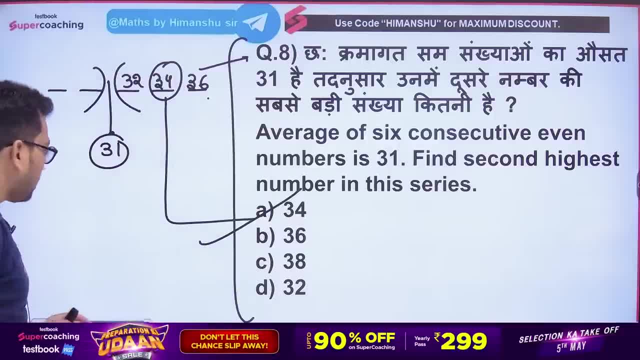 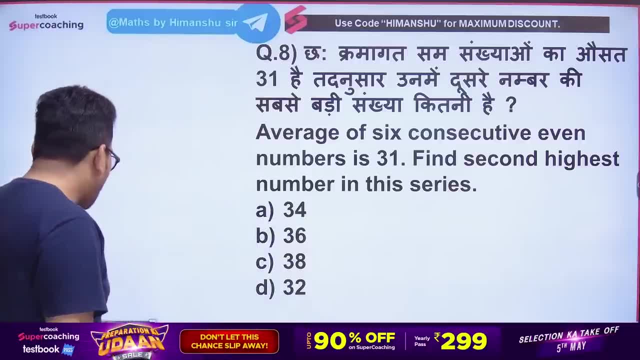 Okay, Yes, very good, Son, I am clapping for those who do it, Okay, And Oh, wow, man, That's what I was thinking about. Come on, come on, come on. Well, I gave the question in the last class. 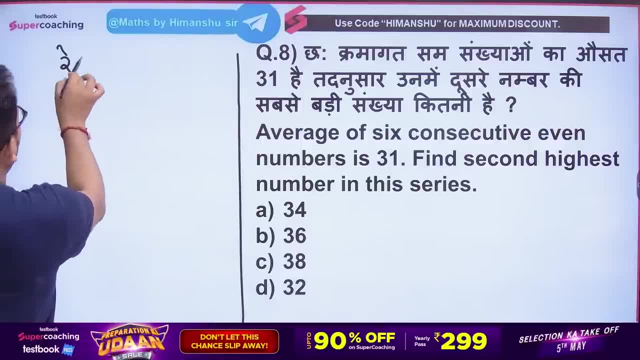 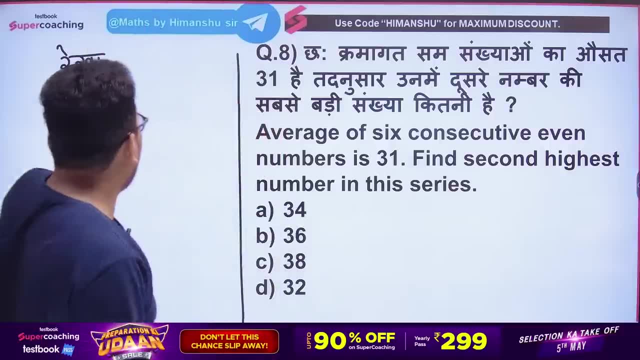 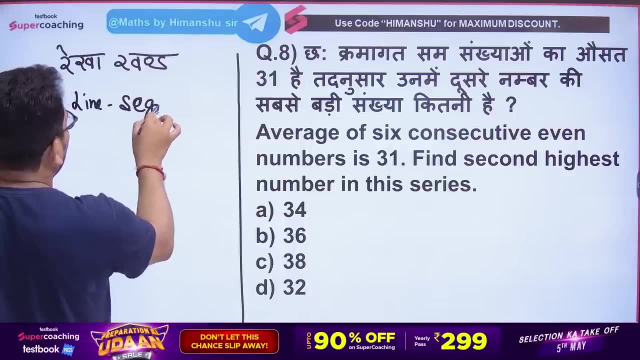 I asked you people that tell me in the line line Once you all will answer me in the comment section, Because today it may be possible that some children are new, So tell me. how many points are there in the line line? How many points are there in the line segment? 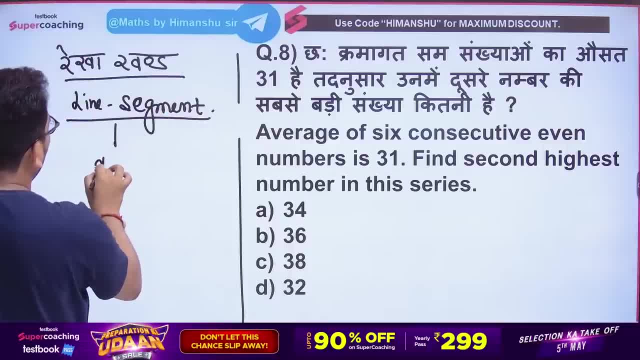 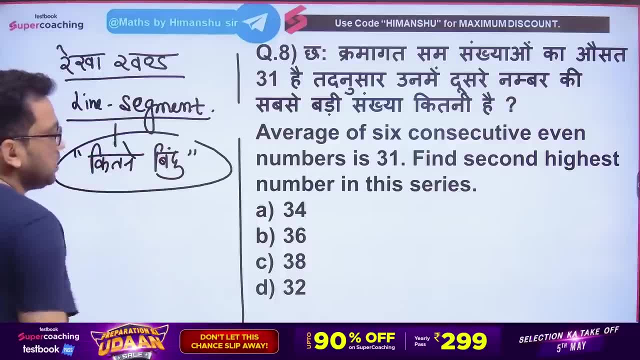 Tell me quickly. How many points are there in the line In the comment section? First, answer me this, Son. I gave you this in the homework, Okay, In the last class, when our Maha mock test number 2 happened. 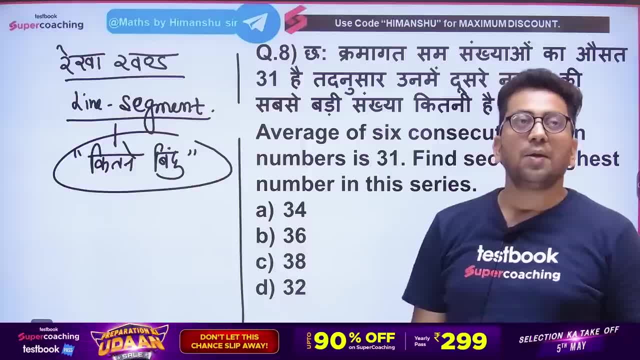 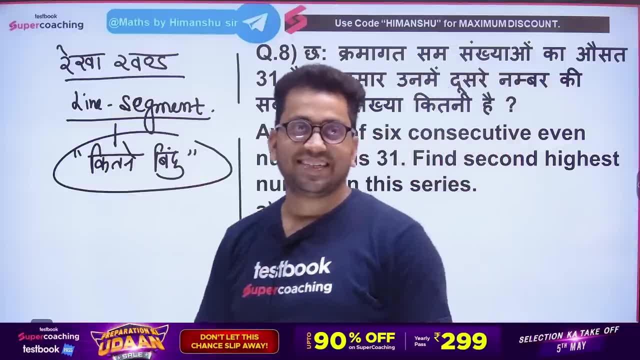 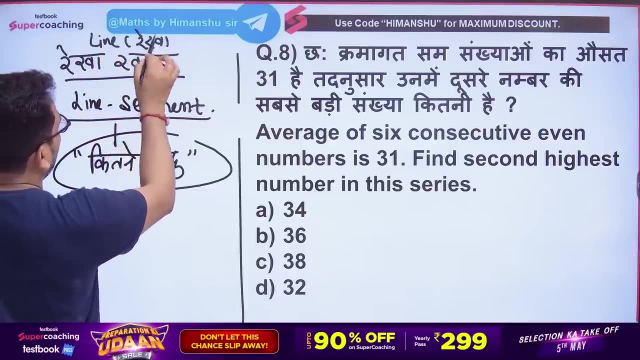 And I can see that few children have attended that mock test. Brother, all the things are for you people. You guys attend, Okay, Yes, how many are there? How many are there? Okay, very good. So see here. If I talked about line, that is the line. then the children answered: here, infinite, that is infinite. 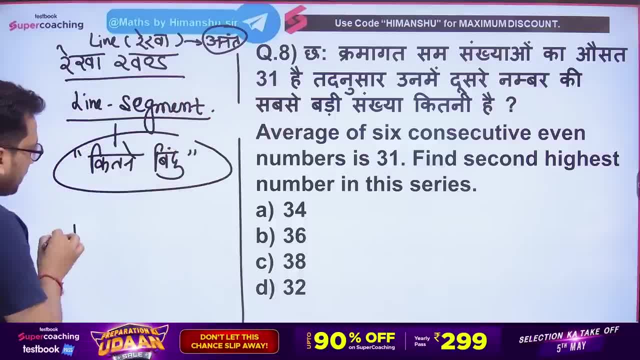 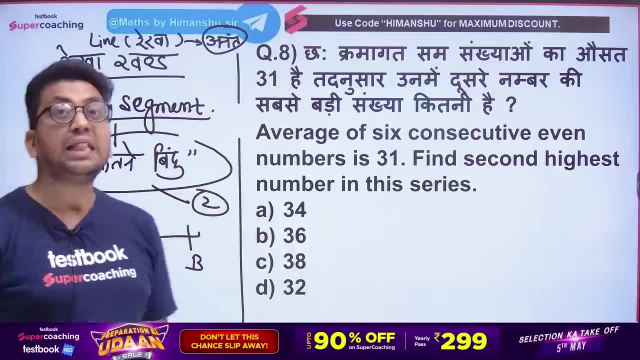 And when I talked about the line segment, then it is absolutely correct that here, son, there are two points, A and B. That is the points that will be made. here will be two points, But your answer is wrong. Why wrong? 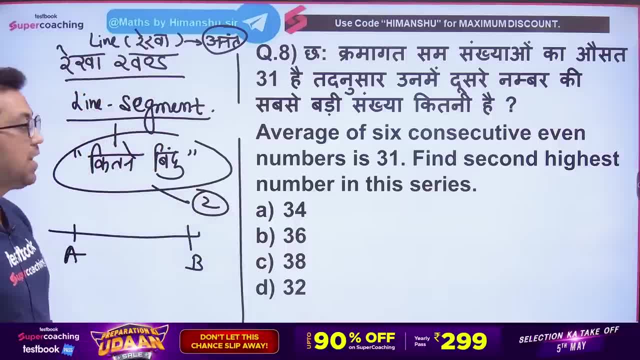 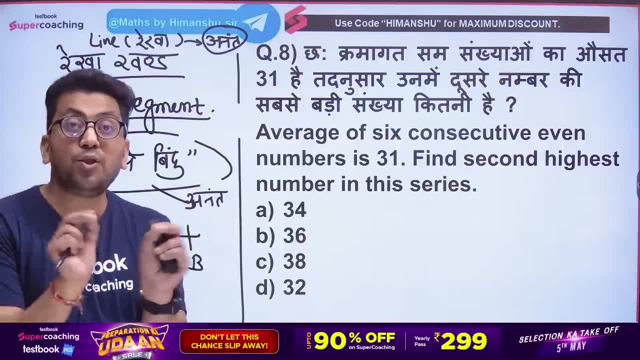 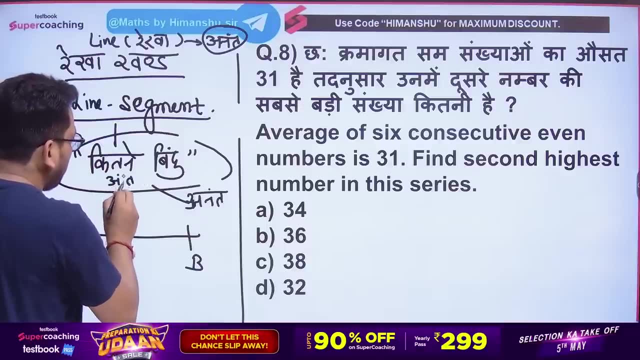 Because you did not understand the question properly, Son. there will not be two here. There will be infinite here. What will be infinite, Son? I did not say the last point. Yes, if I ask two, how many? how many last points are there? 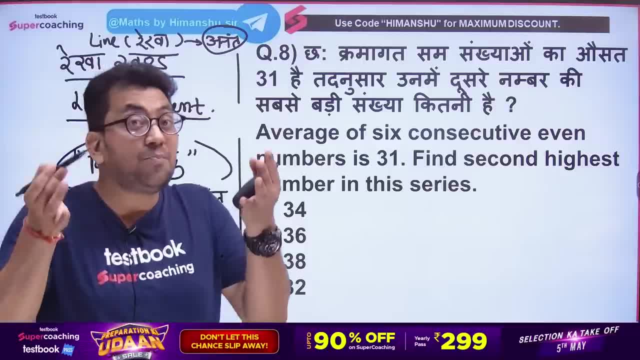 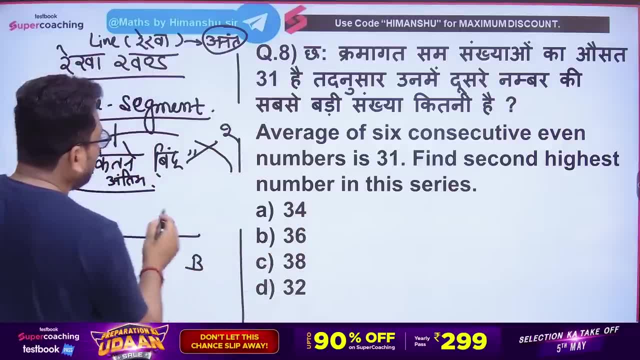 Or I can say this: How many extreme points are there, How many end points are there, How many last points are there? then its answer is two. But when I asked: how many points are there? So, son, how many points are there? 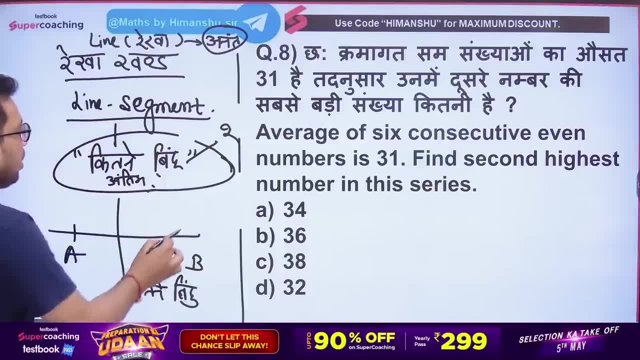 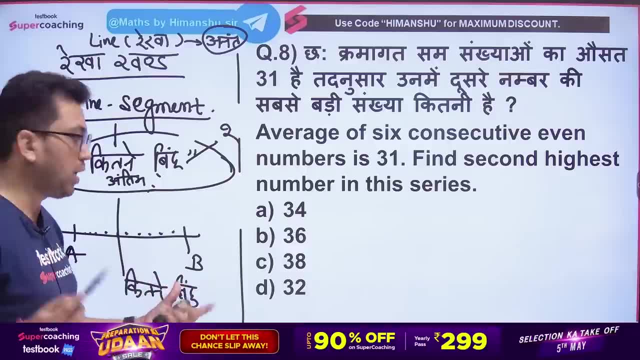 The answer will be infinite. Why will it be infinite? The line between A and B, this is a line segment. there will be infinite points on this line segment too. There will be infinite points. How many points will there be? Infinite means infinite. 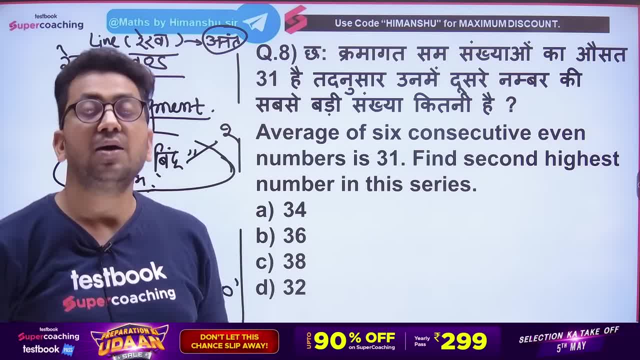 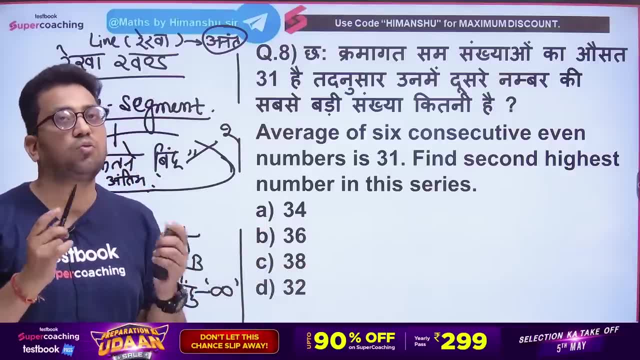 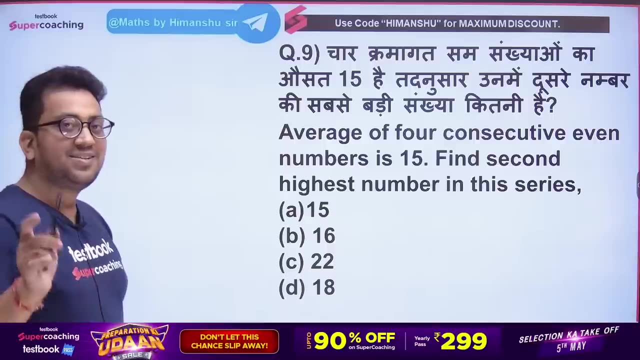 So its answer was to be infinite. Always keep this in mind. Examiner turns the question in this way: The child thinks that I did it right, but it turns out to be wrong. Always keep this in mind. This is the question. Whatever question I ask you. 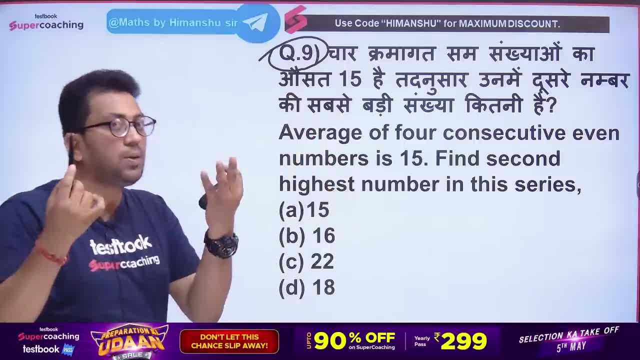 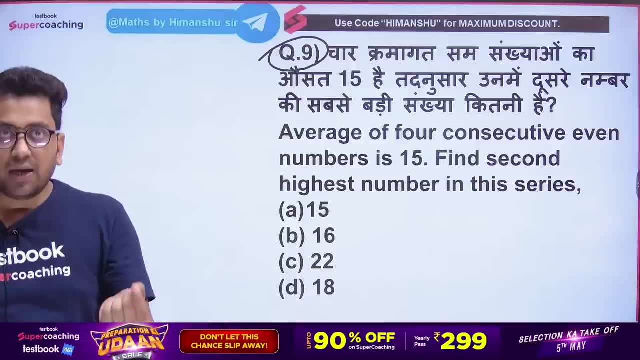 I ask it with some thought in mind, So that the concept of our children is clear. Next question: The average number of 4 round numbers is 15.. According to that, what is the largest number of the second number? Answer it quickly. 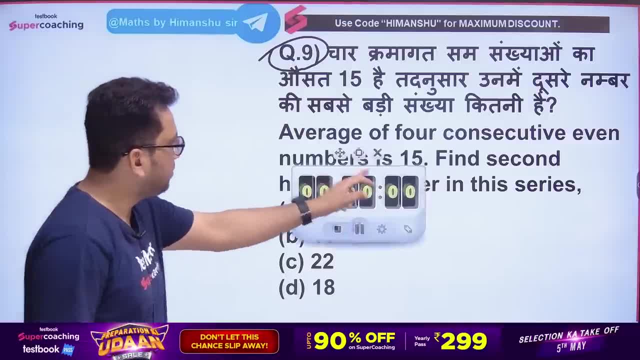 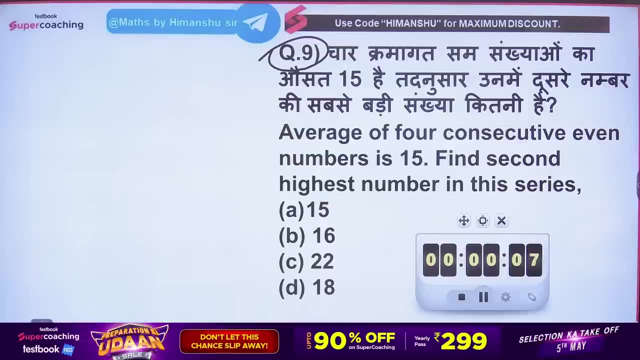 Mr Lal, Answer it. We will set a timer of 20 seconds for all of you. Tell us what will be the answer. All of them, All of them Answer it. Tell us what will be the answer. Look dear. 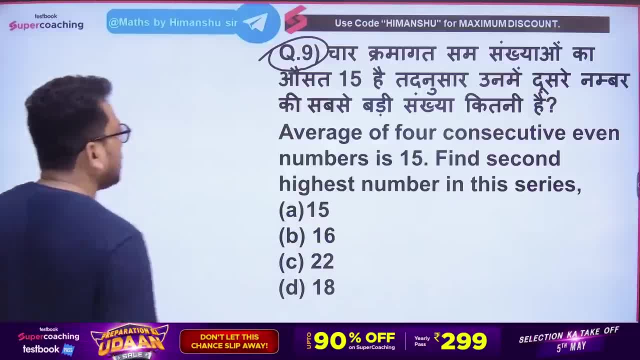 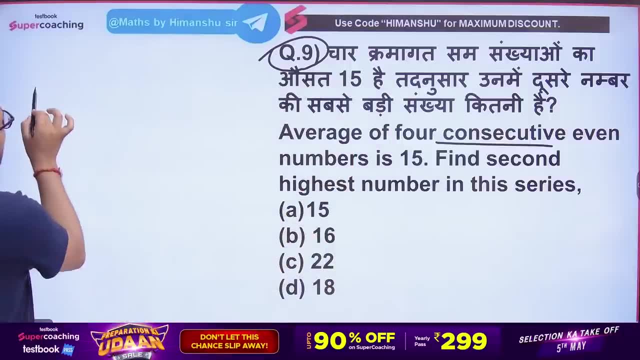 We tell you that the average number of 4 round numbers is the maximum number of 4 round numbers. That means 4 average numbers. Sir, if there are 4 average numbers, then put 4 lines: 1, 2,, 3, 4.. Very simple. 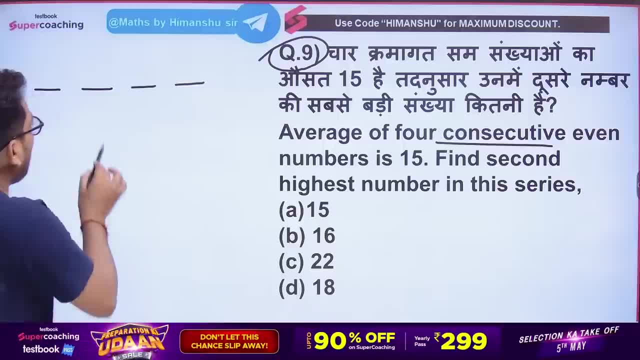 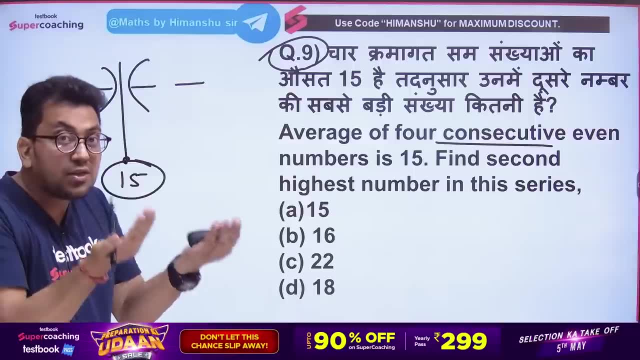 Sir, the average number of the second number is the average. That means 2 here, 2 there, Sir. the average number of the second number is 15.. It is our average, Sir. the average number of the second number is the largest number. 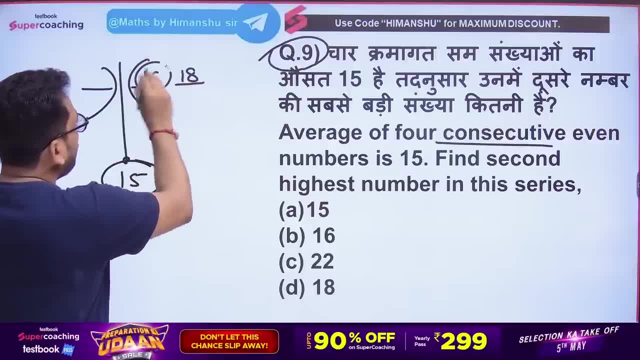 And these are the total numbers. So after 15, the total number will be 16.. And after 16, it will be 18.. But the number of the second number is 16.. So, very good, All the children are answering. 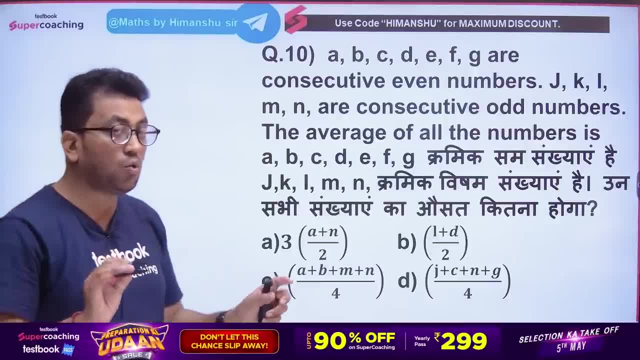 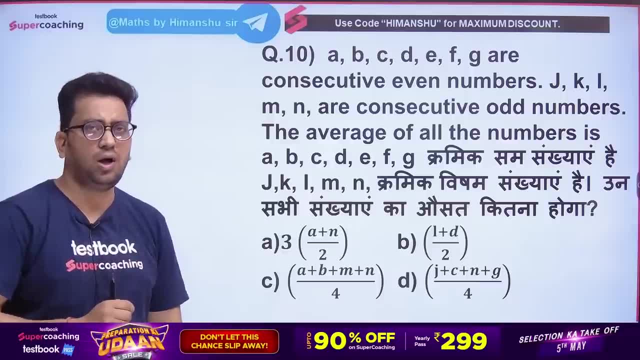 Option number B: Tell me, is there any child who is not getting it? Will it come? Have a little patience, Have patience, Have patience. If such serious questions come in your exam you will say, sir, is it halwa or halwa? 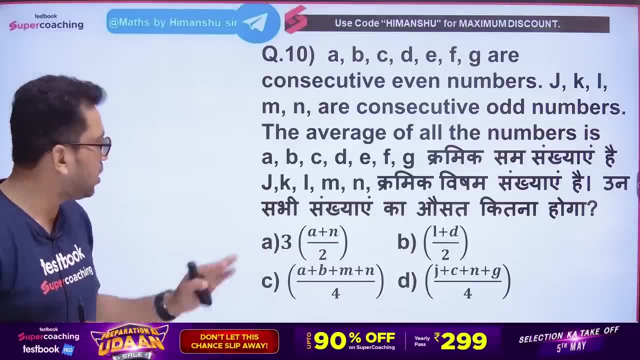 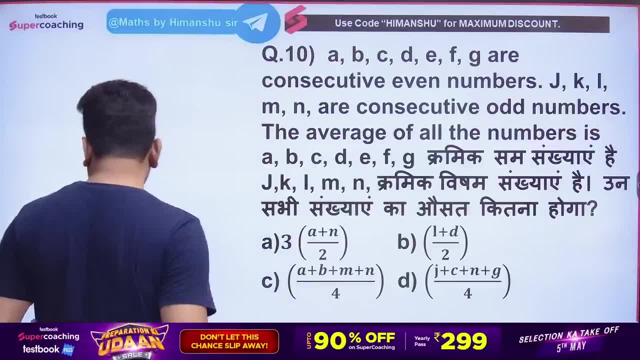 You will tell me yourself, sir. is it halwa or halwa? It is the same. A, B, C, D, E, F, G are integral numbers. What are they? They are integral numbers. J, K, L, M, N. 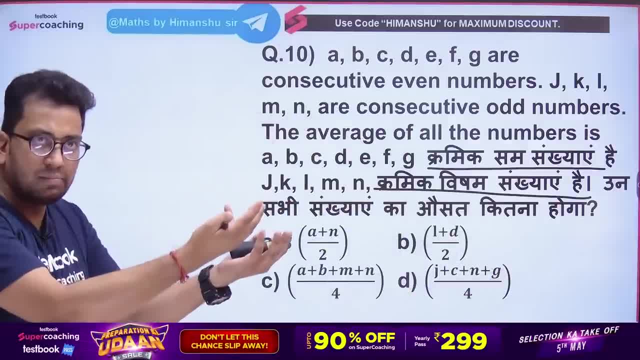 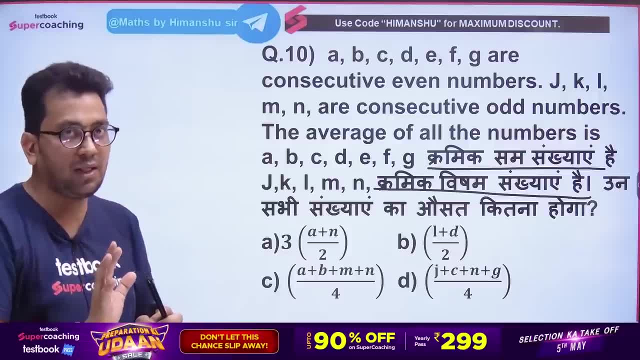 are integral numbers, They are integral numbers. These are integral numbers, But they are integral, That is, they are consecutive. That is, the concept is going to be the same. He says: what will be the ratio of all those numbers? 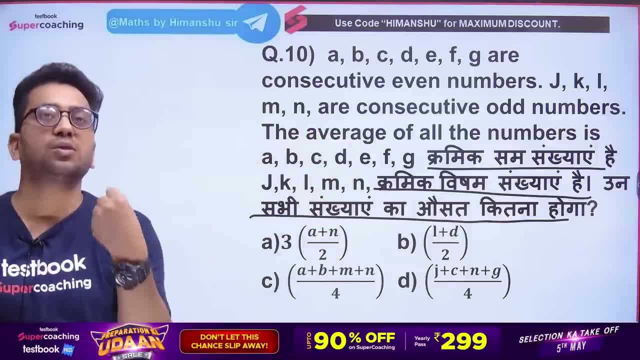 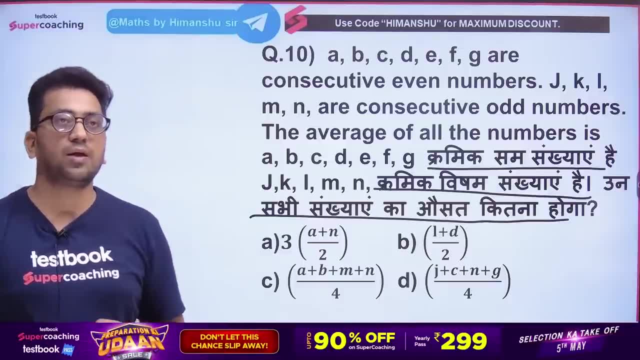 That is, if I talk about the ratio of both of them, then what will be their ratio? This is being asked to you. Okay, Try it. Let's see how many children are able to answer. Fly the question, son. Tell them that the answer will come. 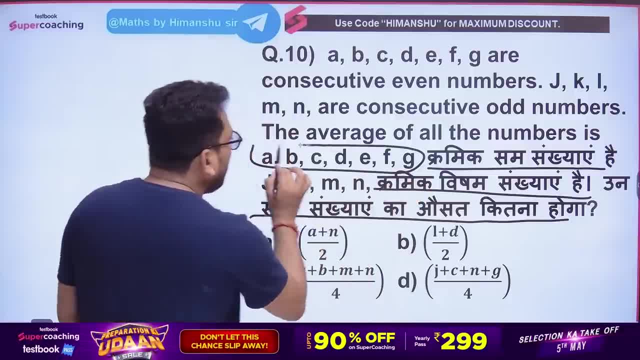 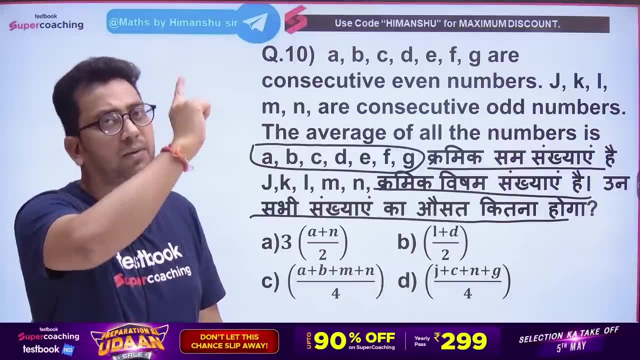 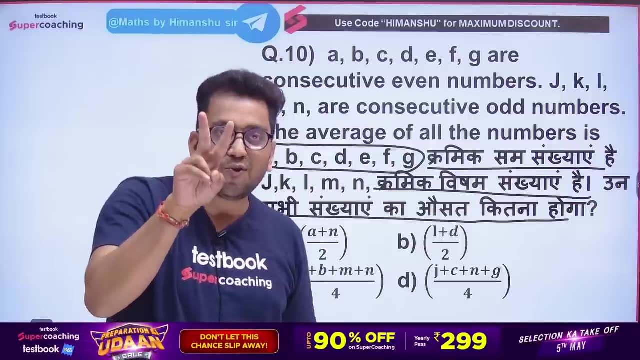 Tell me one thing: What you are seeing, these are integral numbers, So what will be the number in between them? Will it not be average? Tell me so much. What will I do? I will see its ratio, And when I get both the ratios, 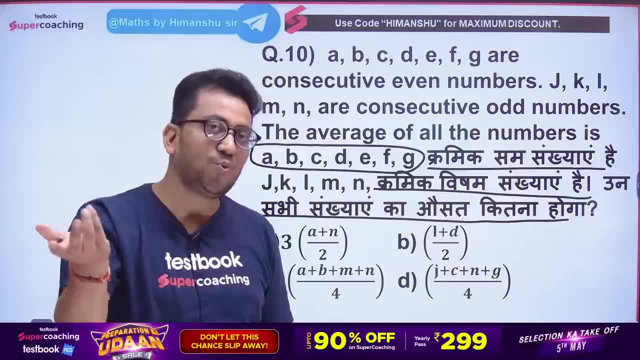 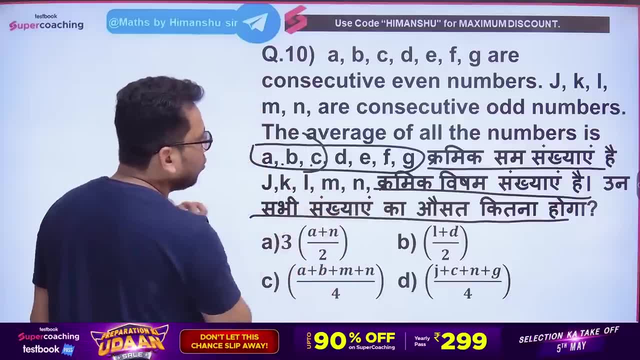 that is the two numbers. I will get their ratio. Oh yes, I will get the whole ratio. How See: 1, 2, 3, 4,, 5, 6, 7.. In 7 numbers. 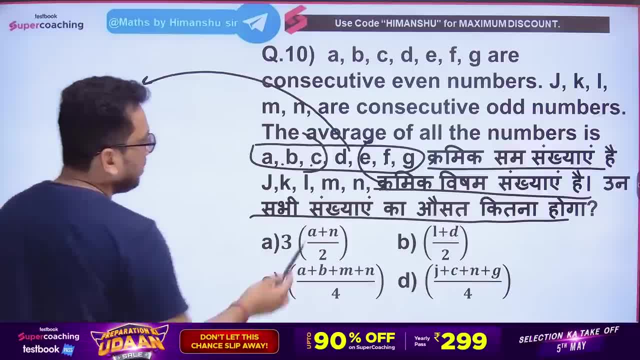 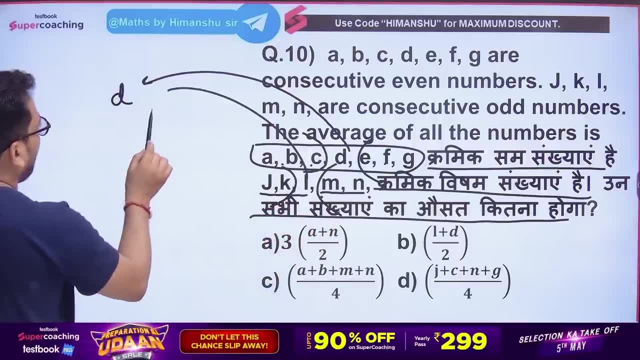 3 is next to this. 3 is next to this. its ratio is D. Let's move on here. Here, sir J K L M N are 5.. 2 is next to this. 2 is next to this. 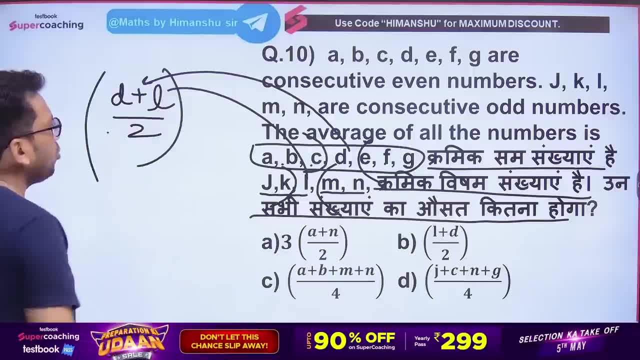 what will be my answer? Join both numbers and run away from them. See, it is your answer. Tell me how long this will take. Will you write on its Solid is our answer. L plus D by 2 or D plus L by 2 is the same thing. 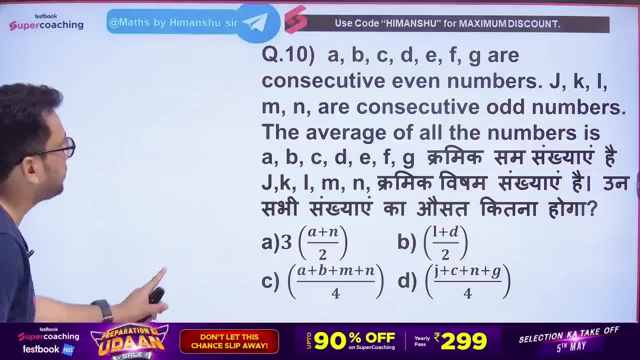 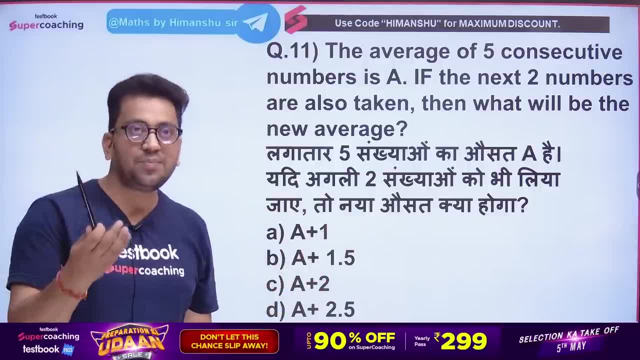 Now B is our answer, Son, do you understand the concept? Are you able to understand the filling of the questions? The next question is before you. Here it is Now here. there is a change in the concept And when we will teach you the concept. 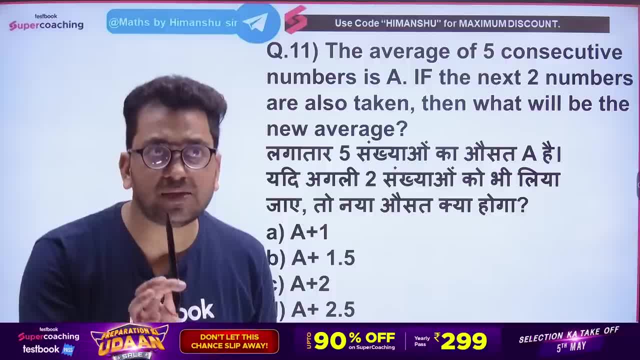 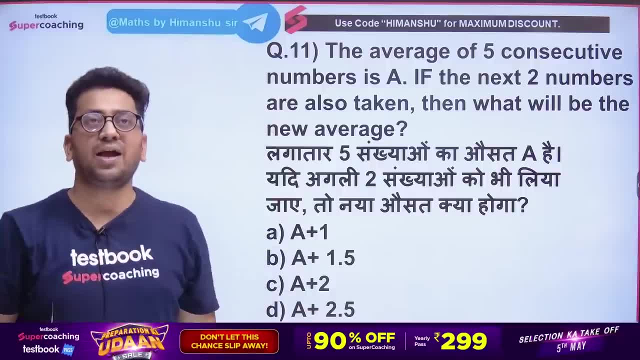 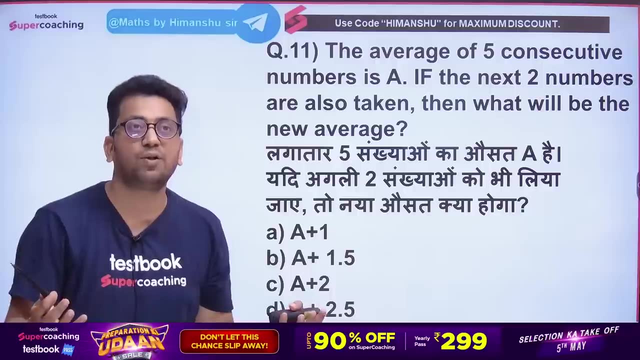 Will you all be ready to learn all the concepts? in the comment section, all the students will write together: yes, sir, it will be fun to study when the desire to study, that is, the desire to study, will develop inside you. Once all the students will write yes, sir, ready, we are ready to understand the concept. 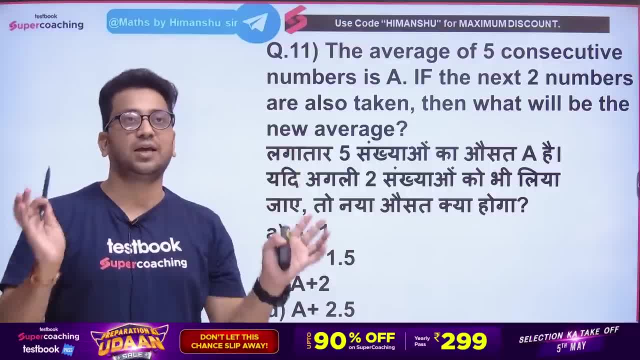 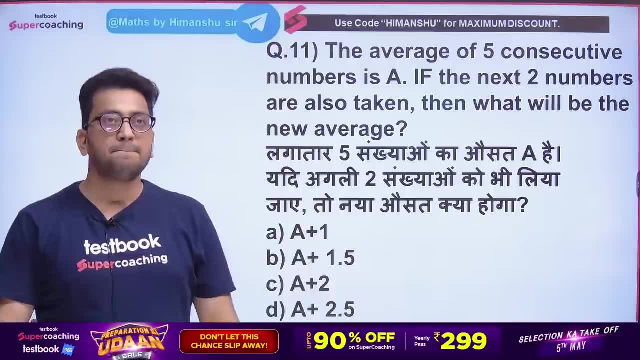 and then you tell us the way to shine, sir. then it will be fun. Are you all ready Once? yes, sir, write quickly in the comment section all of you once, with speed, Yes or no? Yes, Ready, All of you? 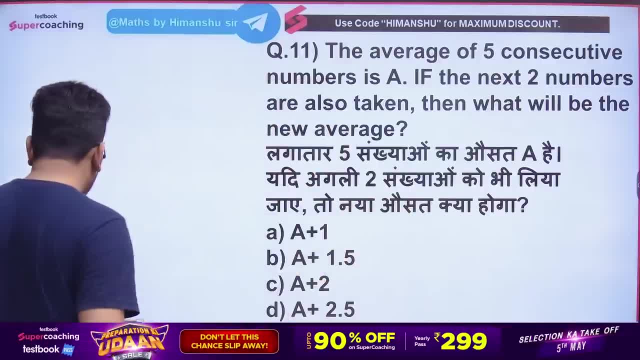 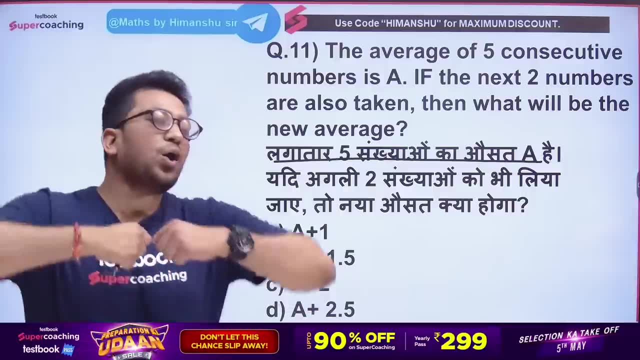 Come son, Constantly 5 numbers, listen carefully, constantly. 5 numbers have the value of A Sir. which of these 5 numbers can it be He is saying that they are continuous? I take any 5 continuous numbers. 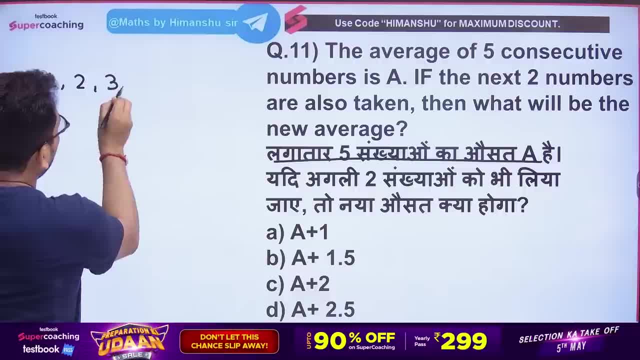 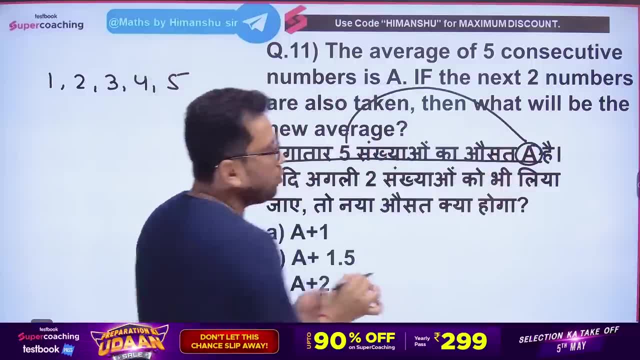 Suppose I took 1,, 2,, 3,, 4, 5.. Did you take? Did you take? Okay, He is saying that their value is A. What is this saying? What is their value? A is Tell me what will be the value of them. 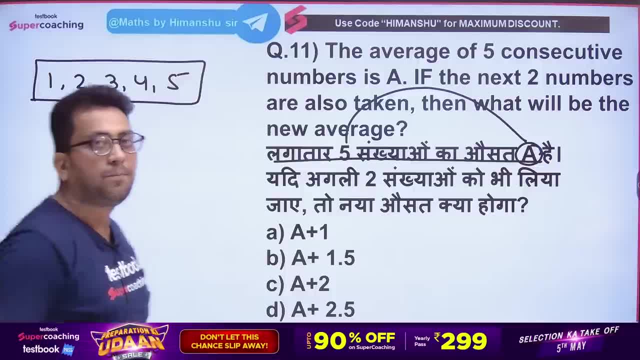 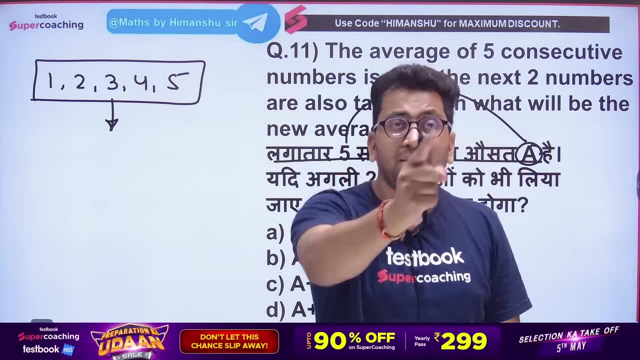 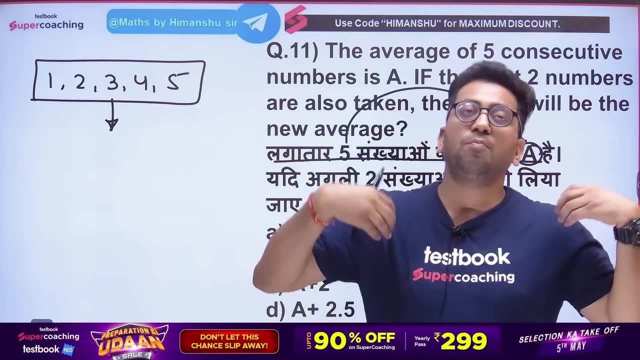 All the children in the comment section. I took these natural. whatever I have taken these continuous numbers, there are 5 continuous numbers. tell me what will be their value? The comment section should be filled. If you understood. if you gave the wrong answer, then my teaching is absolutely useless. 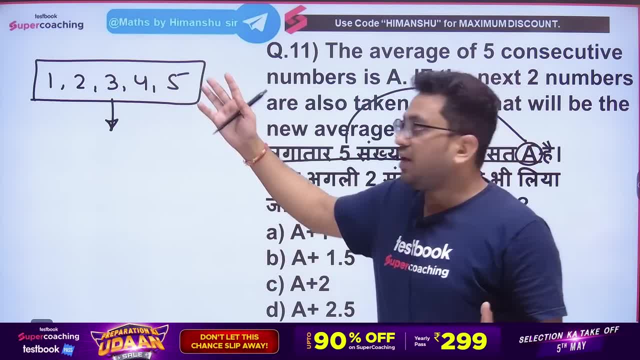 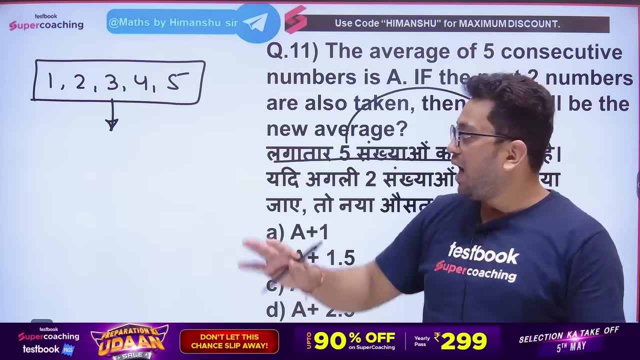 Absolutely useless. I want its answer. tell me, Fine, what will be their value? What will happen? What will happen? Don't give the answer of 2a plus 2a plus now. don't worry, just give the answer of what I am asking now. 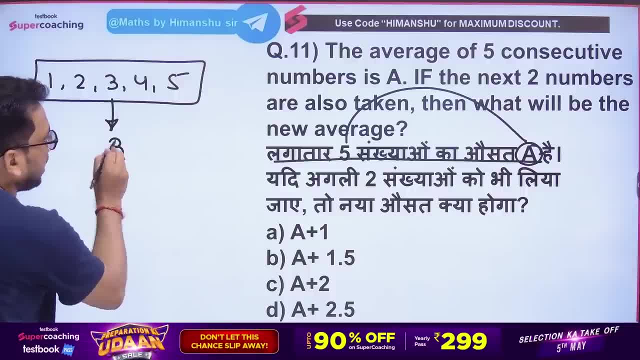 What will come? 3 will come. Very good, Sir. 3 will come. 3 will come. He said it is a. So what did we consider this a, as We considered it as 3.. Are you able to understand? 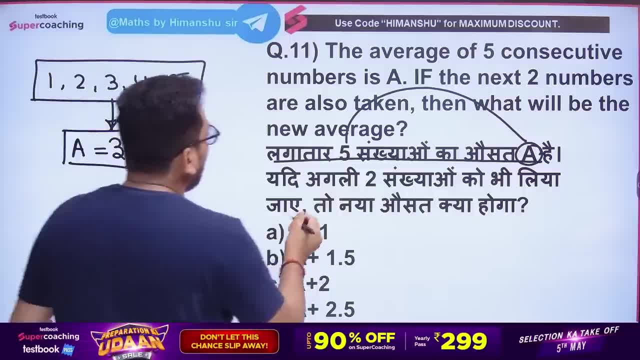 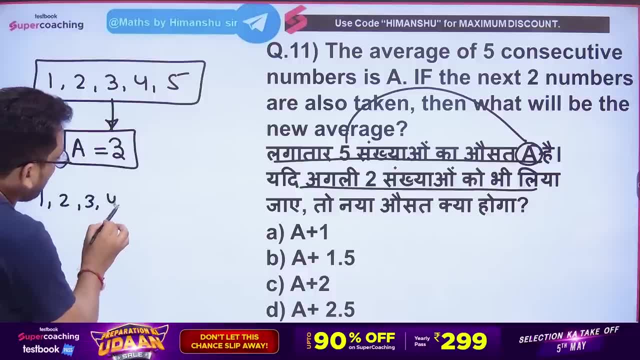 I am teaching the concept and then I will tell you the way to shine. Look ahead. It is said that the next two numbers were also taken. Now, the next two numbers of it were taken: 1, 2, 3, 4, 5, 6, 7.. 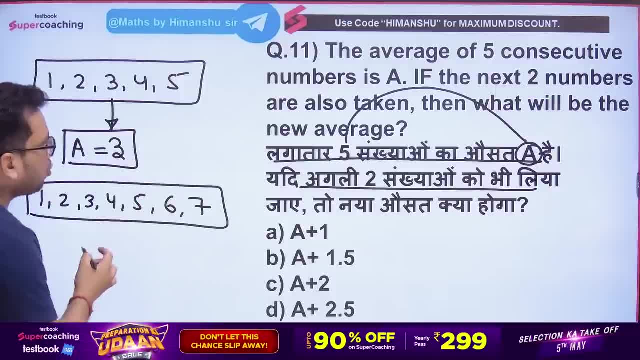 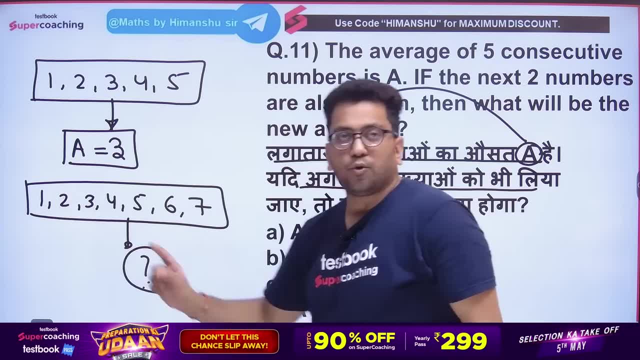 Take the next two numbers more. Now you people tell me what will happen to it. Tell me quickly what will happen to it. I want its value, which you can see. It is a circular number And the middle number in the circular is that value, you know. 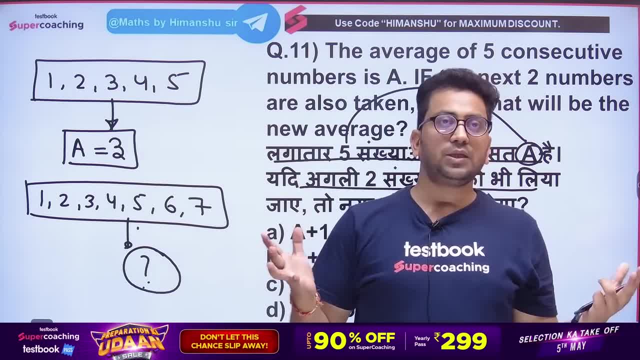 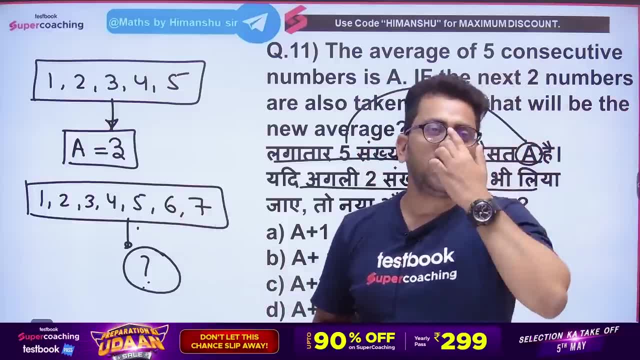 Tell me quickly what will happen to it. Tell me quickly, Make my heart happy. Tell me quickly what will be the value of this circle With the back, All of them. So you will say that, sir, 1,, 2,, 3,, 4,, 5,, 6,, 7 are there. 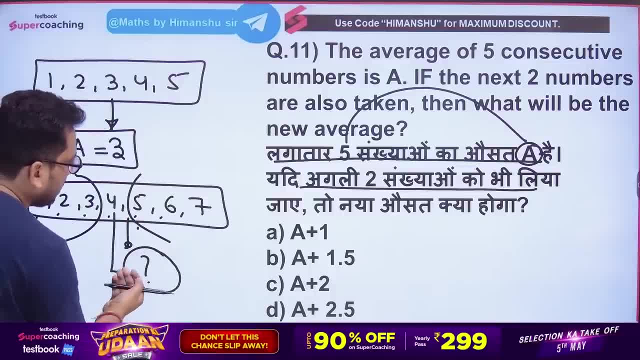 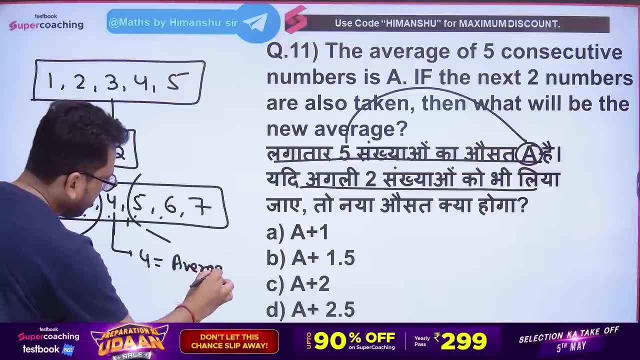 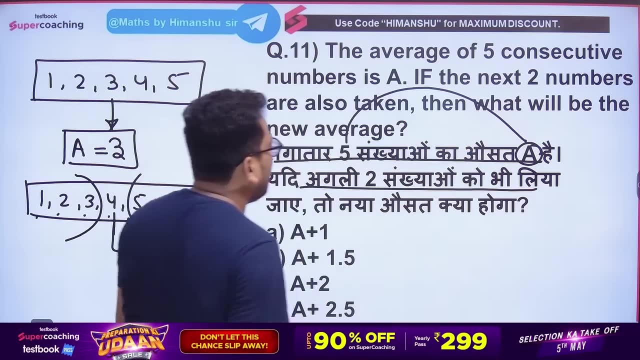 So 3 to this side, 3 to this side. Sir, this 4 is our value. This 4 is our value. 4 is the average. Okay, brother, 4 is the average. It means that he was telling us that if the next two numbers were taken, then what would be the new value? 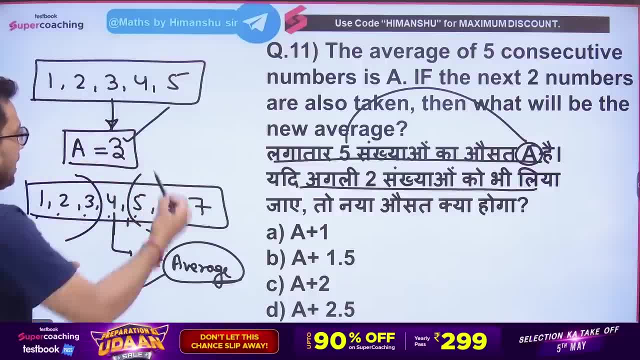 Look at this: Earlier the value was 3.. Now the value is 4.. That is, how much is added to 3?? 1 is added, 1 is added to 3.. So can I call 4 as a plus 1?? 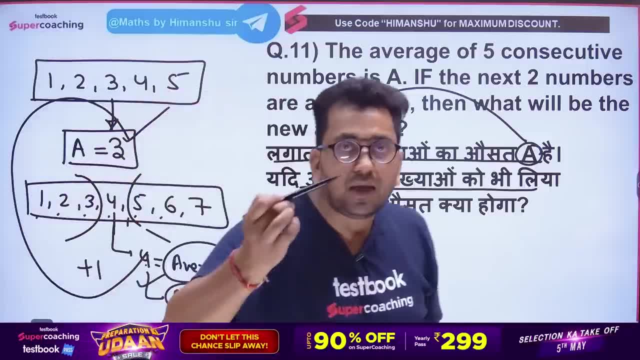 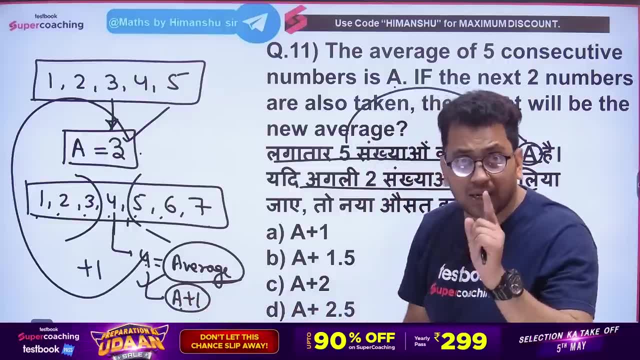 Yes, sir, I can say That is the first value was a. Now I have that value: 3 and 1.. That is 4.. That is a plus 1 came. Say yes, 3 and 1 is 4.. 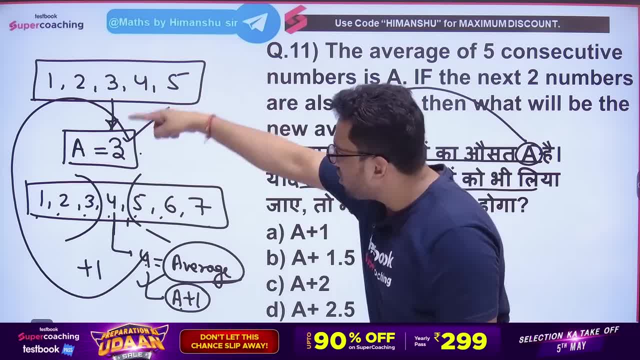 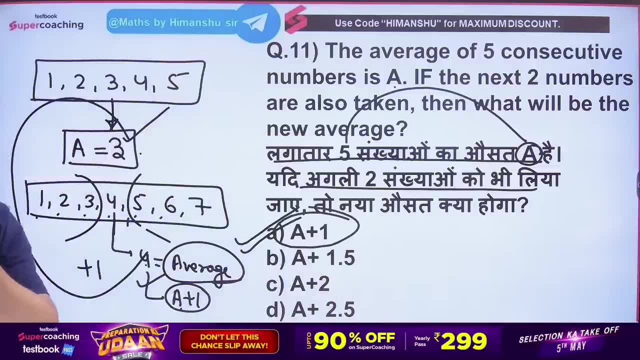 So here a plus 1 happened. That is, the first value was added to it. That is the answer we will get. here is a plus 1.. This is the point of this question. This is the whole concept. Now let's come to the way to shine. 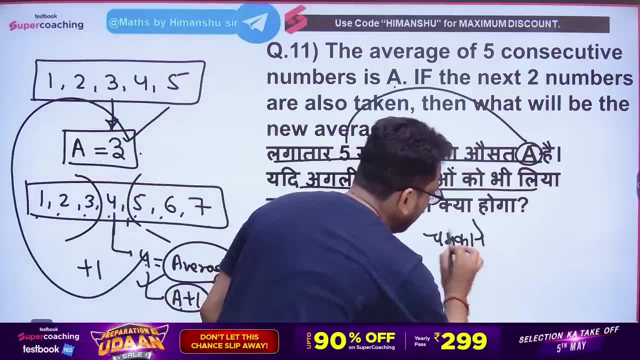 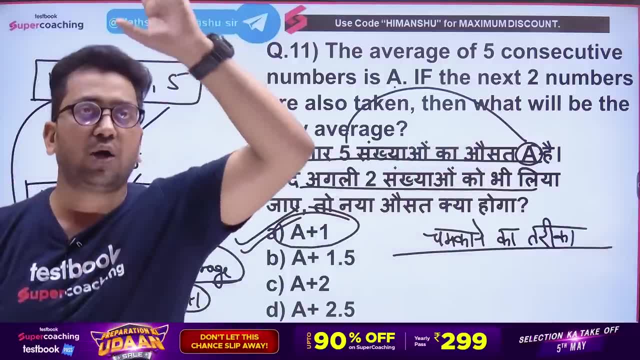 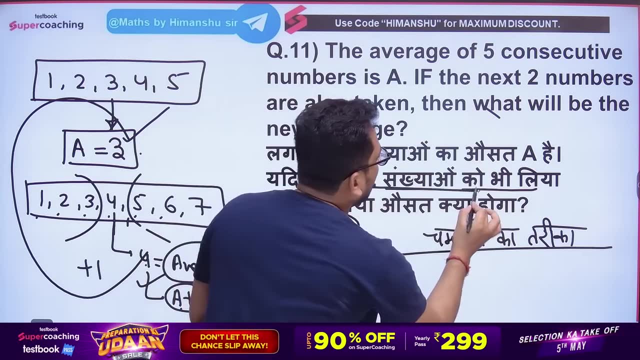 How will everyone shine in the exam? The way to shine. This is very important, son, Because if this comes, then your way of playing in the exam will be different from others. So see what is the way to shine. Our child will only see that. how many next two numbers, how many next two numbers are being added. 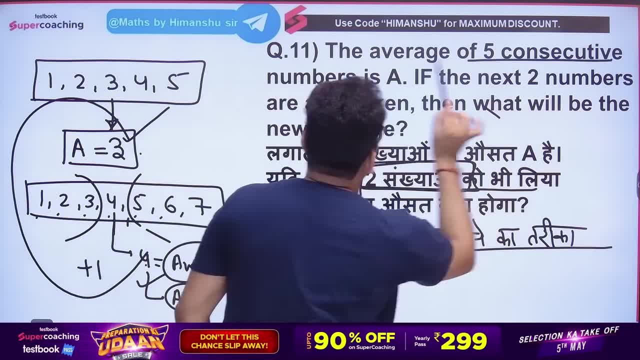 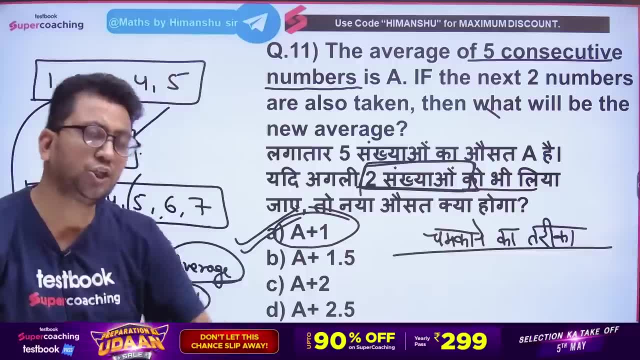 So don't pay attention, These are consecutive numbers. These are consecutive numbers. So in that you will see how many next numbers are being added. All the numbers that are being added, divide them by 2. And, whatever will come, add it to the first value. 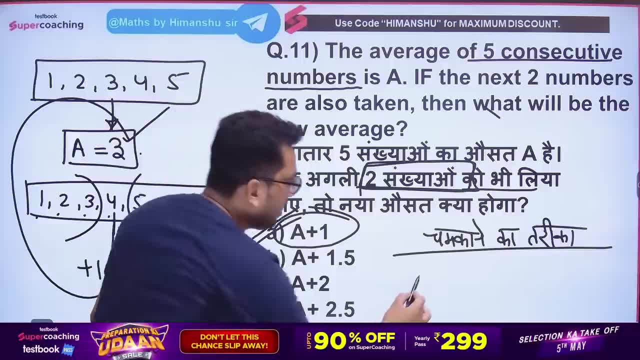 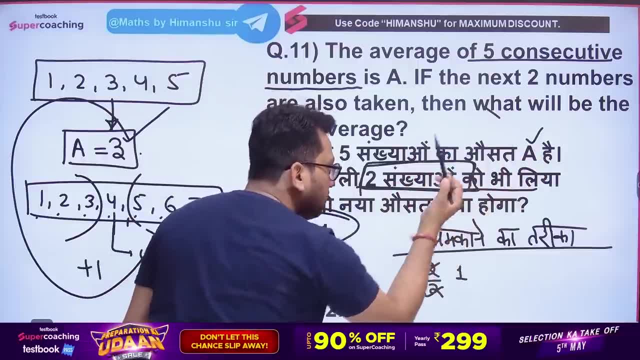 What does it mean to say? If the next two numbers were being added, then you will divide 2 by 2.. How much did it come? 1 came And the first value that will happen. you have to add it to that value. 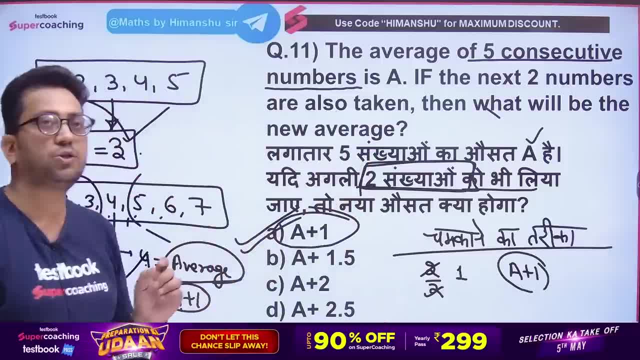 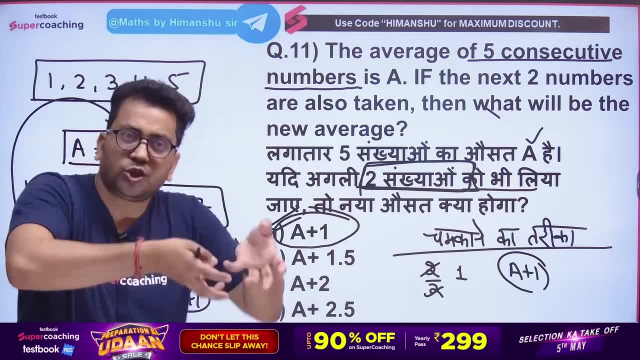 That is our answer, is a plus 1.. Can you understand my words In this way? See, if the next 5 numbers were being added, then I would have divided 6 by 2.. If 5 were being added, I would have divided 5 by 2.. 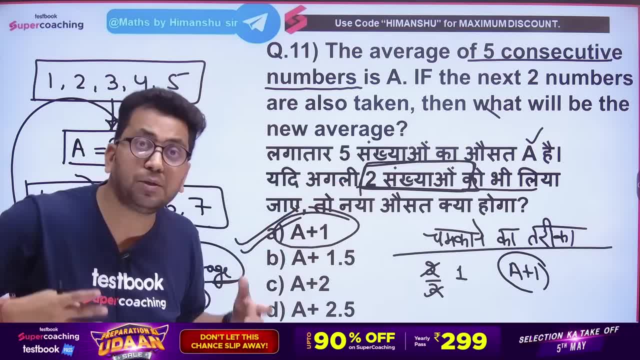 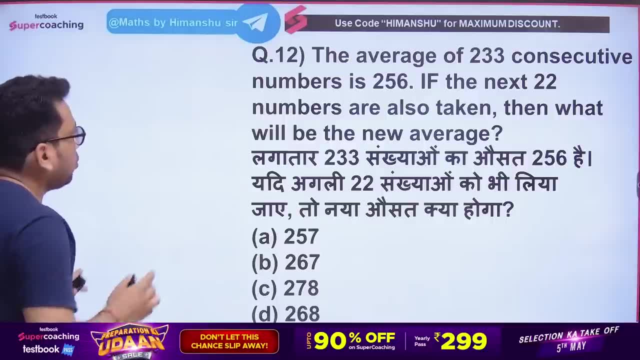 If 2 came, I would have added 2.5 in the middle. That is the answer is a plus 2.5.. Tell me if you understand the concept, then give me the answer to this question Now see, these are the questions. 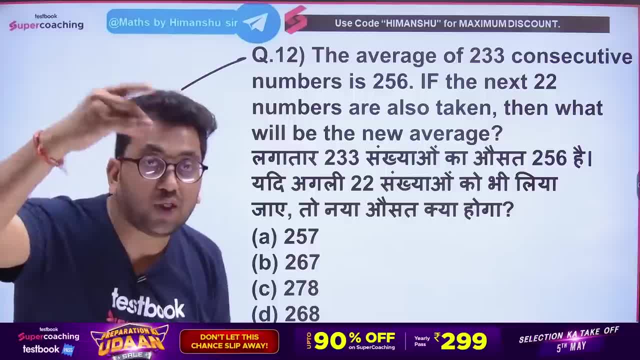 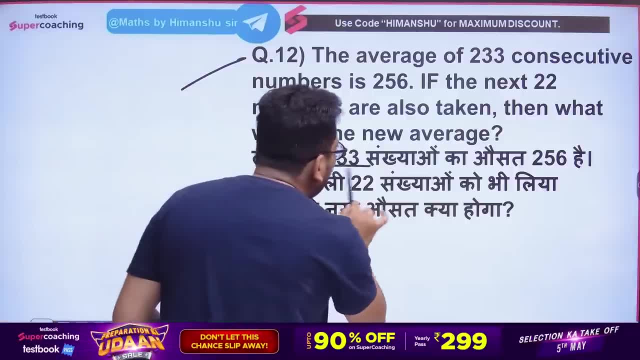 Now my child will smoke these questions. Smoke, smoke, Hey, it will shine by looking. It will shine without a pen and paper. He will say that the average of 233 numbers is constantly 256.. Pay attention to the average. What is the average? 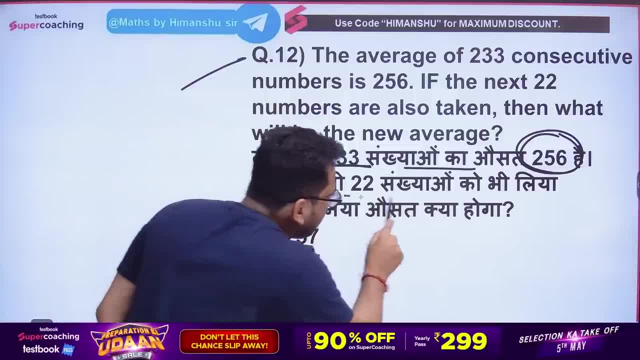 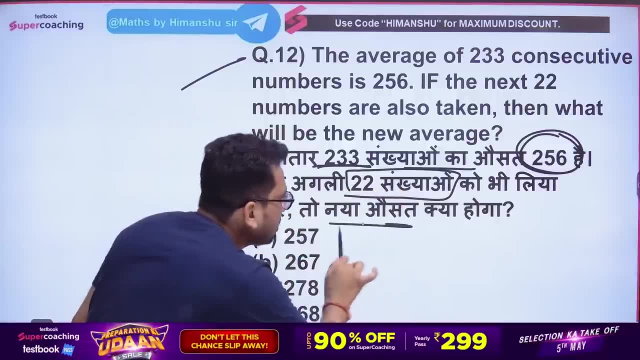 256.. Okay, If the next 22 numbers are also taken- how many numbers were taken? 22 numbers- Then the new average is asking. Our child will shine. What will he say? He will say: sir, tell me how many numbers were added. 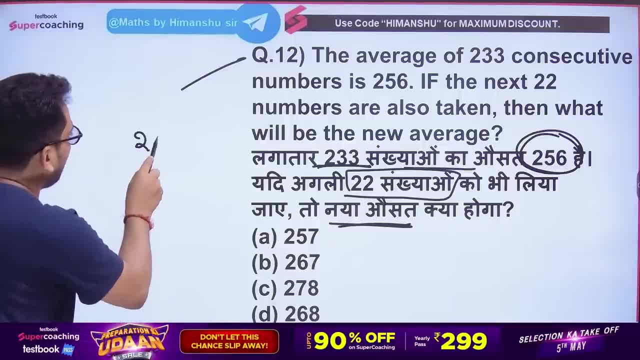 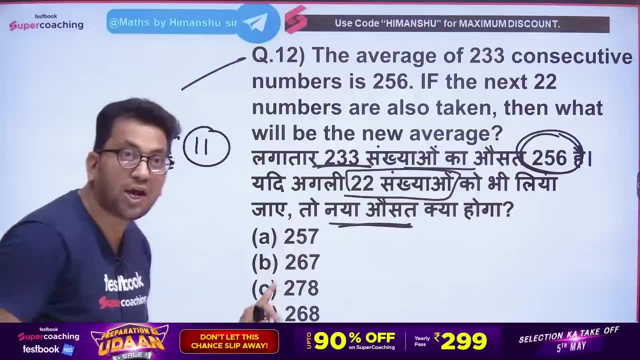 22 numbers were added, Then he will just do half of 22.. How much is half of 22? 11.. And by raising 11, in which will it be added In the old average? Then a new average will come. 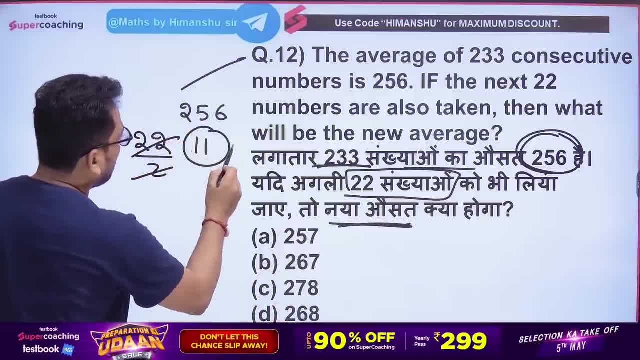 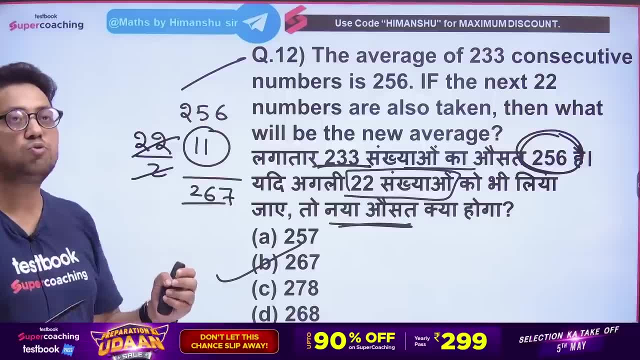 That is, it will be added in 256.. What are they understanding? 6 and 1 is 7.. 5 and 1 is 6. 266.. This is ours. Tell me how long will it take to shine this question? 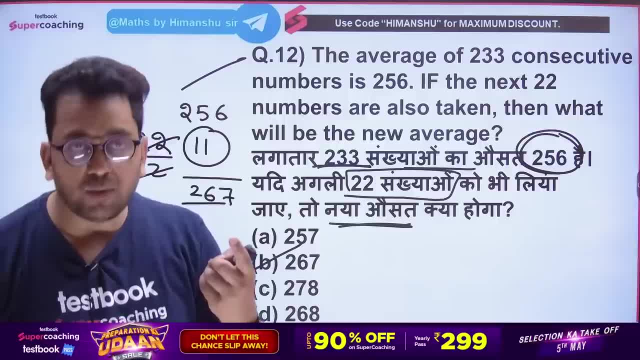 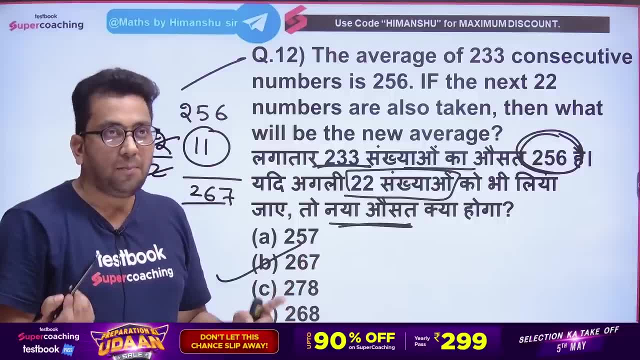 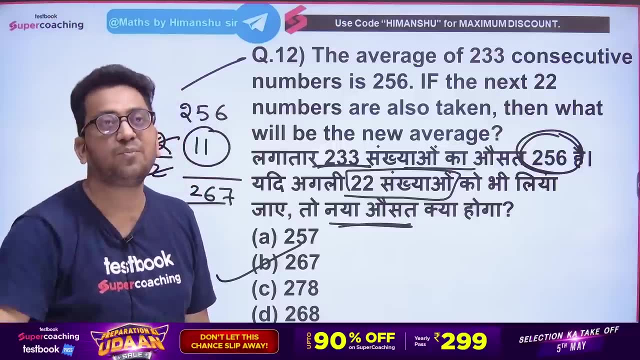 It will take no time at all. Can you understand what I am saying? It's fun, isn't it? If you want to know the answer, then click on the like button. from the heart once, I always say that this is the content that you will only get in the class of Himanshu, Sir, and not anywhere else. 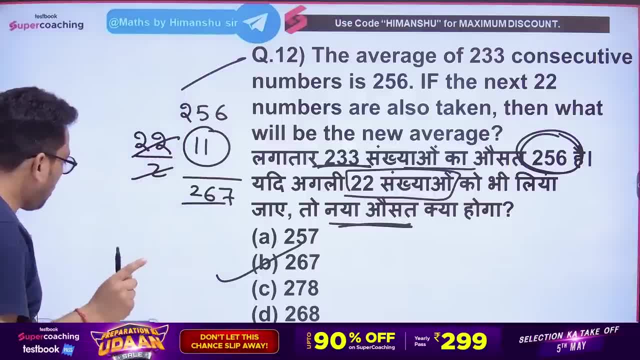 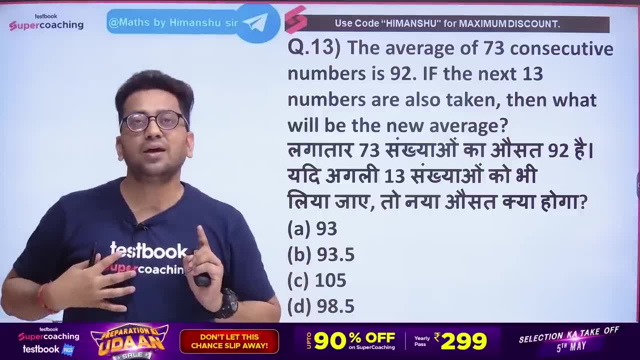 Like all of them from the heart once, And if you are studying math, then there should be only one name in your heart and mind: That I am studying math from Himanshu Sir That I know so well that wherever my child studies I have no problem. 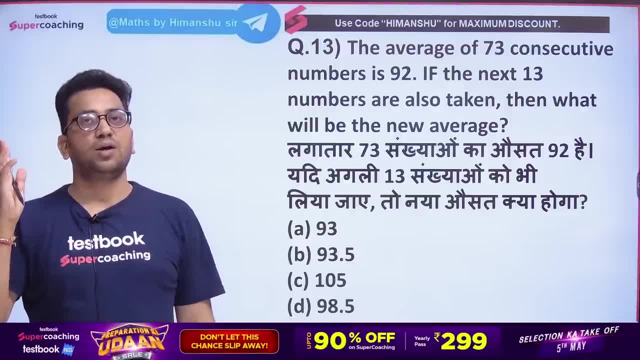 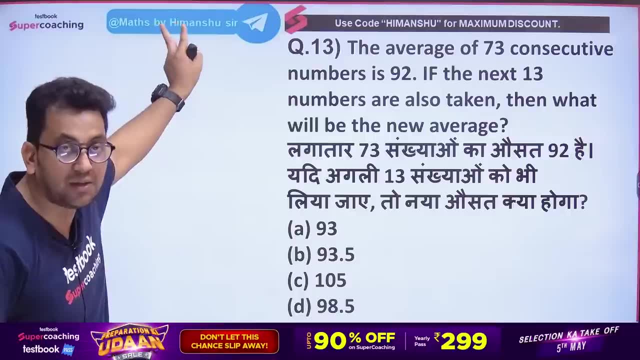 But if he studies from me, I will make him love math, I will make him select it. Then only one name: Math by Himanshu. Sir, The child who is not yet connected to this telegram channel, come and join. Next question, son. 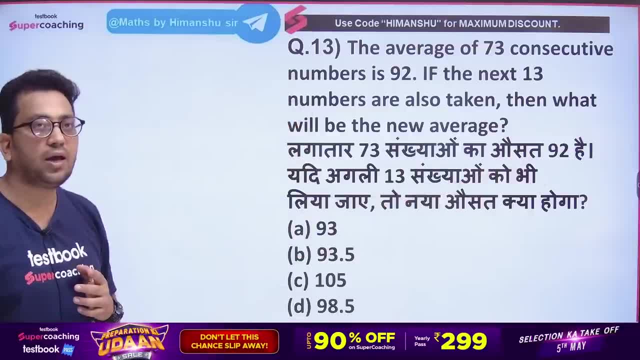 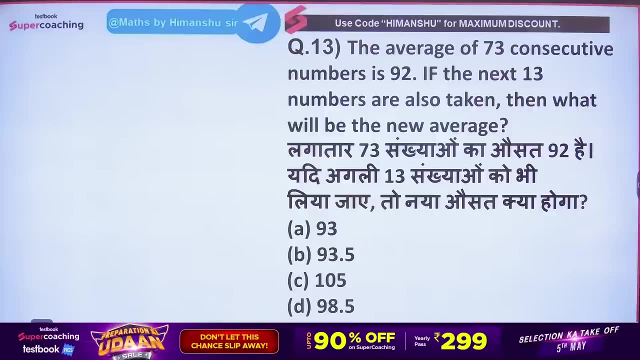 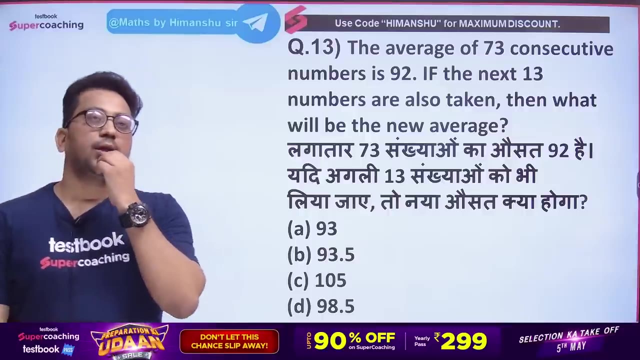 The average of 73 numbers is constantly 92. If the next 13 numbers are also taken, then what will be the new average? This is being asked to you. Shine it quickly. Tell me what the answer will be. Look very good. 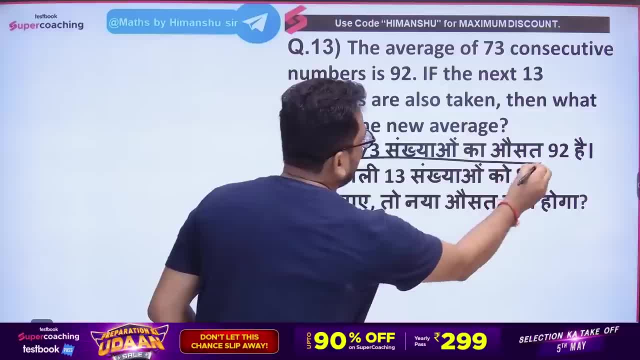 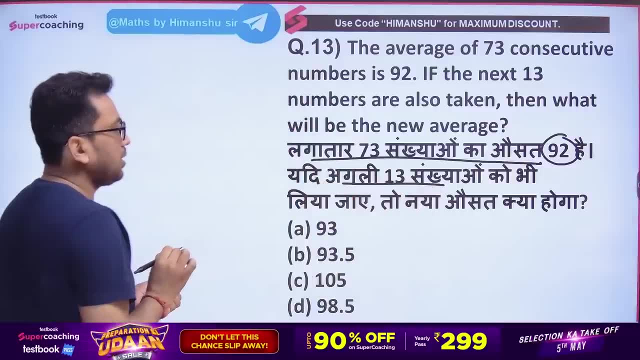 My child will say that, sir, these were 73 numbers continuously. Okay, How much was their average? It was 92.. Okay, How many numbers were added next, Sir? 13 numbers. So what will be the new average? Son, pick up 13.. 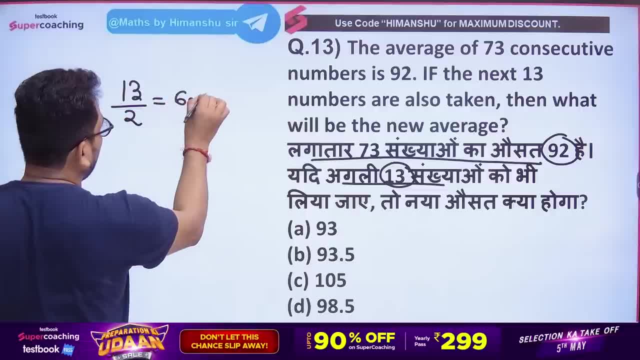 Pick up 13.. Divide it by 2. This is 6.5.. This is 6.5.. And take 6.5 and add it to this average. That is, if I add 6.5 to 92,, then how much will I get? 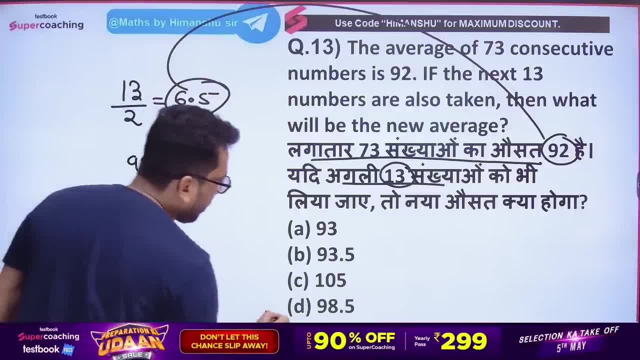 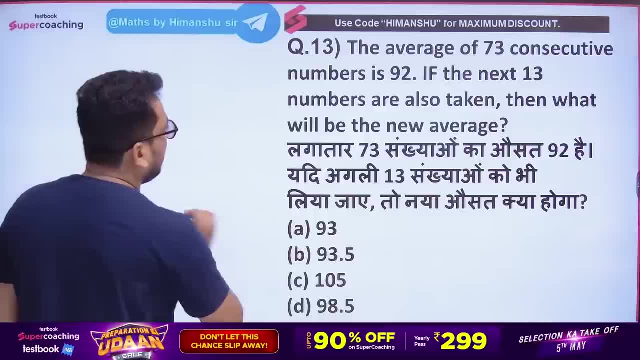 98.5.. That is, our average is 98.5.. Shine it. Are you enjoying it? D is our answer. I think every child will be able to answer my D. The next question, question number 14, is in front of you. 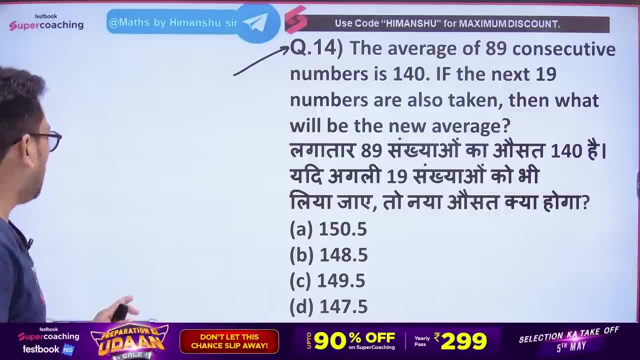 Answer it. Join me at 2.15, 2.15.. I will bring you a great session on this channel: Practice session session. Practice sessions will be there. Mixed questions will be there At 2.15.. Okay. 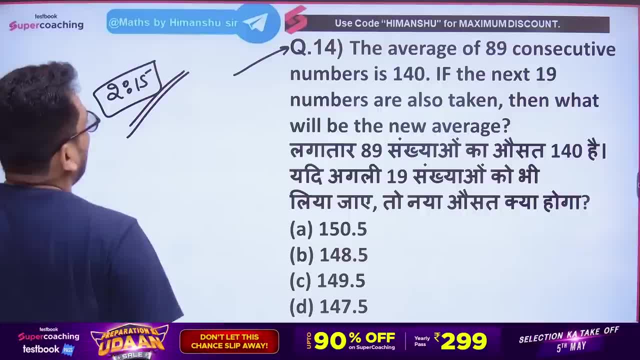 Let's go. It is continuously saying that the average of 89 numbers is 140.. If the next 19 numbers are also taken, then what will be the new average? Blow, Okay, I am understanding. So what will we do? 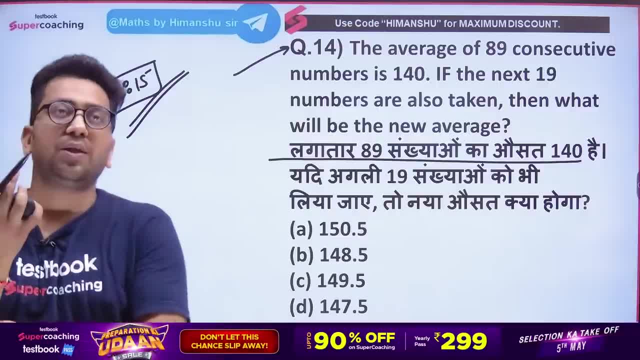 Sir, how many are there? 19 numbers. So what will we do? We will do half of 19.. How much will come? Sir 9.5 will come. Sir 9.5 will come. Sir 9.5 will come. 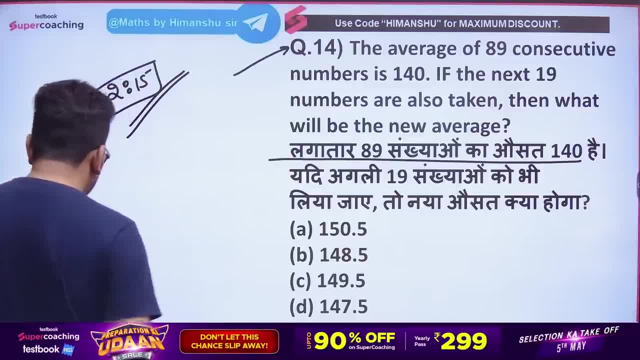 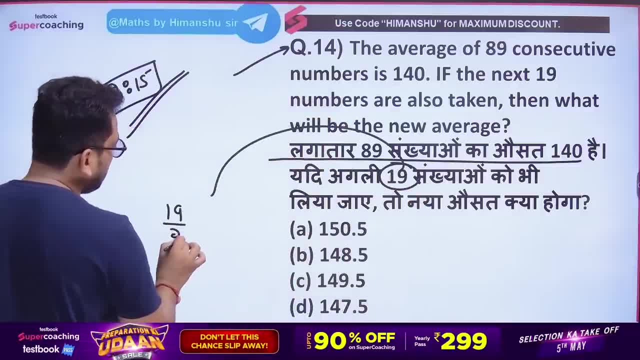 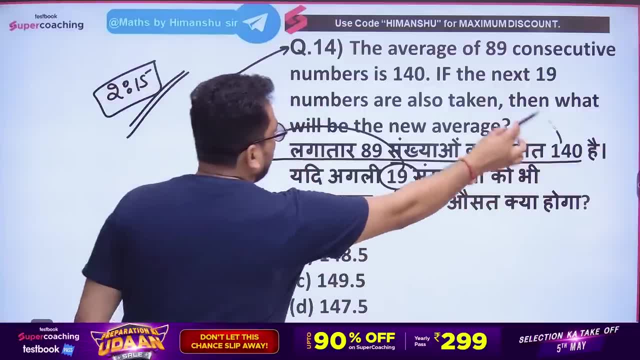 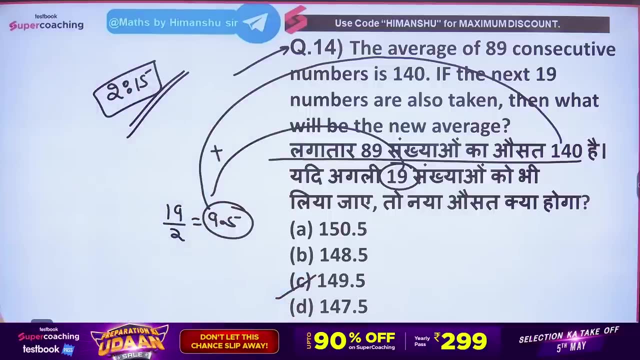 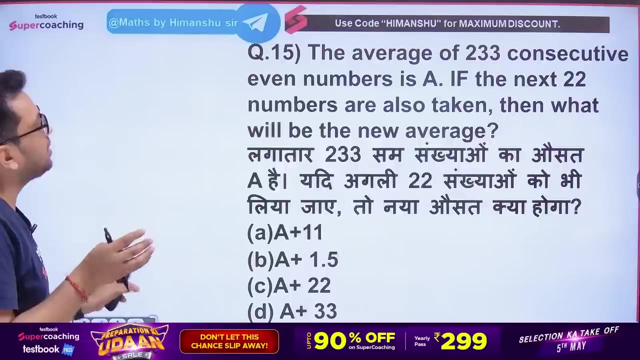 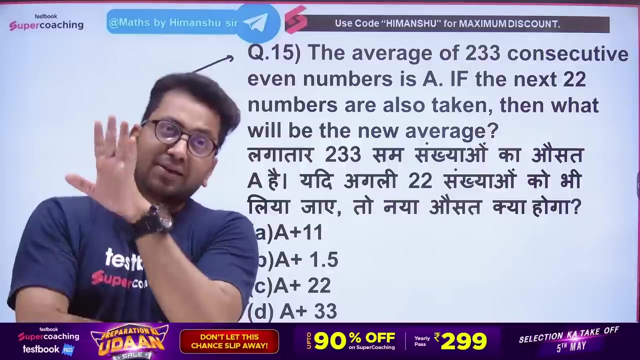 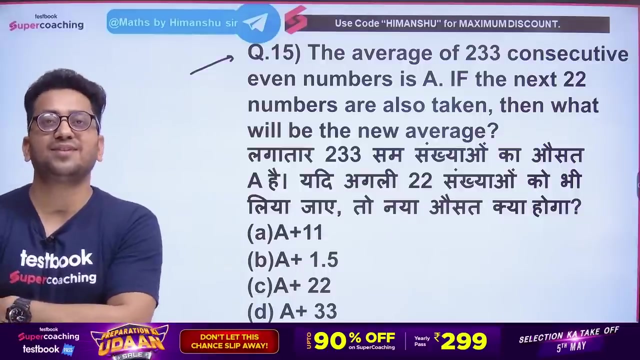 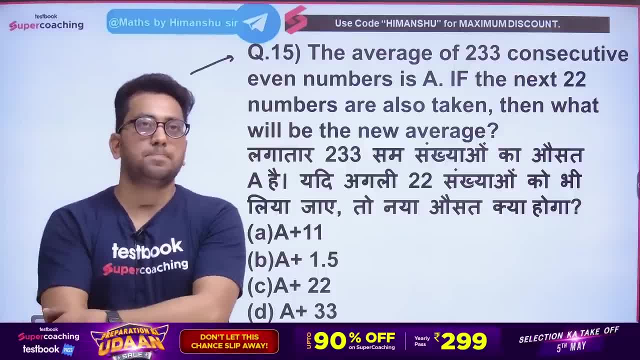 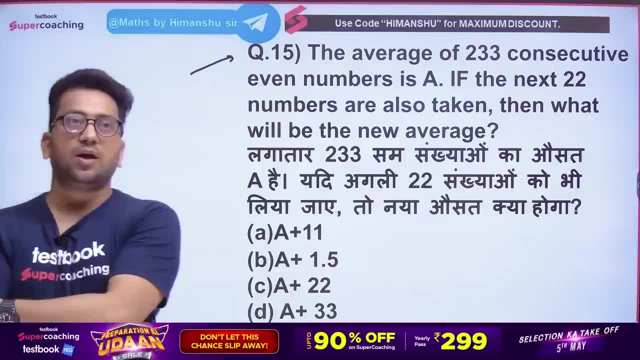 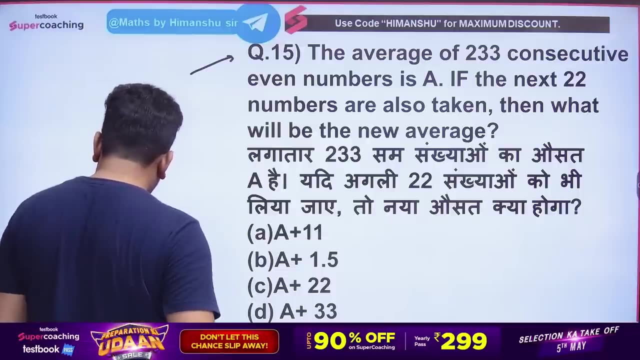 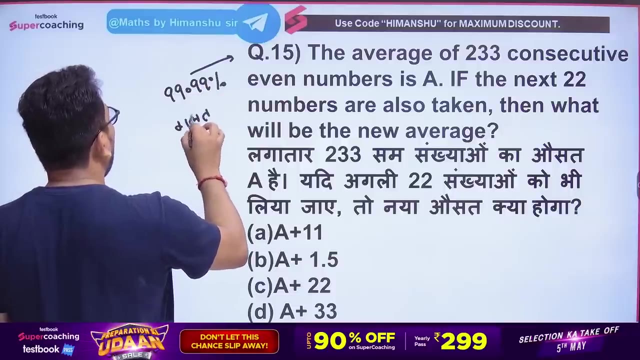 What will it be? A plus 11, A plus 11,. option number A is going towards very good, very wonderful, amazing. see the answer to this question: 99.99% of children give wrong. you will say that, sir, those who have not studied will give wrong. 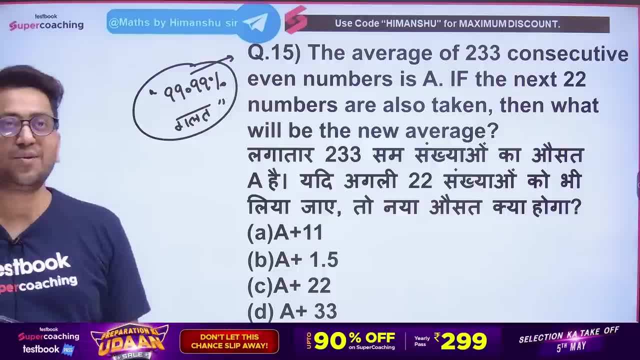 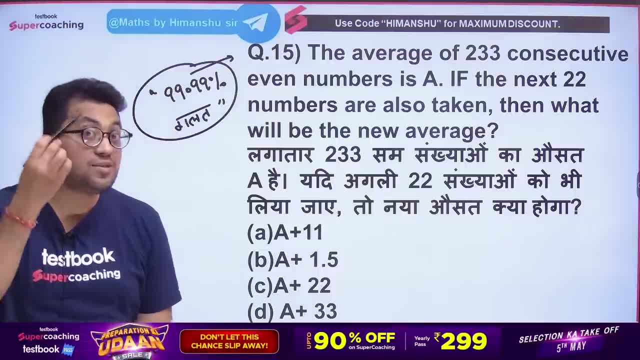 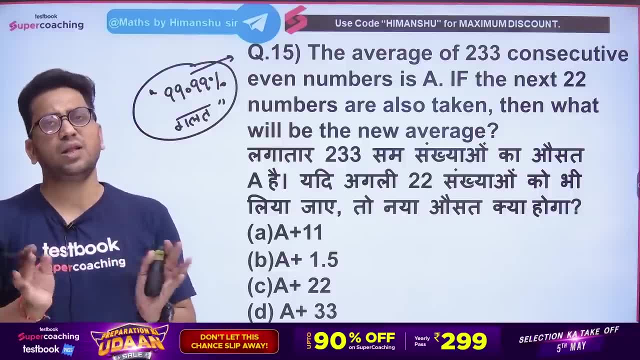 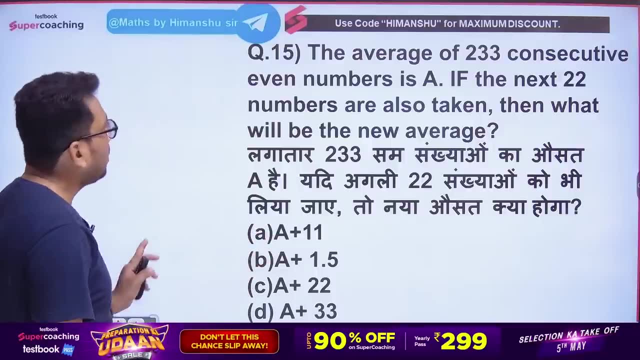 Why One is different from studying. there is a difference in studying from meditation. so the one who studied from meditation will not do wrong, will not answer, but will not do wrong. understand, Understand. The children who are doing this answer are wrong. Why is it wrong, sir? Understand Here when I am explaining you the question. then see what I am saying. consecutive numbers. 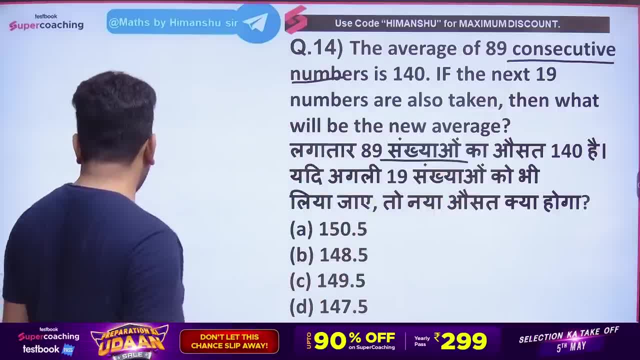 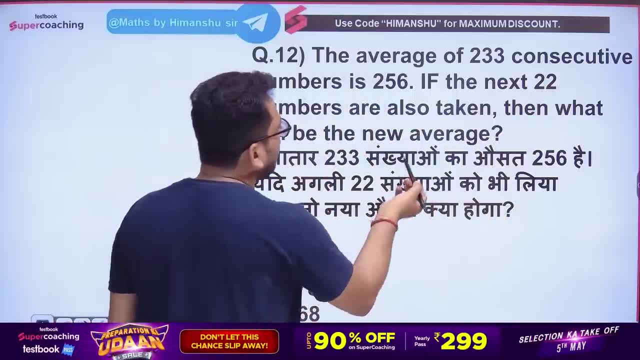 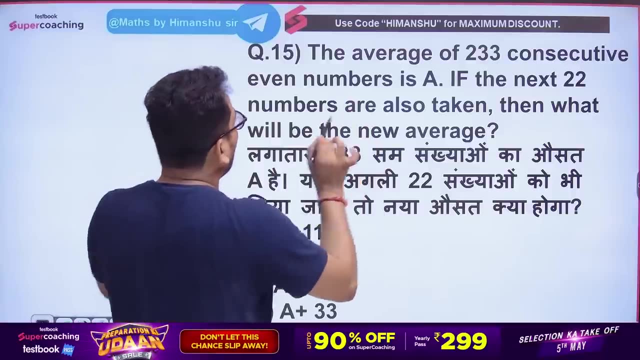 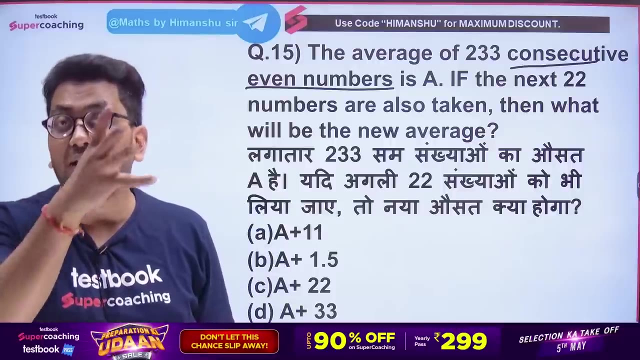 233 consecutive numbers. 233 consecutive numbers are constantly 233 numbers, but here the question is a change. here the question is saying consecutive number, not consecutive even number. that is, the consecutive sum numbers are consecutive numbers, Mr Lal, these are not just consecutive. 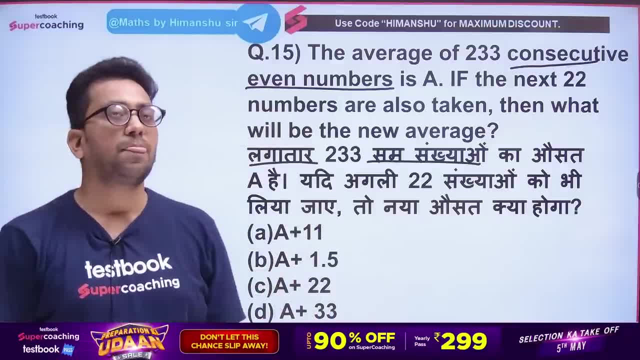 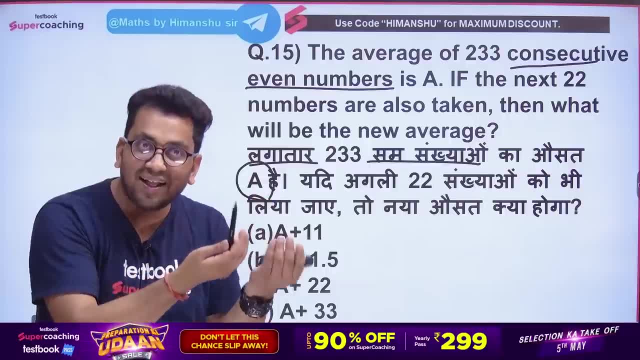 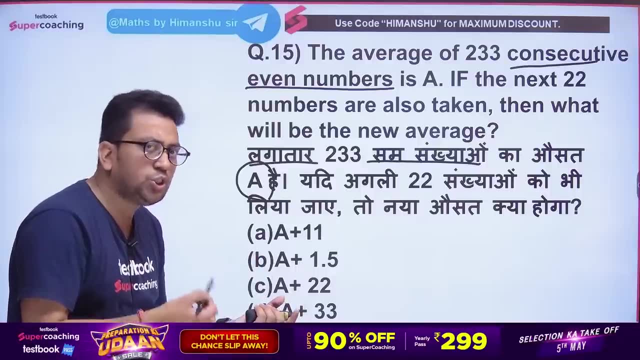 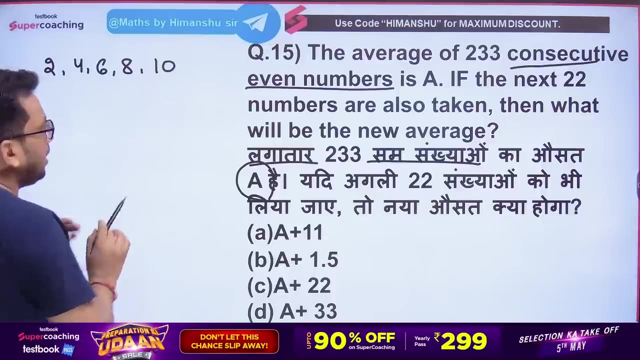 numbers. if it is a, if the next two numbers are added, then what will be the new condition, then the way to shine? it is different. okay, what is it? I can teach you its concept also. if you are ready to learn quickly, then come here. see 2, 4, 8 and 10, son, he is talking. 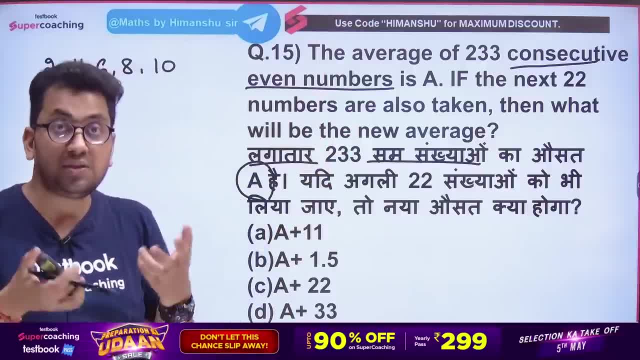 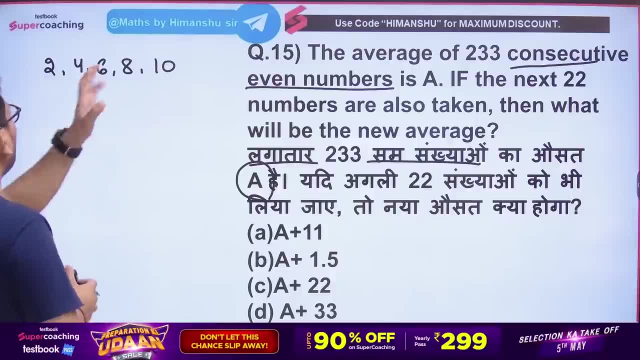 about 233 consecutive numbers. I will talk about 5, I understood the concept. only I have to understand- then accept it, my son- that I have to calculate the ratio of all the 5 consecutive numbers. tell me what will happen, son. you will say that the number of the middle 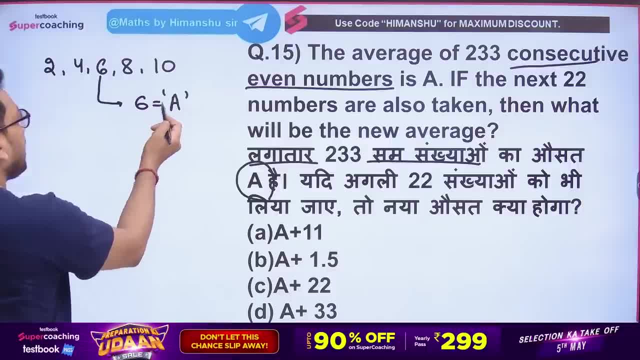 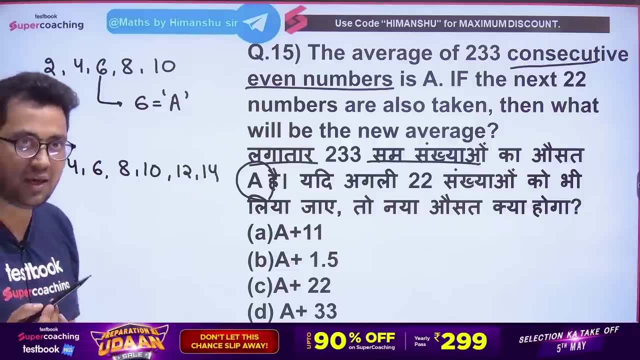 is the ratio, that is, the average is 6,. assume that the average will be called A in the question. now I am saying that the next two numbers should also be added. that is, after 2, 4, 6, 8, 10,, what will be the next two sum numbers? 12 and 14,? son, this is going to come tell. me the ratio of these. what will happen then? you will say that the average will be 12 and 14, then you will say that the average will be 12 and 14, then you will say that the average will be 12. 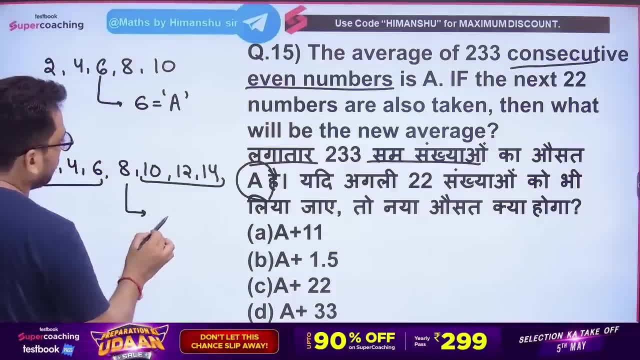 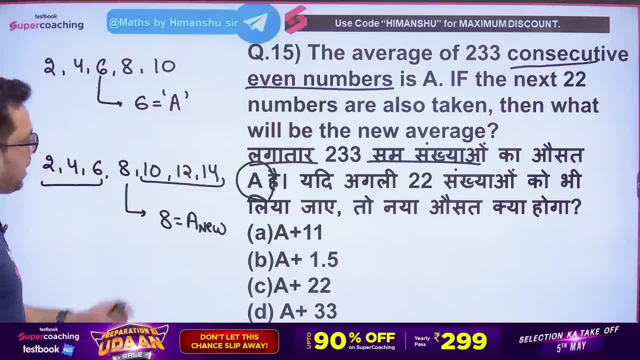 and 14,. then you will say that the average will be 12 and over here. and if the rocking Elima is placed next to the 3, the new ratio will be eight. you tell me what has happened to me. the new average is 8,. it is New average now. you tell me in new average. 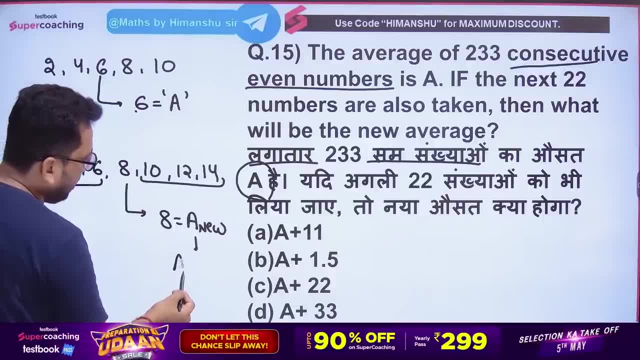 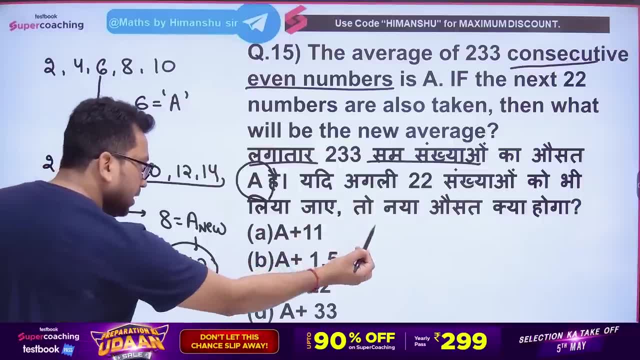 how is the relation with the old average? so you will tell that even the first one is connecting, then there is no connection. what is happening in? the first two is connecting, then why did you connect only two? now the concept will shine from here, and the method. 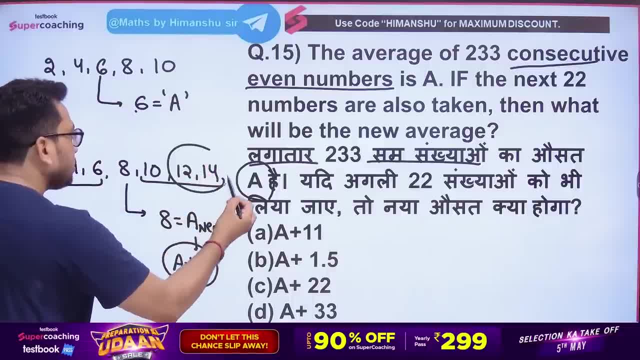 of shine will come out of here. you will decide that you connected the next two numbers. you will say: did you connect? then you also have wood School one. there is also a connection. If you add the two numbers, then can? there is a connection. 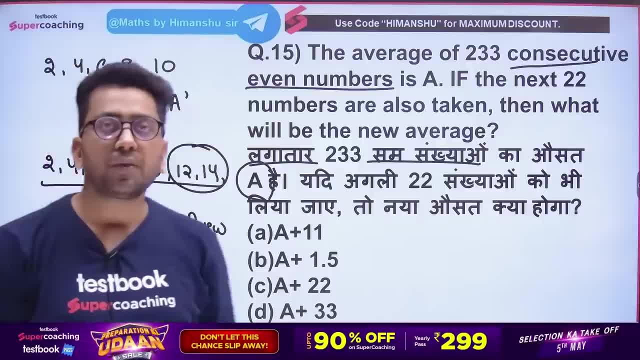 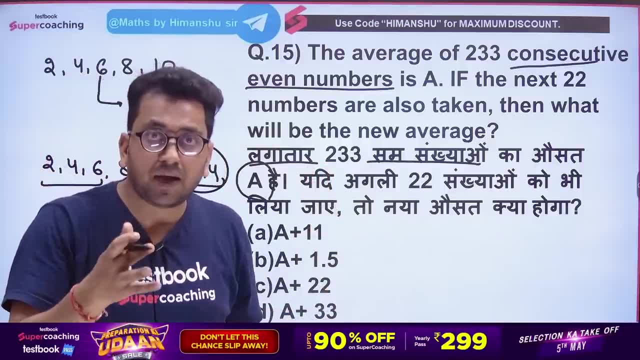 so average mein 2 jodh gaya. Wolo haan ki na Agli 2 sankhya jodi to direct 2 jodh gaya. Achcha sir, yeh concept hai kya? Yani yahan 2 se bhaag nahi karna. 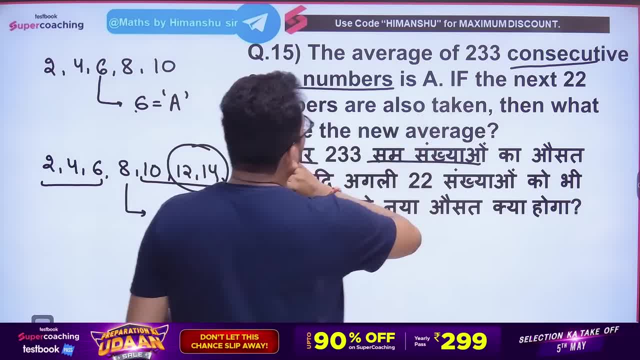 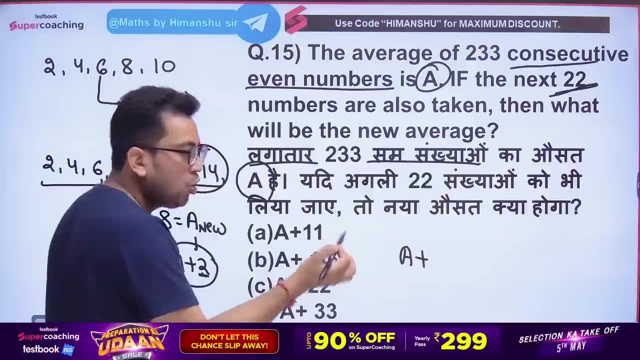 Main kaunga nahi, Aap kahoge. achcha sir. yani, agar inka ausat 230 sankhyaon, ka ausat A tha, aur agli 22 sankhya jodi ja rahi hai, to direct 22 jodh denge kya. 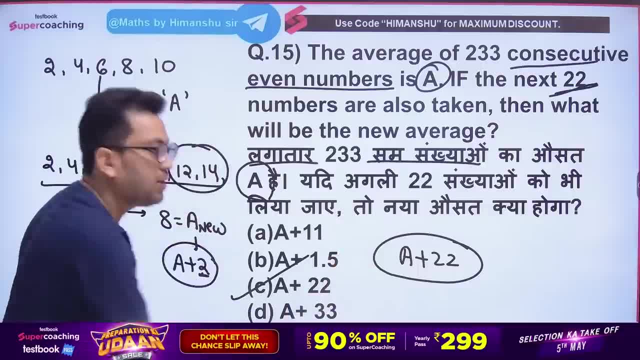 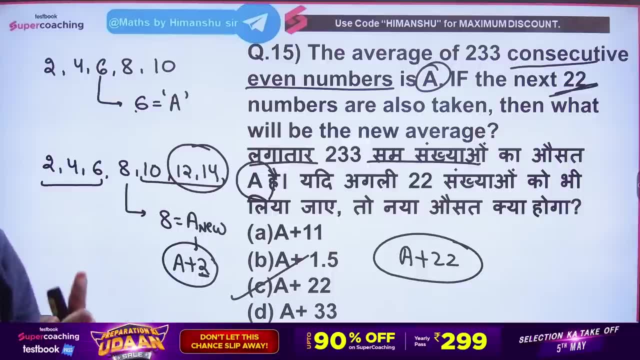 Main kaunga haan miralal, Yani ki. option number C, hamara answer A, plus 22, hamara answer Wolo baad samajh aari hai Clear hai kya Yeh hai chamkane ka? 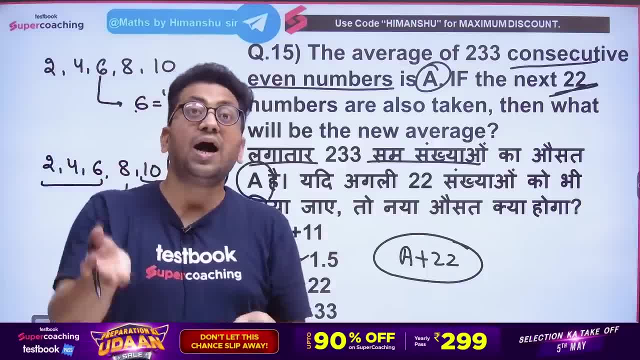 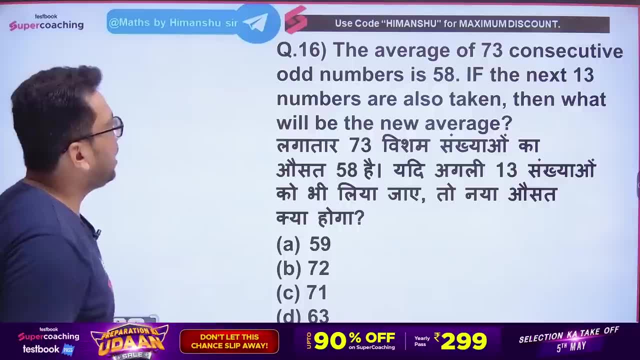 Sir, even hoga, yeh to odd hoga. kya hoga? Even ho, odd ho same hone wala hai. Bas prakrtik sankhya mein yeh karna, ki jo bhi aapke paas number aayega. 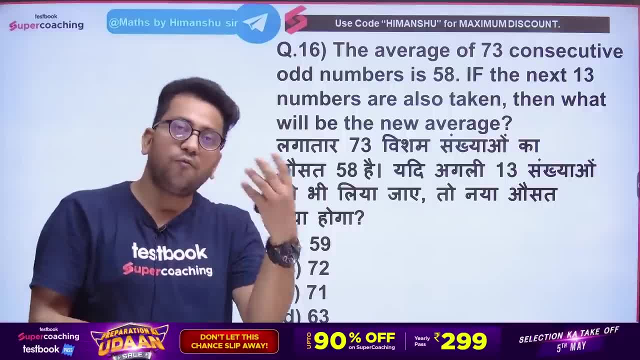 agli jitni sankhya hai, hungi uska aadha karoge, aur fir usko jodh hoge, Yeh direct jodh do Matlab. yeh to aur bhi asaan hai, Agla sawal. 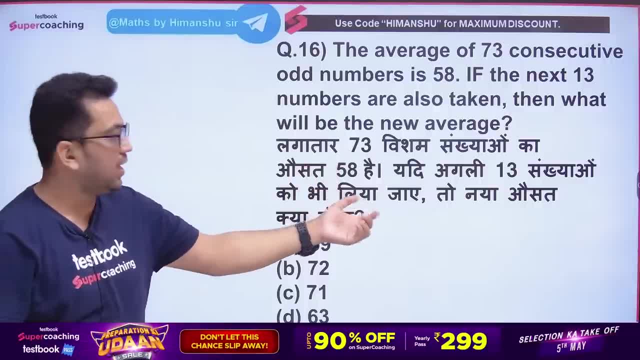 kera lagataar 73 visham sankhyaon, ka awsat 58 hain. agli 13 sankhyaon ko bhi le liya. jaye toh naya awsat. kya hoga? Jaldi se answer kariye. 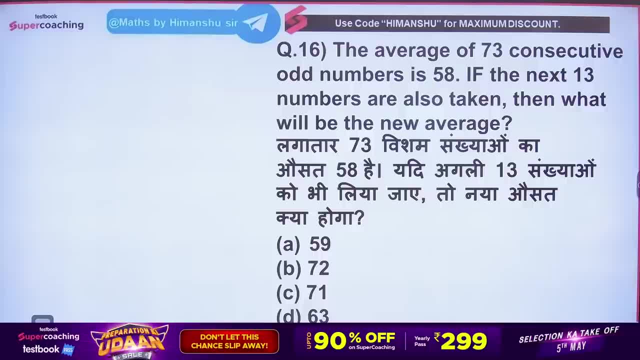 Main chahunga, har ek bachcha uttar de Sabi ke sabi Answer. kariye bata bataye, kya answer aayega. Kik, main dekh paa raha hu, yaha par aap sabi ke like ki sankhya badi kam hai. 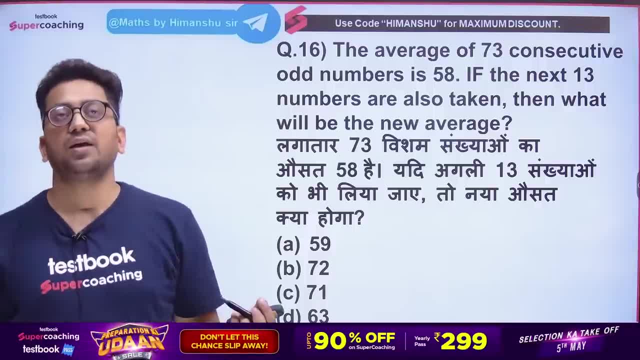 Toh, agar aap loo ko samajh aa raha hai, maza aa raha hai, toh ek baar like ke button pe click kar dijiye: saari ke saari Thik hai. Mujhe samajh aa aega. 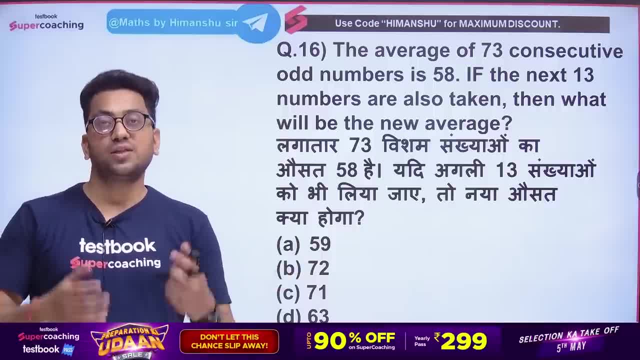 ki mera bachcha har ek cheez ko achche samajh paa raha hai, session pasandh kar raha hai. toh merko aur effort Yeh man hota hai. bata ab, yeh dil hota hai na. 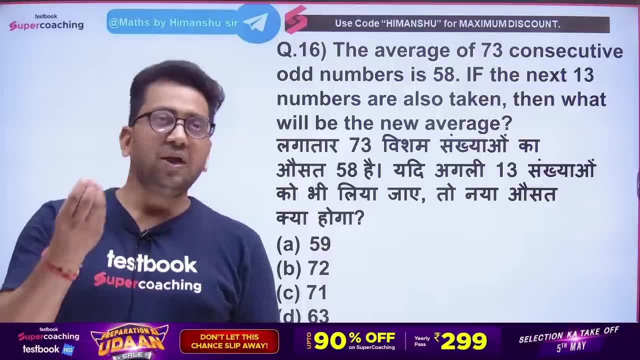 vo bada, bada khush ho jata hai, ki mera bachcha samajh paa raha hai. Wahi motive se mai har ek class lekar aata hu, ki aap ke liye math ko mai asaan bana du. 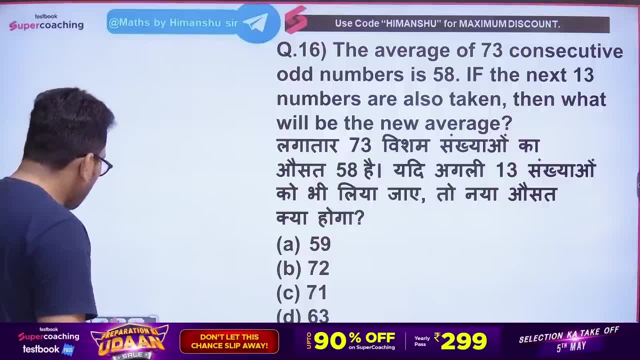 Gadit ko asaan bana du. Liko bata 71 answer kar rahe hain. saari ke saari 71 answer kar rahe hain. bohot asaan hai, bata ki aap kahoge AUSAT 58 hai. 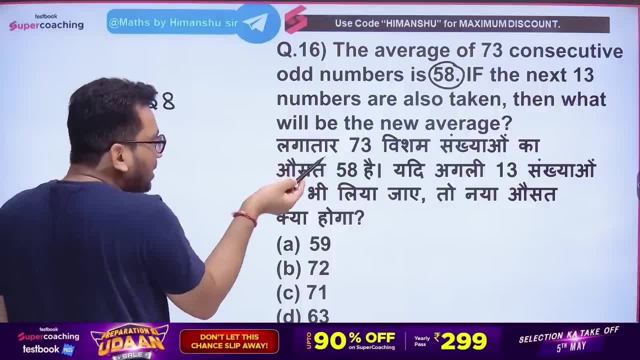 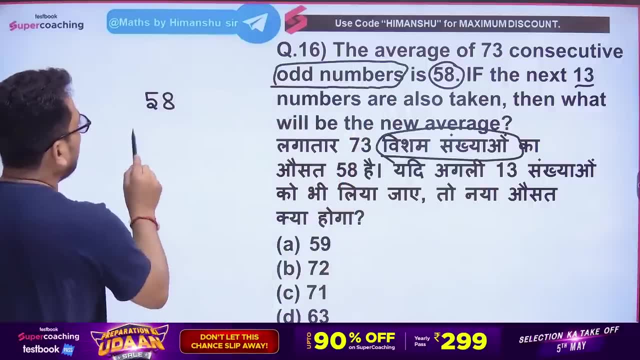 haan, sir hai Agli kitni sankhyaan liye jaa rahi hain 13 haan. Lekin agar yeh visham ki baat boli hai, odd ki baat boli hai, visham ki baat boli hai. 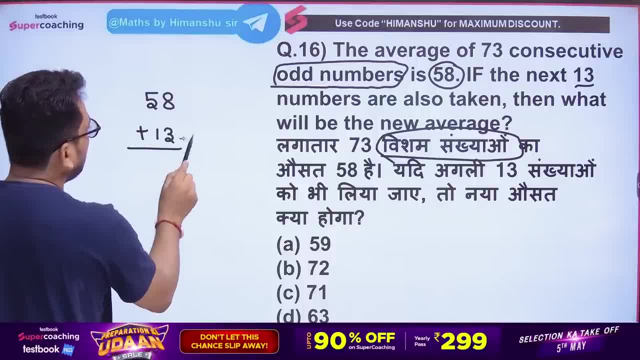 toh mai seeda jodh dunga, sir 13.. Mai sochunga ochunga hai, kuch nahi. 8 aur 3,, 11. Aansal gaya 1, yaani 71 hamara uttar hai. 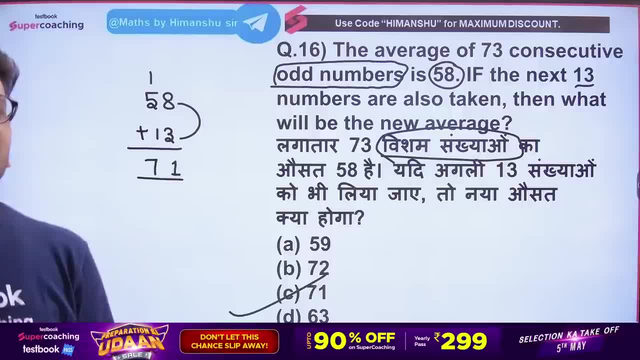 vikalpasi hamara Thik hai Chamka diya Mujhe batao, Aisa kaun hoga, aisa koi bachcha, jisko na samajh kama jaa raha ho, Thik hai. 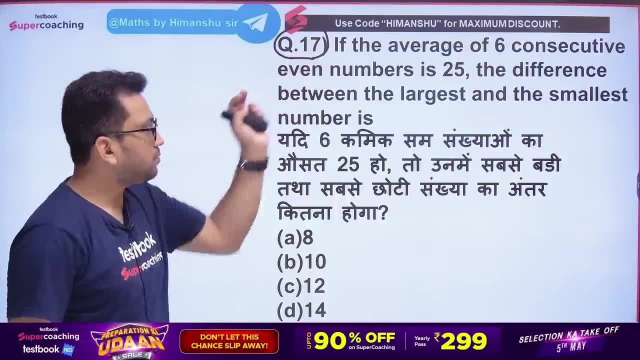 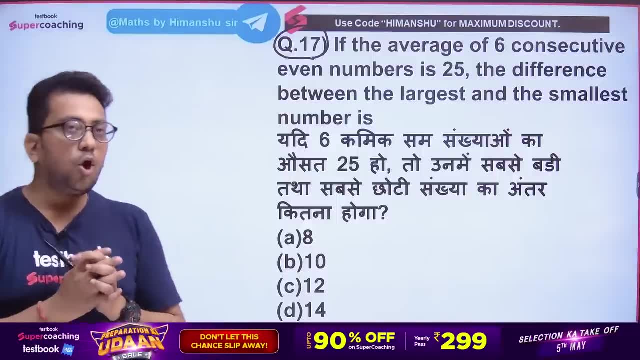 Aayega bata, aayega Thik hai Agla sawal. Seventeenth question: Jaldi se bataye, Ab yaha par hamne sawal me thoda sa aur badlaab kiya hai Thik hai. 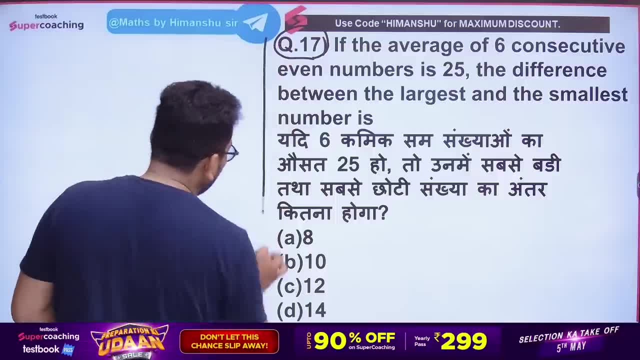 Aur badlaab kiya hai aur aapko yaha par ab hum aur concept sikhayenge. Thik hai, Dhyan se sikhye ga Mai zara ith concept ko aapko sikhane ke liye. 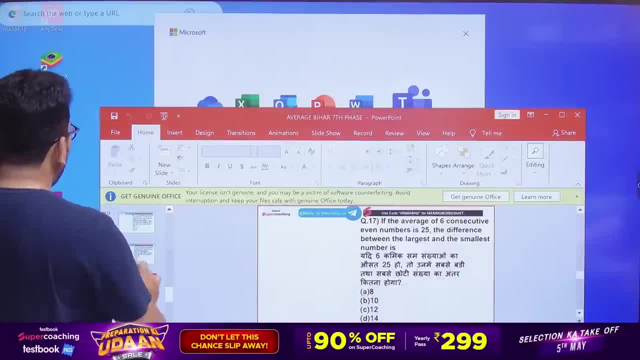 ek bar yaha par aa jaana chahta hoon Thik hai Ith concept ko sikhane ke liye ek bar yaha par aa jaana chahta hoon Ki mai yeh chahta hoon ki aap loko na ek bar padhlo. 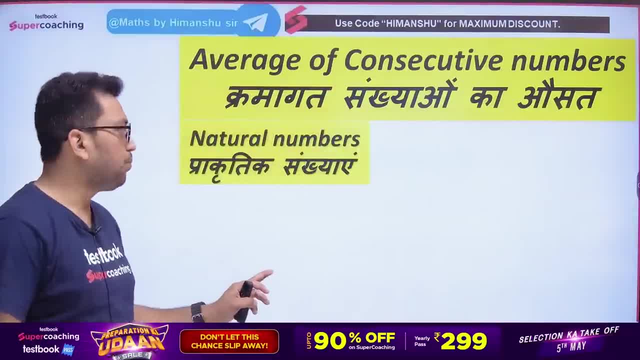 Thik hai Aur phir baar baar padhne, ki wo need hi na ho, wo zaroort hi na ho, Dekho maine, aapke saamne na prakarthik sankhya hai di. 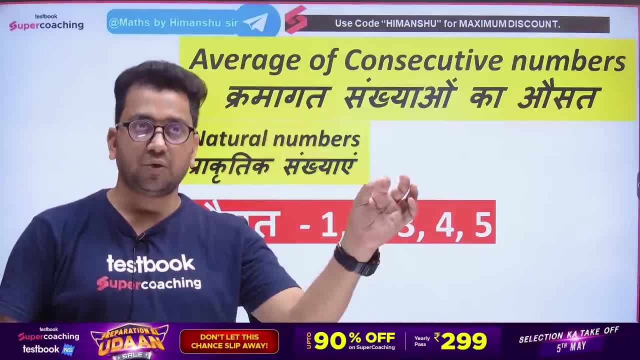 Mai sirf ek example dunga, ek udharan dunga, aur phir uss sawal par aa jaunga: Koki, yahi se aapka wo sawal chamkega, Bohot basic cheez hai Dekho. 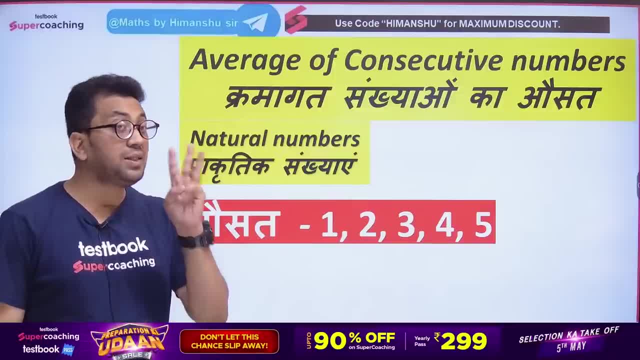 iska iska osat mai kif tarike se nikal sakta hoon Iska osat beta mai teen tariko se nikal sakta hoon, Itne tariko se, teen tariko se, Aur dekh leta hoon ki. 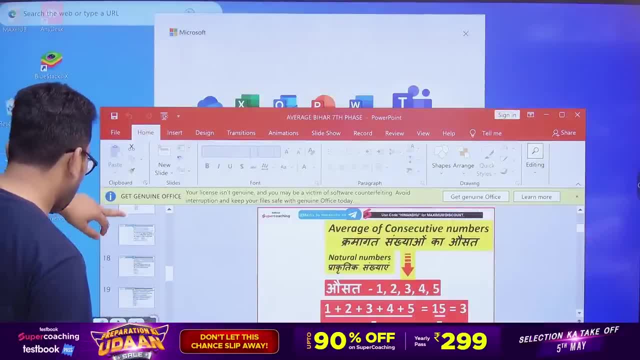 aapko samjhaya nahi hai, kya isma koki dala, toh hoga. maine Ko check kar de raha hoon, Thik hai. agar nahi hoga, toh phir haan. 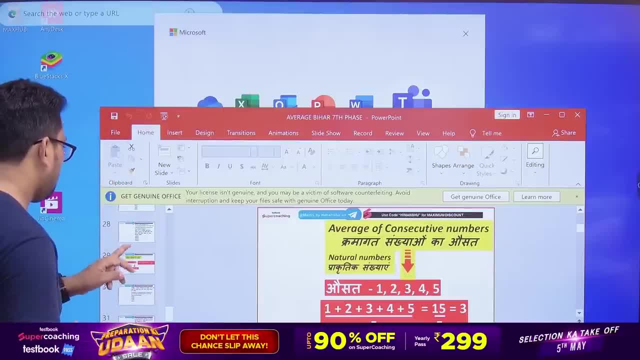 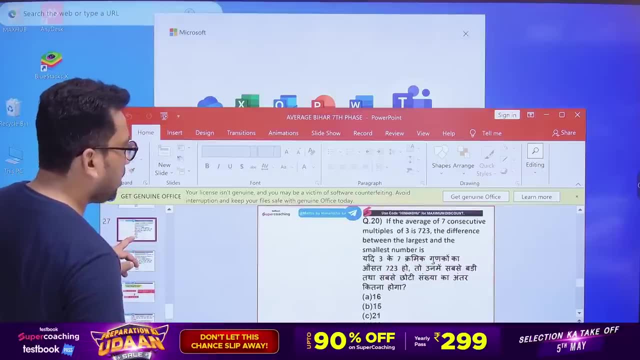 hai bai hai Thik. Hmmm, hai yaha par Thik hai abhi hum kaha par the abhi hum thik hai. Isko mai yahaar pe bata deta hu, Chalo. 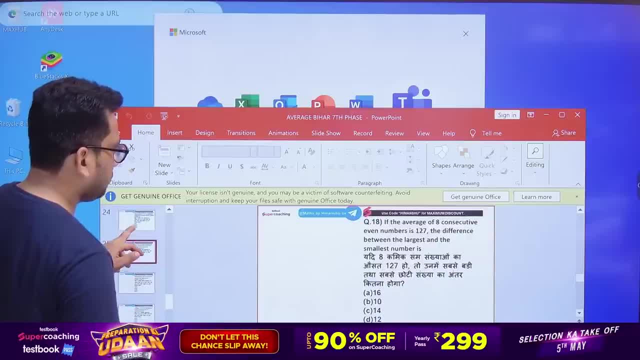 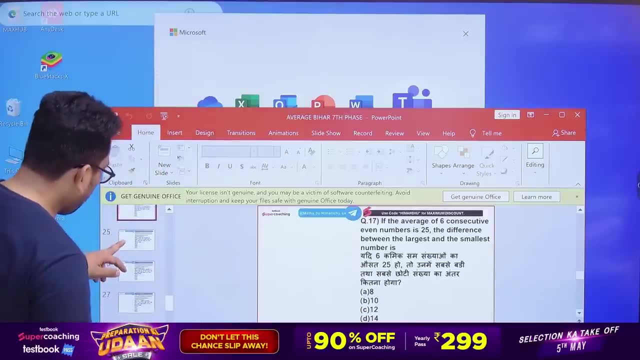 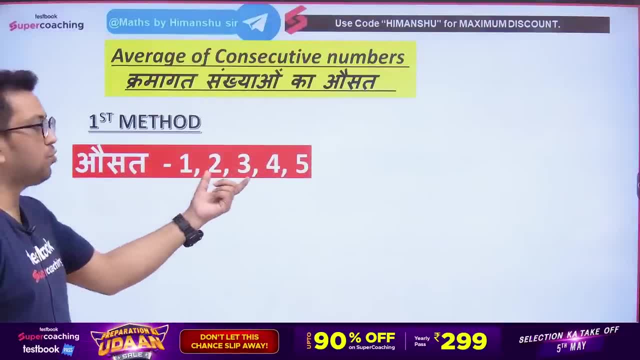 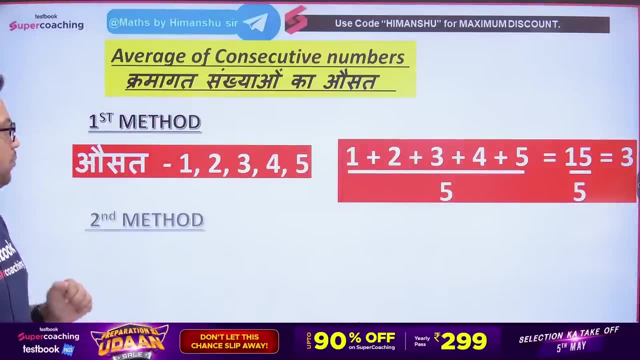 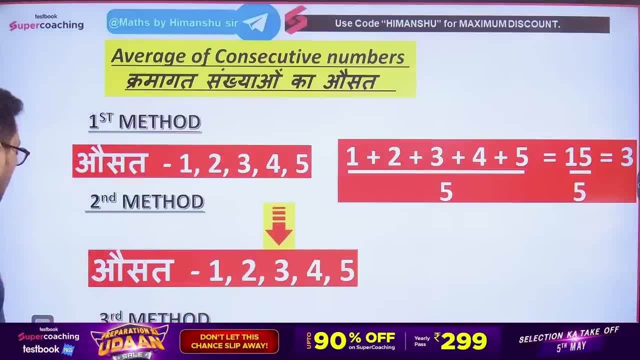 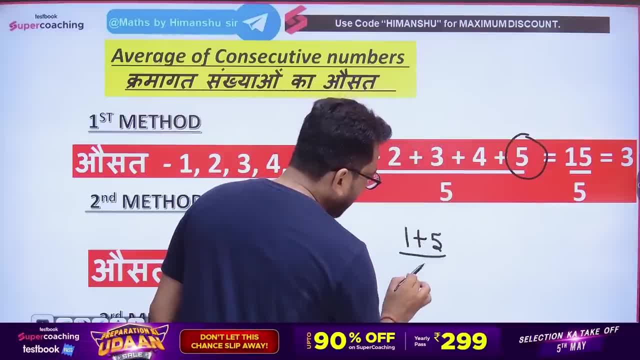 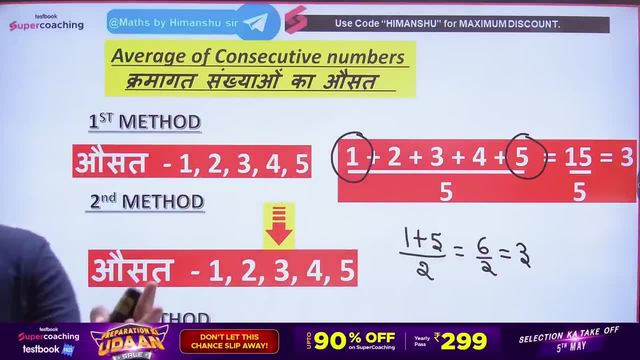 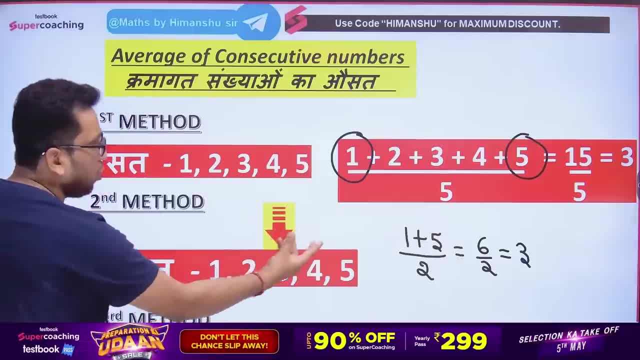 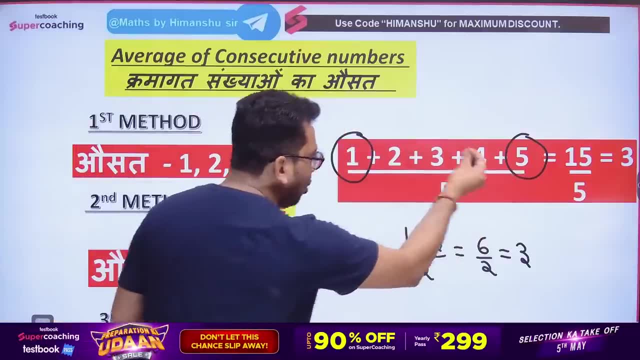 sabar, sabar, sabar. The third way is to add the first number and the last number, divide by 2, then only the number will come. That is what will be the first number. it will be the smallest number. that is the smallest. 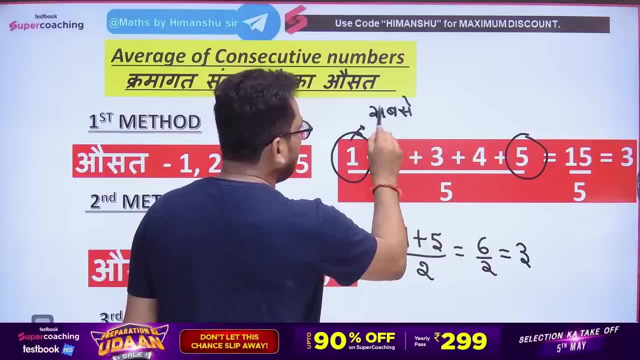 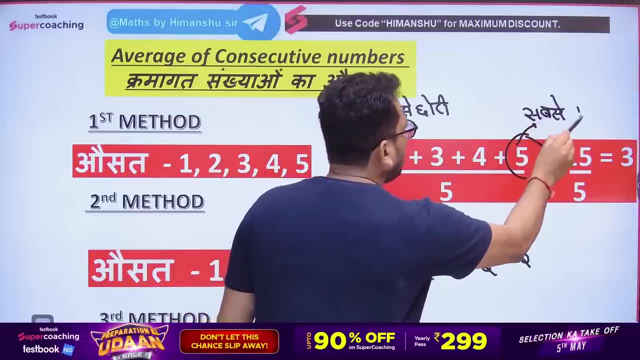 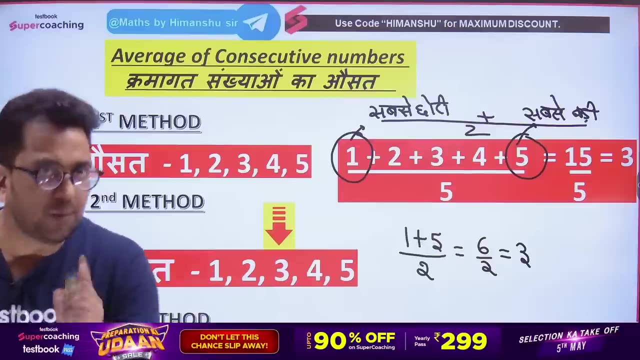 number. That is, add the smallest and add the largest, add the largest and divide by 2, then what will you get in the number of numbers? The number will come. So, on this concept, on this concept, now see how the questions are being asked. 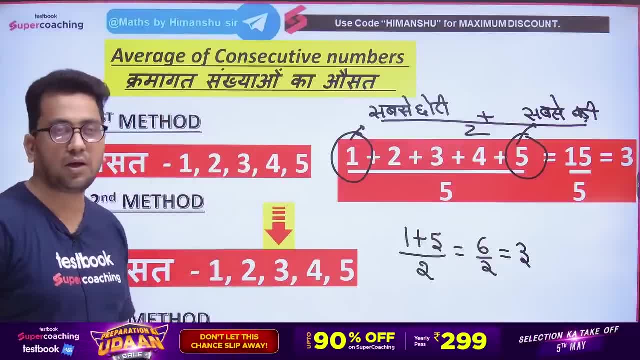 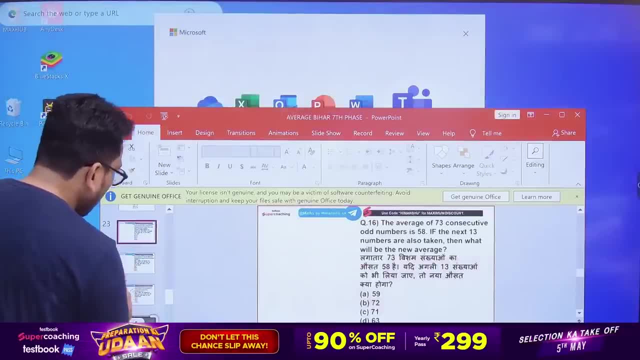 Okay, everyone understood this. now come to the questions. Now, see, you will start shining all the things. Okay, all the things will shine, one by one. Look very carefully. We were on this question on the 17th question. 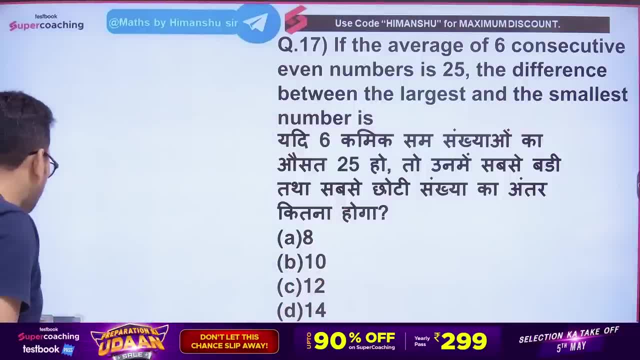 See what he is saying. If the average of all six numbers is 25, then 1,, 2,, 3,, 4,, 5,, 6,, 7,, 8,, 9,, 10,, 11,, 12,, 13,. 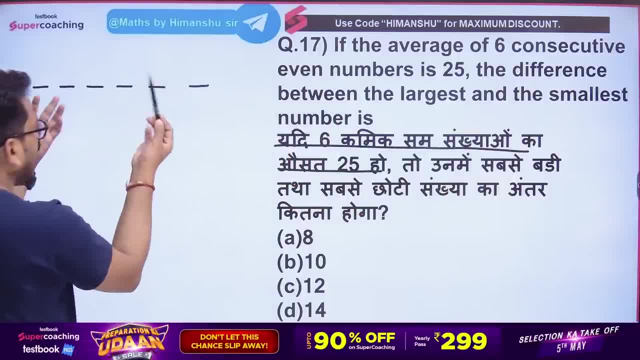 14,, 15,, 16,, 17,, 18,, 19,, 20.. There are 6 number of numbers. Their average is 25.. So he is saying: find out the difference between the smallest and the largest number. 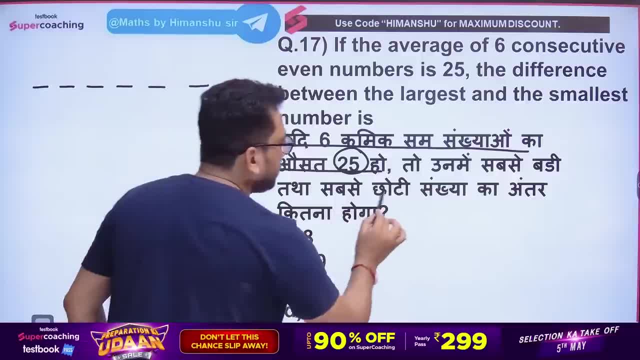 Okay, this is also very easy. This is also very easy. Come, let's come here first. Okay, now give me its answer. give its answer. Means. what will our child do To do this? he will say that the average is 25, so the number in the middle will be 25.. 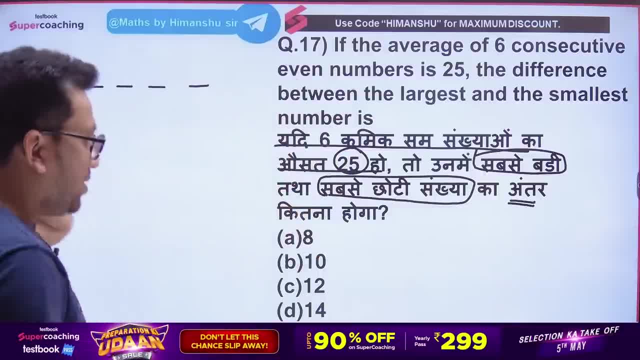 Say yes, Kee na. How many numbers will come in the middle? 25 will come. Say yes, Kee na. Yes, sir, 25 will come. Sir, 25 will come. 25 will come. Yes, sir, 25 will come. 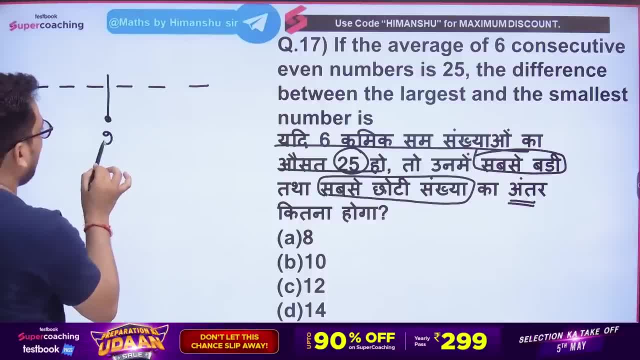 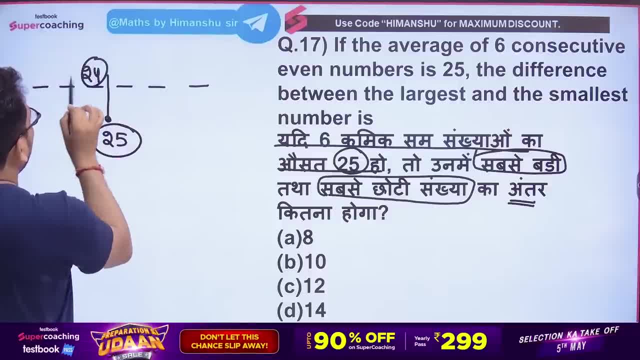 Sir, what will you get before 25?? Sir, you will get 24.. What will you get before 24?? You will get 22.. What will you get before 22?? You will get 20.. Do you understand what I am saying? 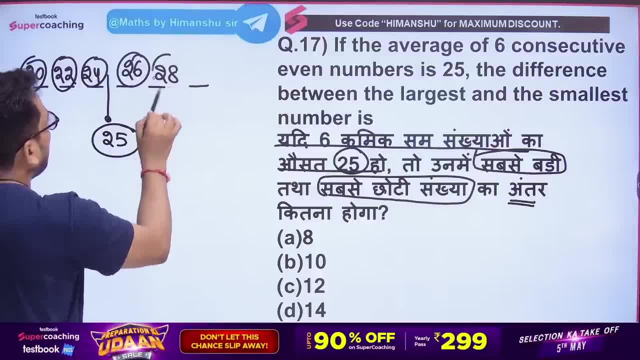 What will you get after 25?? You will get 26.. What will you get after 26?? You will get 28.. What will you get after 28?? You will get 30. Say: do you understand? Yes, sir, I understand. 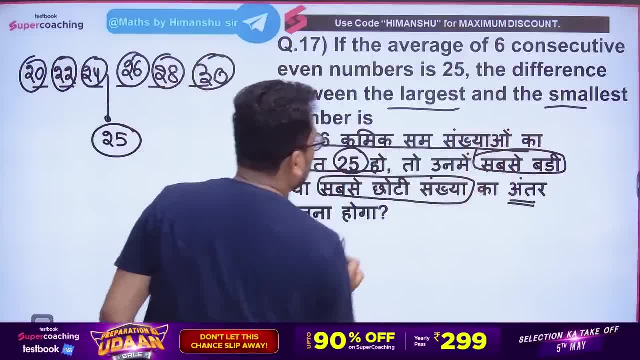 Okay, sir. now I want to find out the difference between the biggest and the smallest. So the biggest is 30 and the smallest is 20.. If we find out the difference between 30 and 20, then how much will it be? 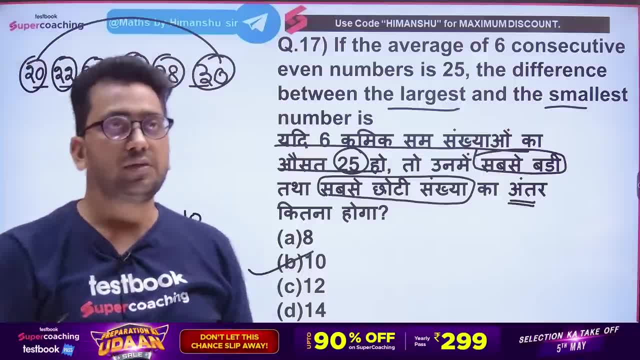 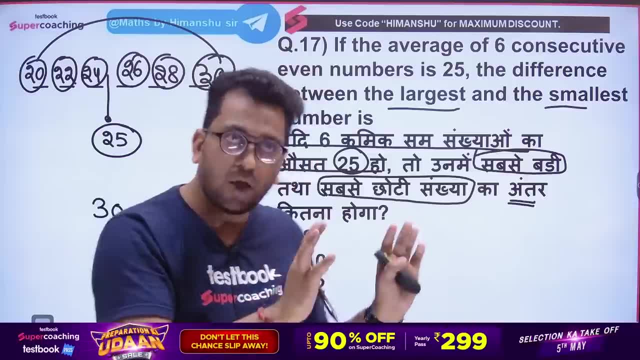 There will be a difference of 10,, that is, we will get the answer of option B, We will get the answer of 10.. Say yes, Keena. Is this the thing that all the children are able to understand, The concepts that I have just explained? how are the questions based on that? 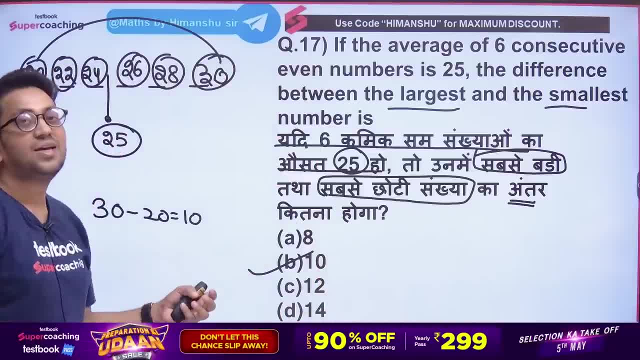 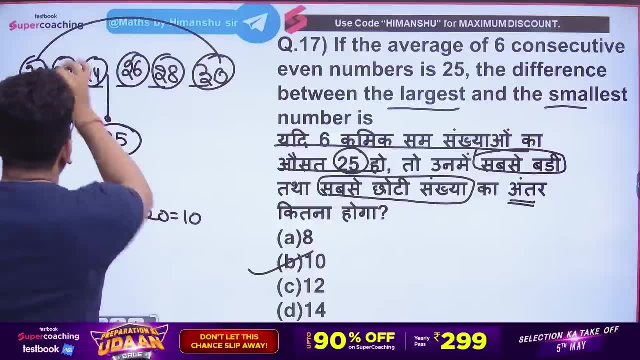 We will also do that now, But this was very easy, So it came in the middle, Let's see. So did you understand all this? But I say that you do not need to do this to ask this question. Not at all. 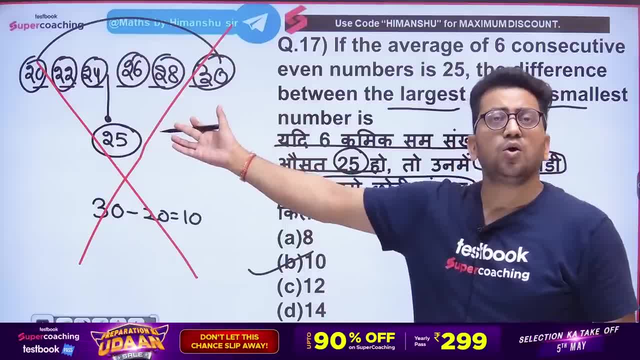 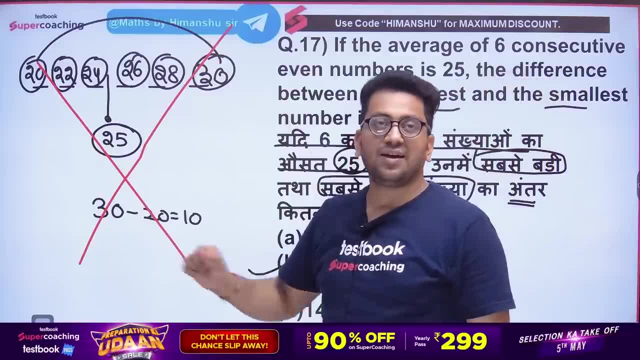 You will say: sir, why are you saying this? This is easy, Why are you putting all this nonsense for us? This is so easy. I am saying that it is still easy. Why is it easy? Because the numbers are less. 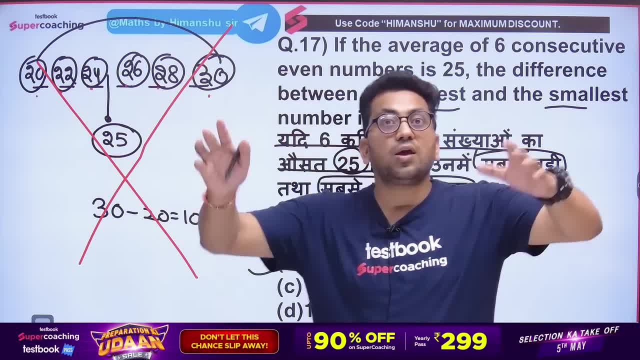 There are 1,, 2, 3,, 4,, 5, 6.. I am saying that it would have been 106.. Then all the numbers would have been written. Tell me, Then all the numbers would have been written. 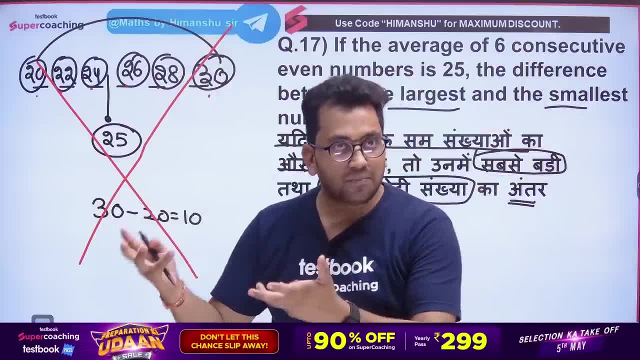 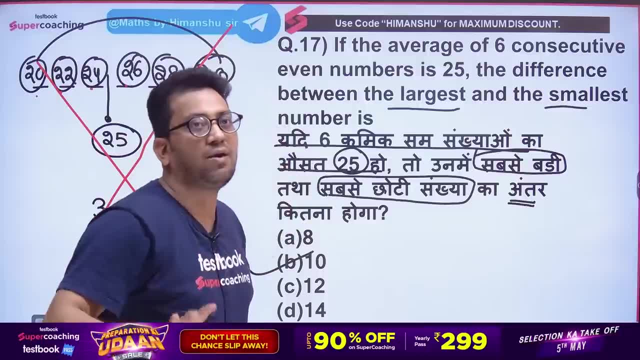 Sir, if we would have seen the difference, the age would have passed. The exam is of limited time. If we have to give the answer at that time, then we will shine The way to shine. What is the way to shine now? 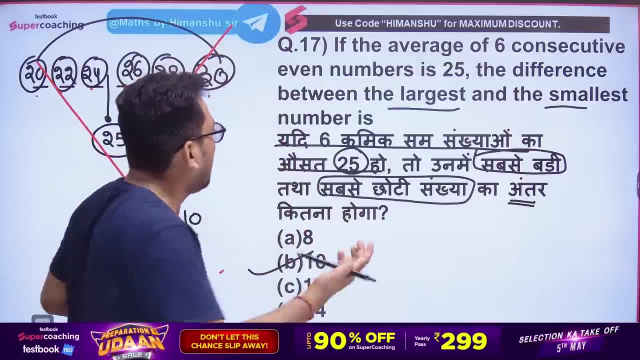 Look at the way to shine. You bring your Himanshu Saraswati's measurements. What do you have to see? What is the measure? It does not mean anything. You will say what. It does not mean anything, sir. 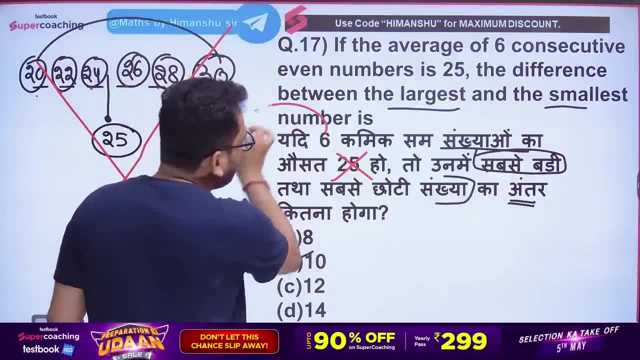 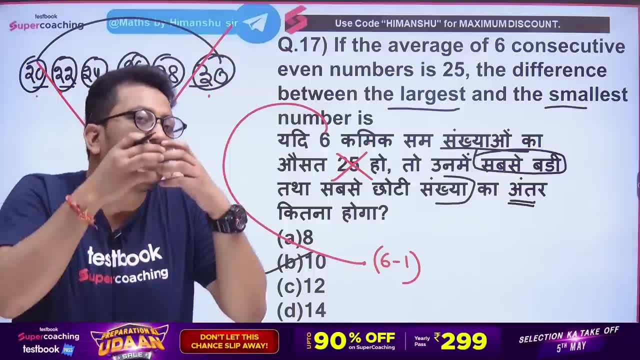 No. Now look at the numbers. How many numbers are there? There are six circular numbers. Reduce one out of six, Reduce one out of all the numbers And do the calculation from the difference. From which difference? What does difference mean? 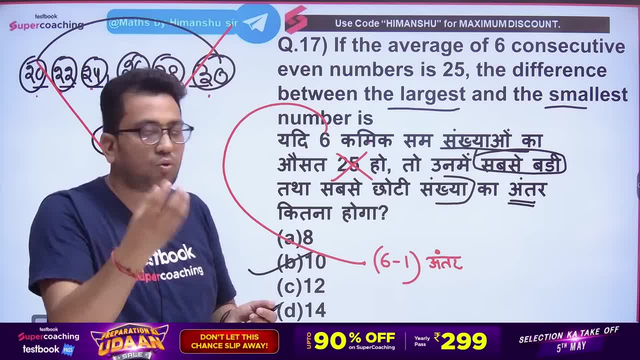 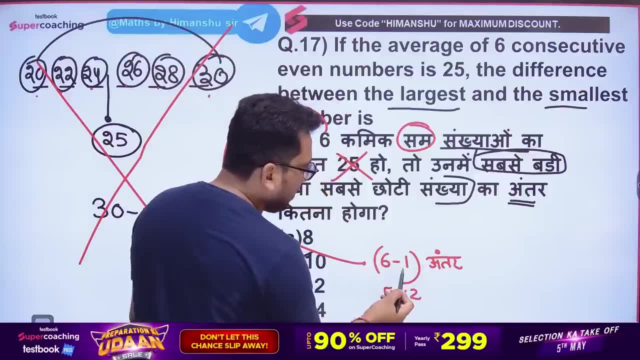 In this sequence, the difference between the columns. multiply it with that difference. Now, as these are all numbers, then there is a difference of two in all numbers. So multiply it with two. That is five times two, Brother. six minus one is five. 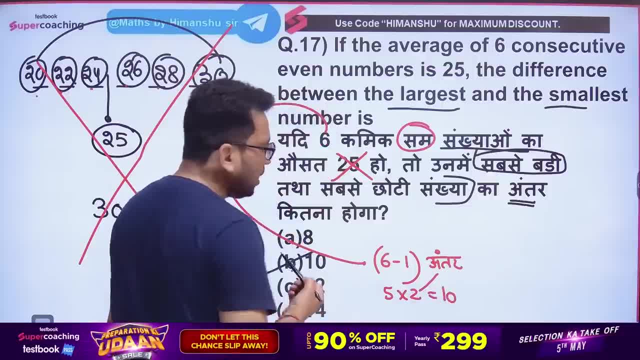 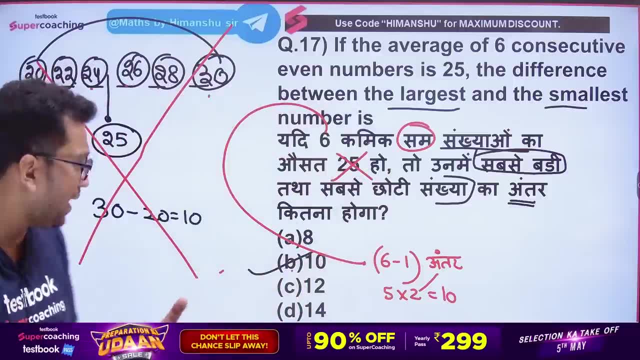 How much is the difference? Two, Five times two, you will get the answer of ten, That is, we have the option B. Hey, shine like this, Shine with concept. This is also a concept Why? Because, sir, if there are six numbers, 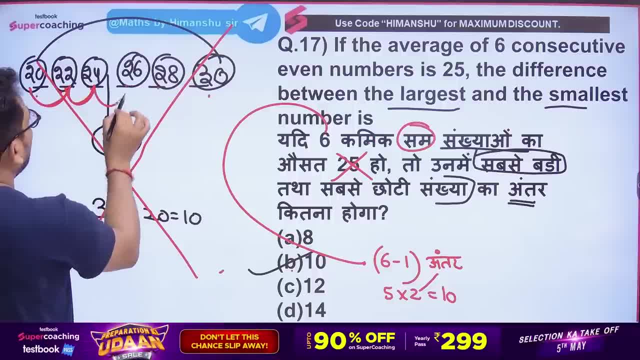 then the difference in them will be five. One, two, three, four, five, One, two, three, four, five, Five differences, And if the difference of one is two, then the difference of five times two will be ten. 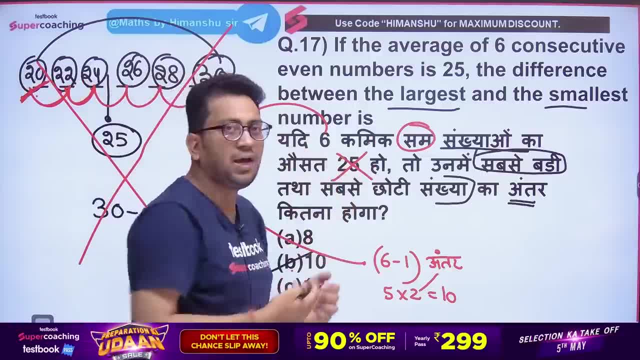 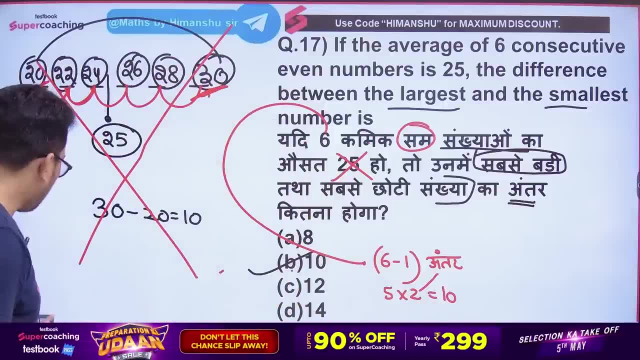 Between the decrease and increase. So, brother, what does the average mean here? Yes, Why should we get it When it doesn't mean anything? We will just shine like this right. Next question: If you understand, then shine this question. 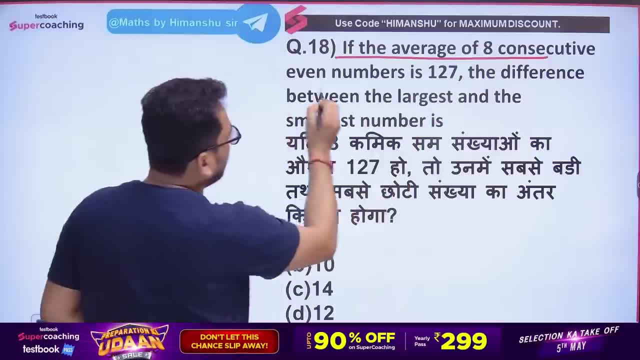 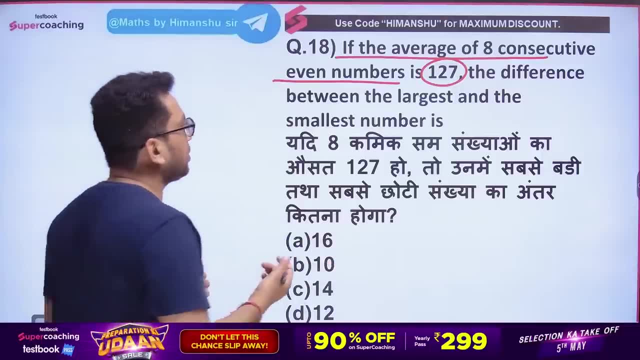 See what he is saying. If the average of eight consecutive even numbers is 127. It is 127,, son. The average of eight consecutive even numbers is 127. Eight. If the average of eight consecutive even numbers is 127,, then you have to tell the difference between the biggest and the smallest. 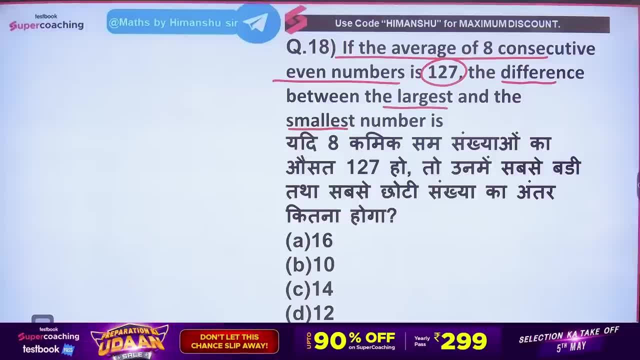 Answer quickly. Tell me what the answer will be. Okay, Ananya Gupta is saying: Yes, son, Absolutely. You also have beta available. son, Practice questions: Absolutely, And it is available with the best content. son, Let's go. 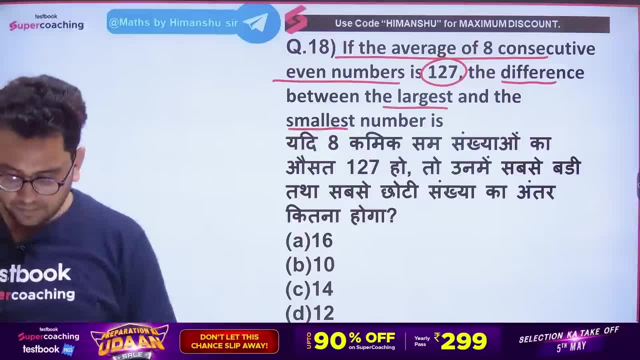 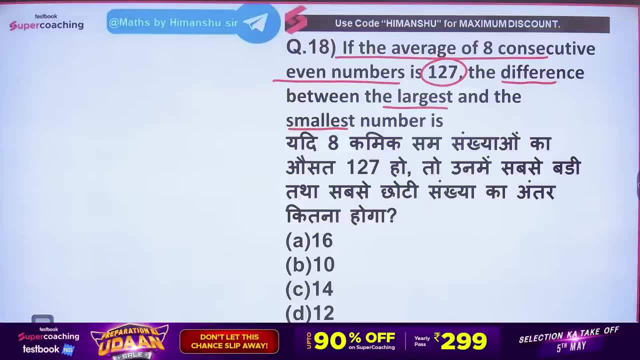 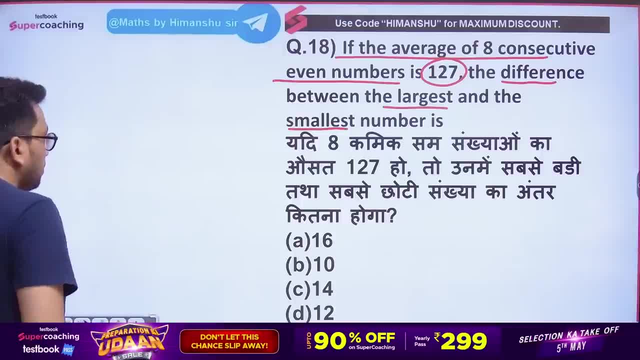 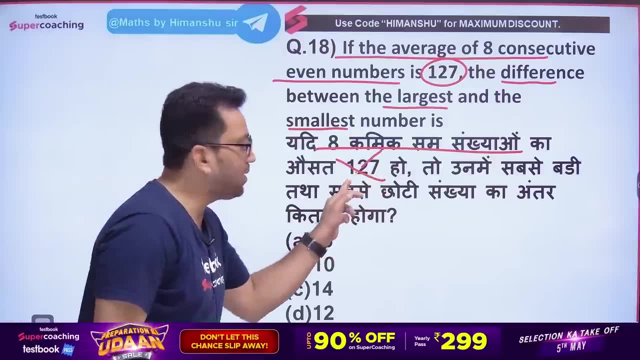 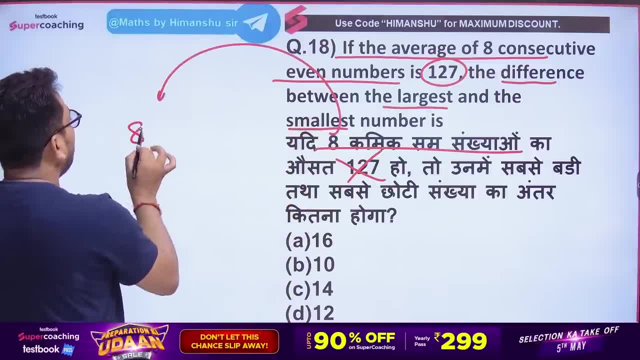 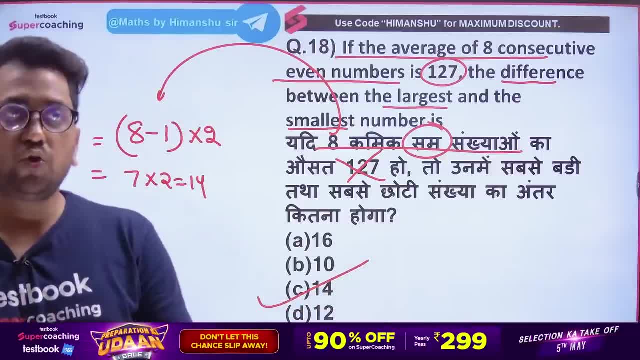 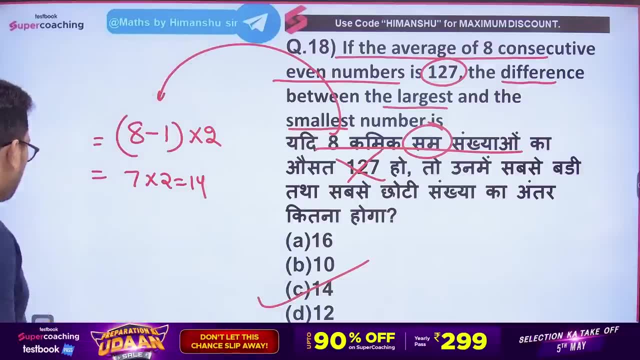 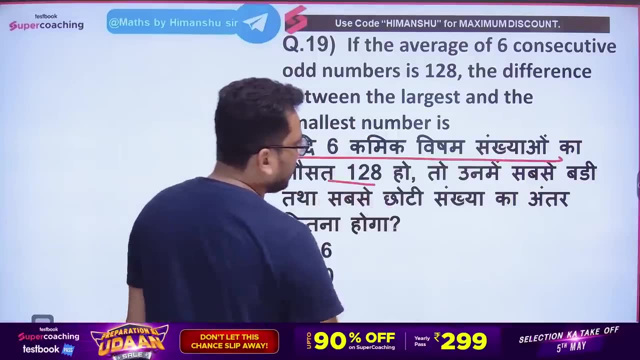 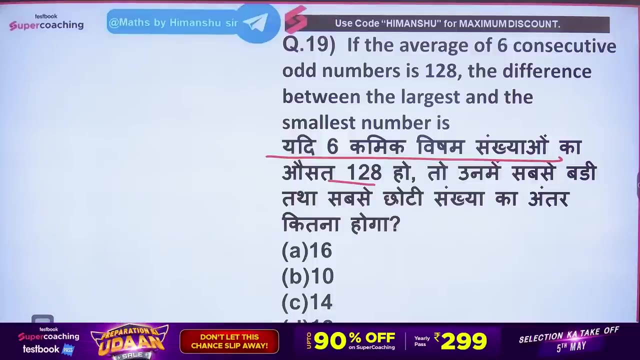 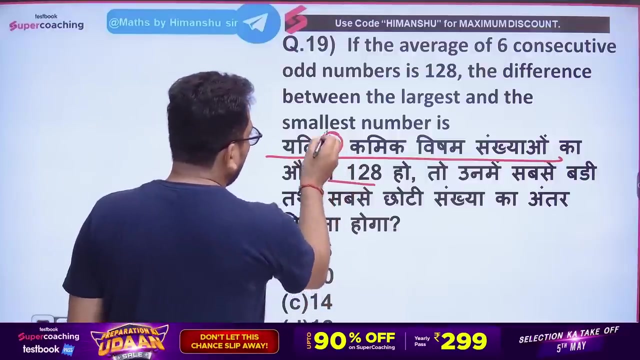 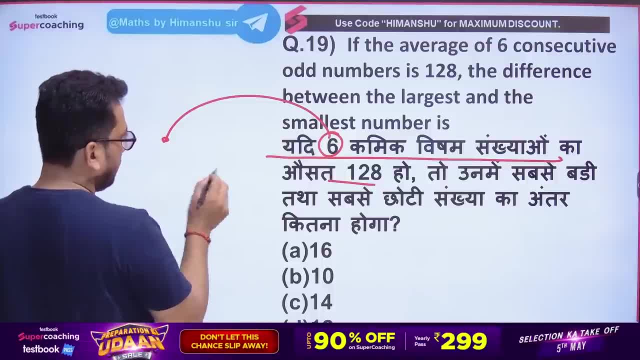 There are 6, right, son. So why are you doing 14?? 10 will come here, right? Okay, if you subtract 1 from 6,, 5,, 5 will not be 10. Because there are 10 number of Karmic numbers, so 10 will be our answer, right. 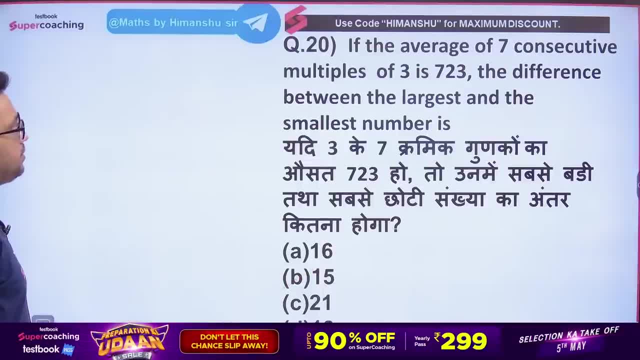 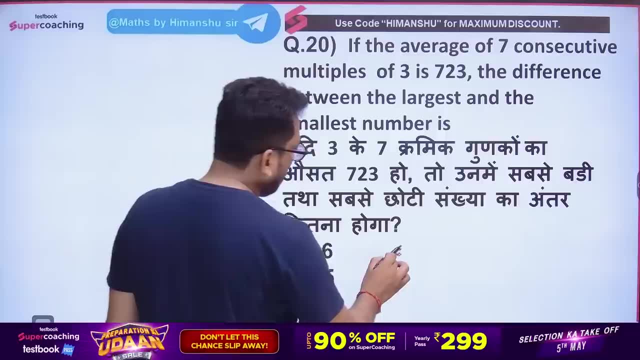 10 will be the right answer. 20th question: Do it carefully. Do it carefully, Okay, Yes, I will tell you in Vikalp D, which you might not be able to see. Vikalp D is 18.. 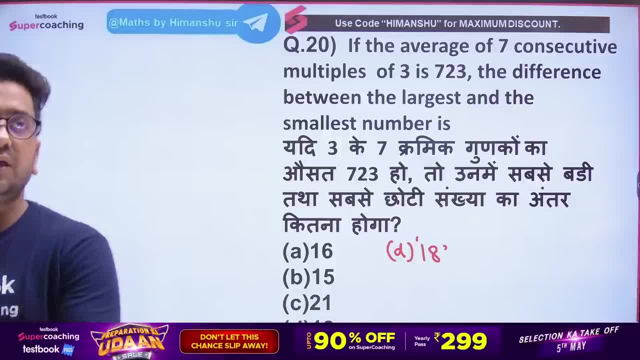 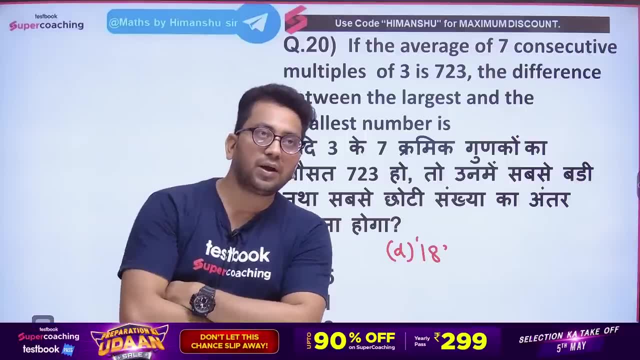 It is 18, right, Vikalp D is 18.. Quickly answer the question. Very good, Pragati Dharmendra Khushbu, Niku Renu Anamika Harendra Pankaj. 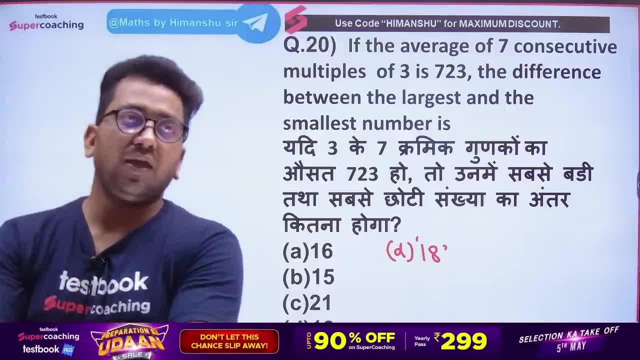 Come on, all the children: Abhisht, Gaurav, Pappu, Pinky. Pappu is also there, Pinky is also there. Very good, Come on. Archana, Anamika, Deepak, Sushma. 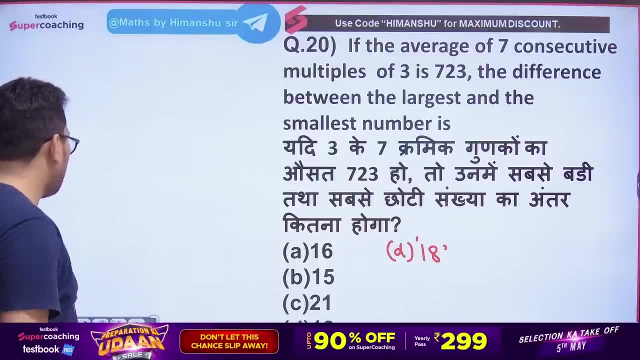 Gautam Poonam Rajesh. All of them are left. This time quickly, with speed. Sir, look here. If there are 7 Karmic numbers of 3, how many are there? 7. How many are there? 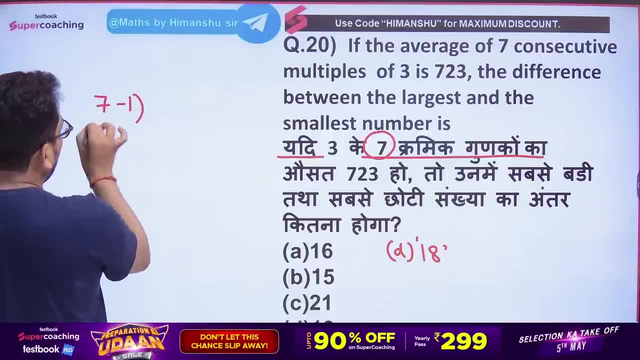 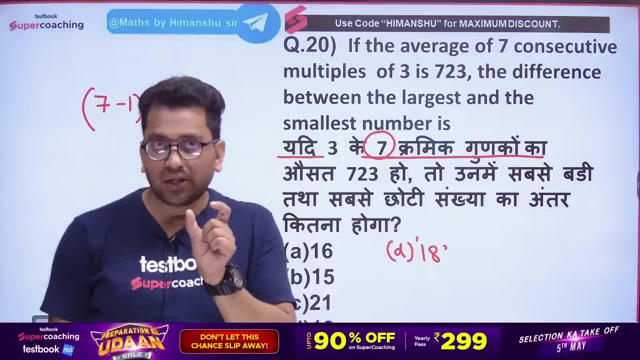 7. There are 7 numbers, So we will reduce 1 out of 7.. Now will it be 2? No, Here it will be 3.. I have told you, with the concept, that the difference between the lines has to be multiplied by that difference. 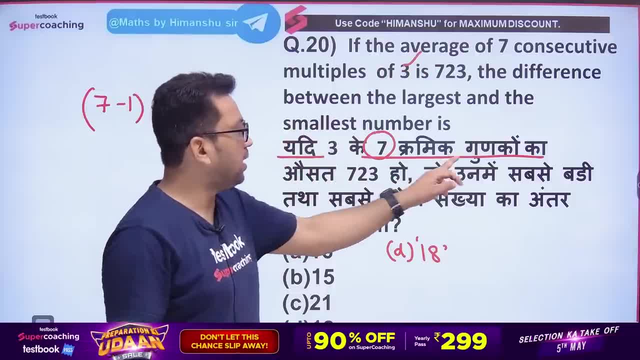 Now, if there are 3 multiples here, there are 3 numbers, right? So the difference between 3 and 3.. If there is a difference between 3 and 3,, 3 times 3 is 3,. 3 times 3 is 6,. 3 times 3 is 9,. 3 times 3 is 12, there is a difference between 3 and 3.. 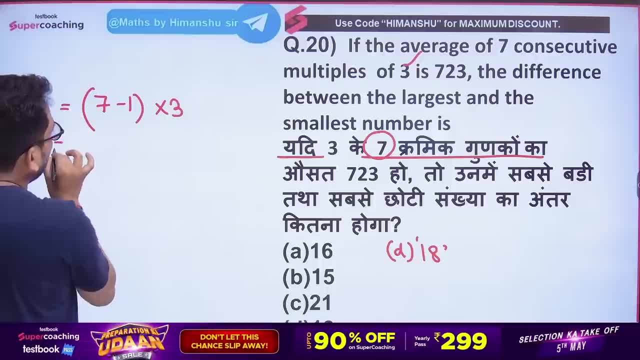 So that means we will multiply it by 3.. So 7 minus 1 is 6, and 6 times 3 is 18.. That means the concept D will be our answer. D will be our answer. 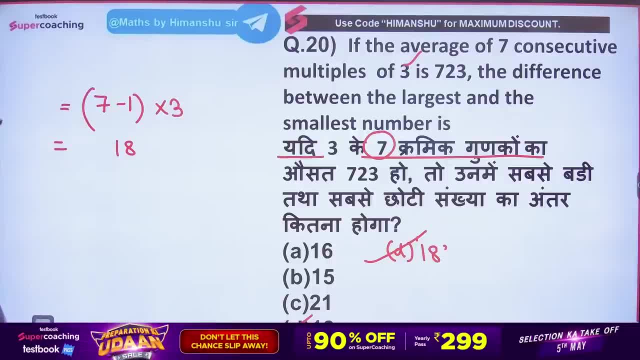 18 will be the right answer. Okay, Are you understanding the thing? You have to do it in this way. Is it clear to all of you? Perfect, 21st question. 21st question. 21st question: Here it is in front of you. 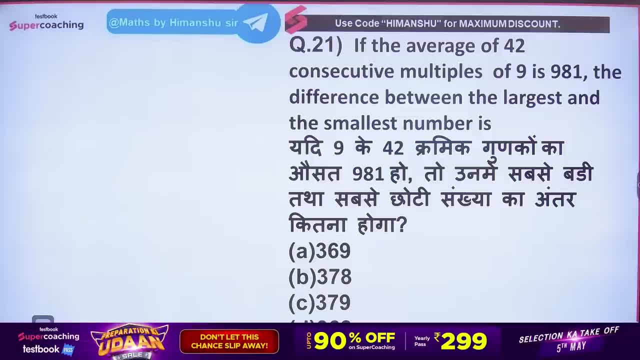 Let's see how many children are able to answer. Answer it correctly. Tell me what will be the answer. son, Let's go. Yes, What will you do? Understand carefully. You said that 9 has 42 karmic qualities, right? 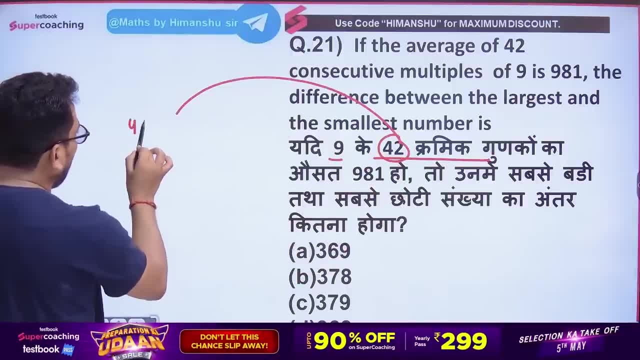 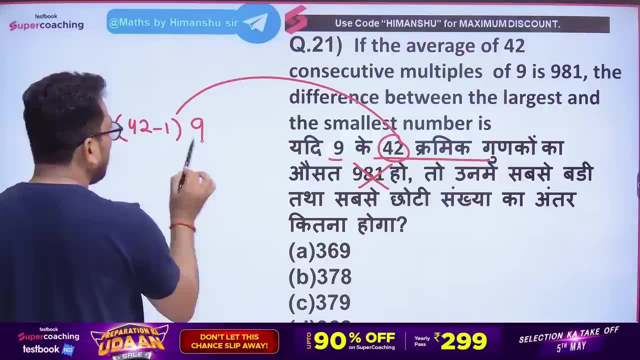 So see, there are 42 qualities. So what will you do from 42? You will reduce 1.. That means you do not care how much measure you have given. And what do we do directly? If you say that there are 9 karmic qualities, then do it from 9.. 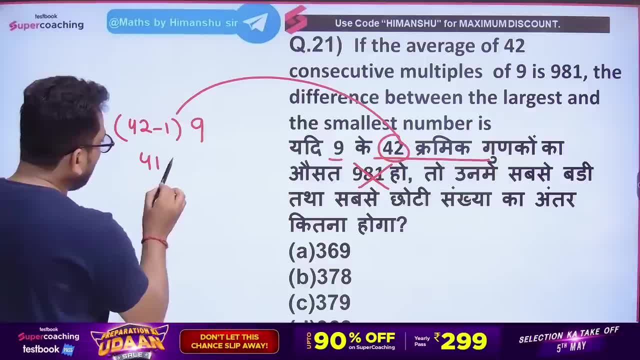 Because there must be a difference of 9 and 9.. Now if we do the calculation from 41 to 9, then 9 is less than 9 and 9 is 36.. That means our answer will be 649.. 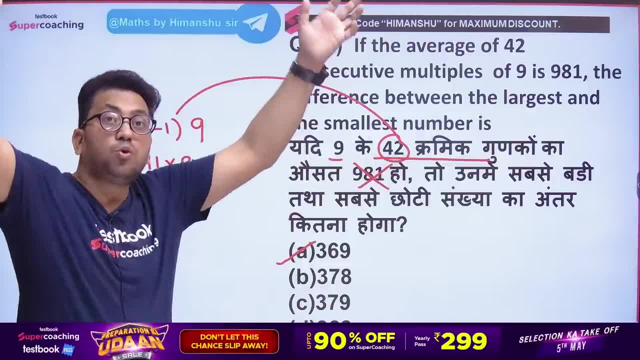 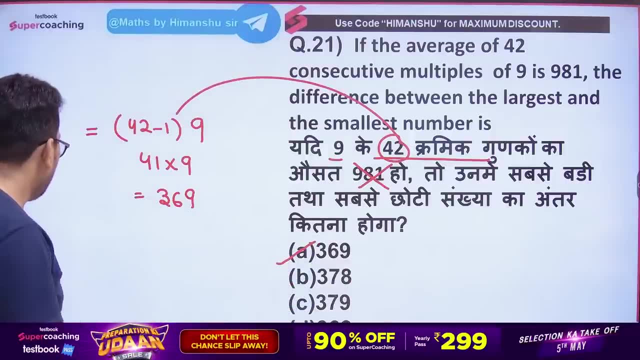 Think for yourself, son. You would have written 42 karmic qualities. Yes, You would have taken small and big. Sir, it would have been night. This would have been our answer. Yes, Come on Now the last question. 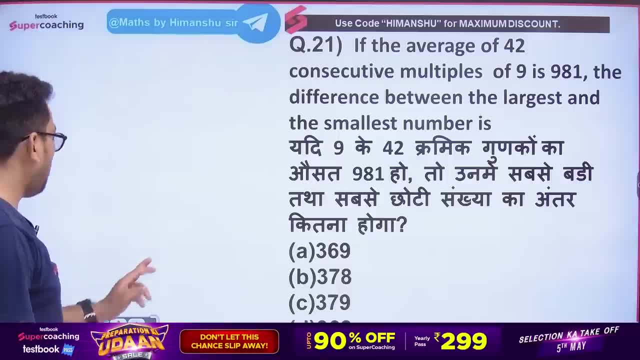 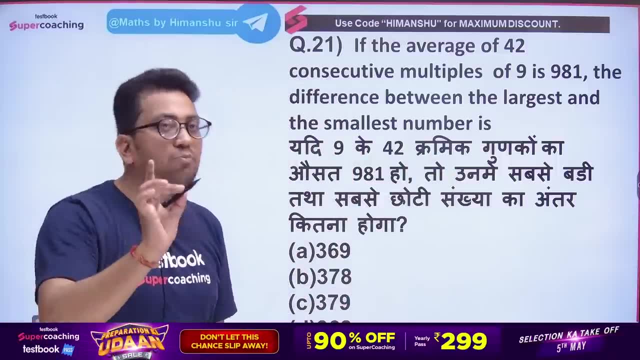 Now the next concept has come. Come on, I am asking you one question. I am asking you one question, I am making a change in this And you all have to answer it in the comment section. Take a screenshot of this. 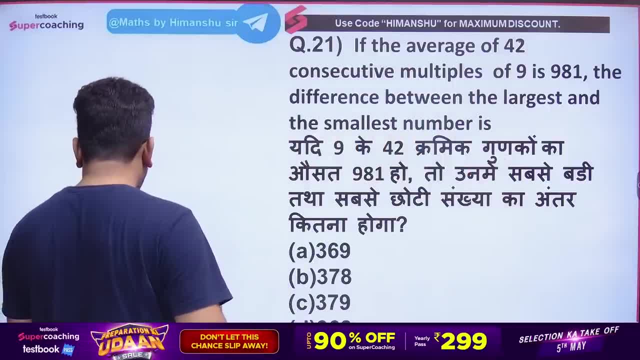 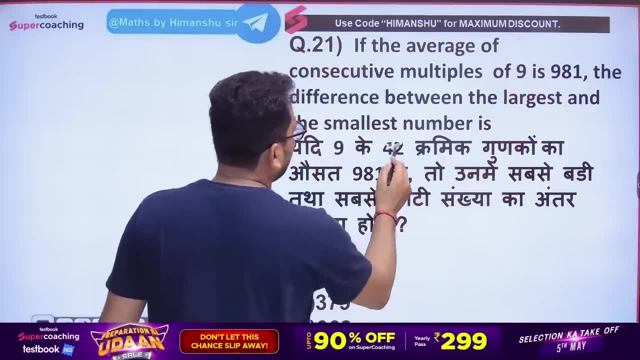 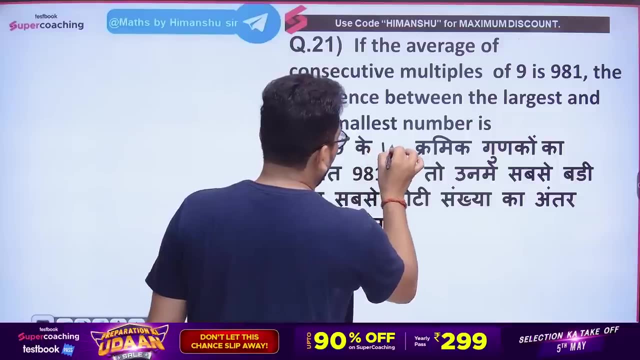 I am telling you, son, if the average of 42 is not here This time, it is not 42.. Okay, understand very carefully, It is not 42.. This time I am saying 101.. What is 101? 101.. 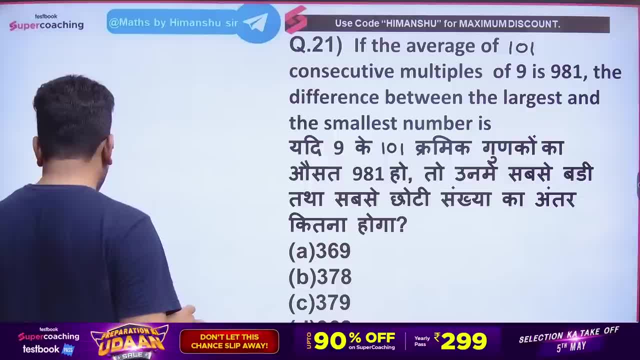 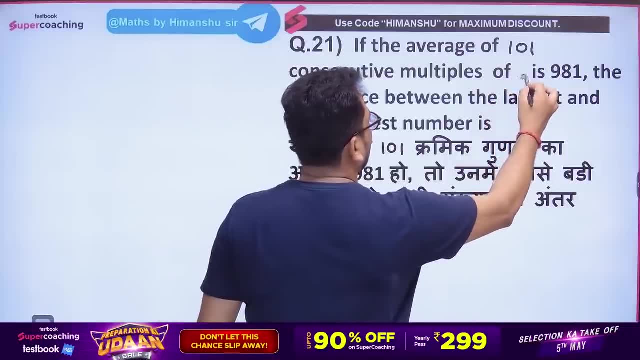 It is 101.. And there is not 9 here. Okay, There is not 9 here. He has given you here How much 10.. How much has he given you, son? He has given you 10.. Okay. 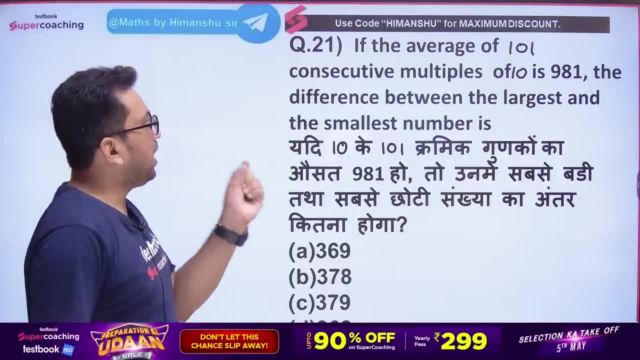 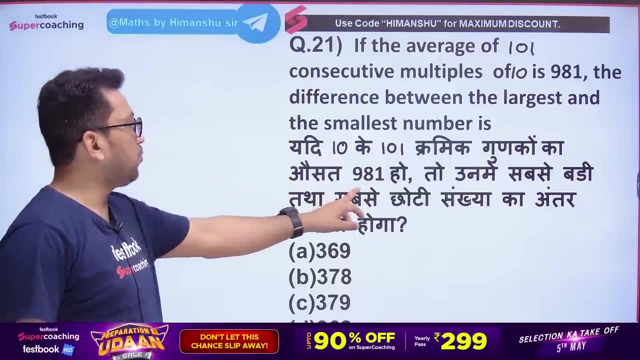 Come on, So you have to tell what will come. Okay, If the average of 101 consecutive multiples of 10 is. He has given it in this way And he is telling you that you have to tell the difference between the biggest and the smallest. 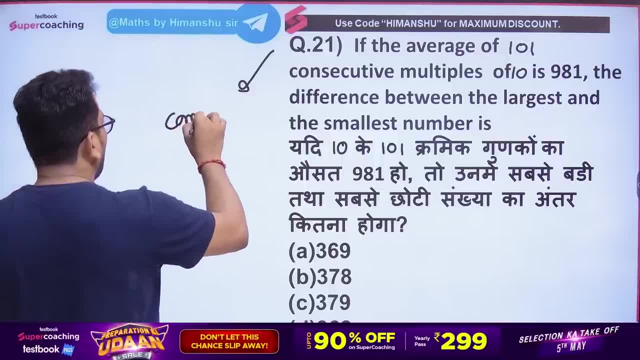 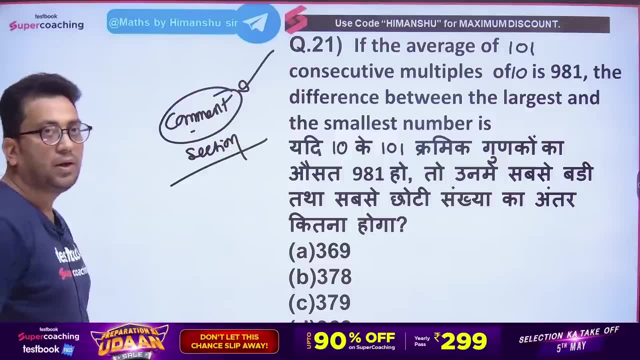 So you have to answer this question in the comment section. And son, look all the children who are watching the session here. I want every child to answer this question in the comment section, Okay, Okay. So now I will give you one more special information. 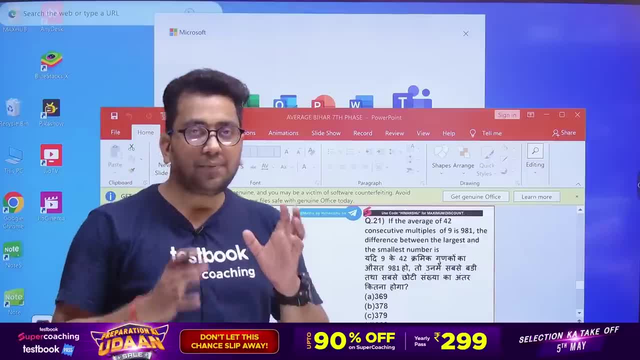 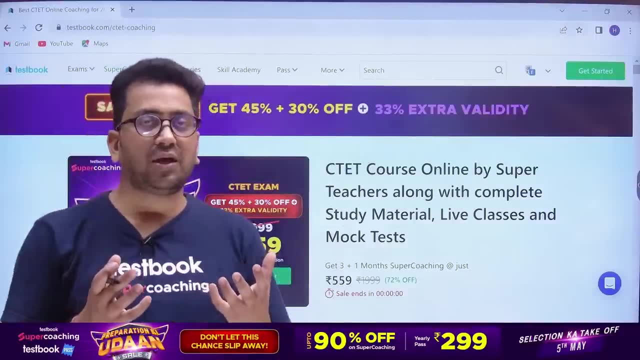 Look, son, On Super Coaching. the batch for Bihar, Shikshak Bharti, 7th Phase, has arrived. for all of you, The meaning of bringing this batch was only that that all the children of us are preparing for it. There is very little time for it. 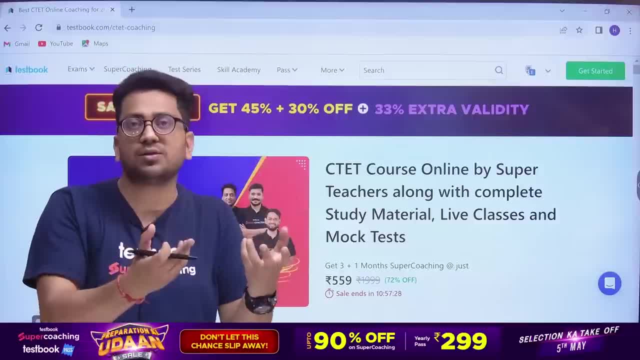 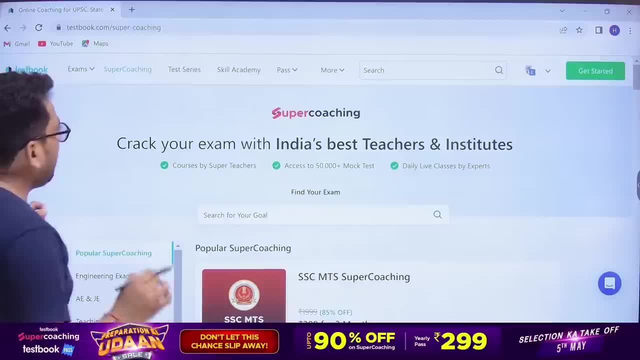 So this is the absence of time: How to complete the time, How to utilize it. So for that, I have made a batch available for you, And this exam date is going to happen. Okay, As soon as, son. what do you have to do first? 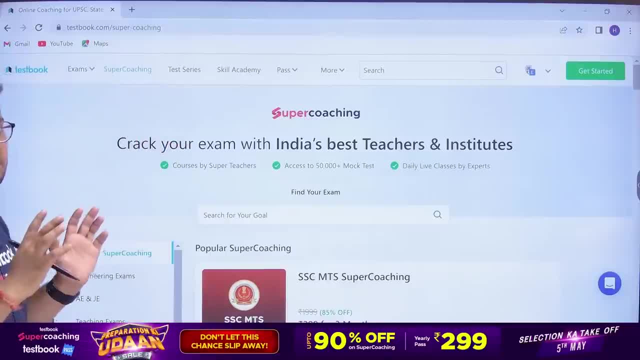 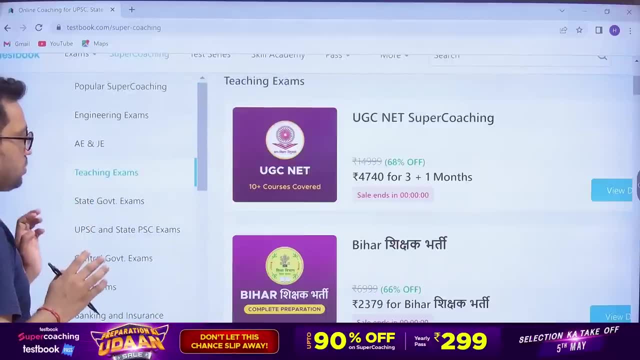 Let me tell you how you have to enroll. Then, what is the specialty of this batch? We will tell you about it. You have to go to Super Coaching. After going to Super Coaching, you will choose the teaching exam category. here You will see Bihar, Shikshak Bharti. on the second number.